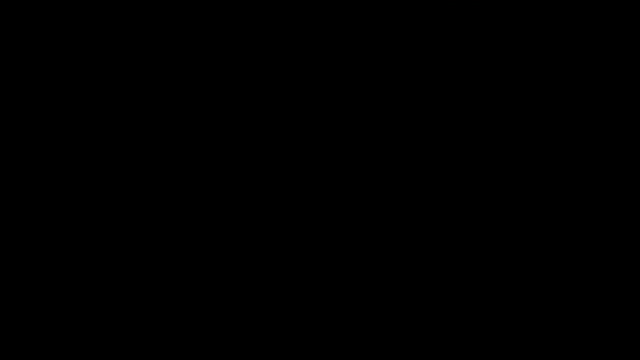 In summary, de Broglie proposed that for a matter particle with mass m moving at velocity v, you can associate a plane wave of wavelength lambda equals h over p, which is equal to h over mv. where p equals mv, This is the momentum of the particle and h is Planck's constant. Furthermore, 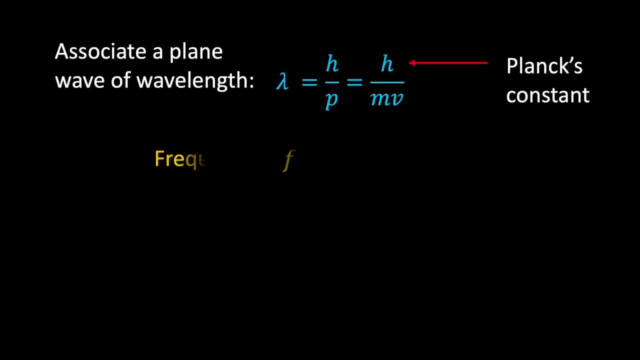 if the particle has energy e, then you can assign a frequency f equals e over h. These relations connect the particle concepts of energy and momentum, e and p, with the wave concepts of frequency and wavelength f, and lambda De Broglie took the bold. 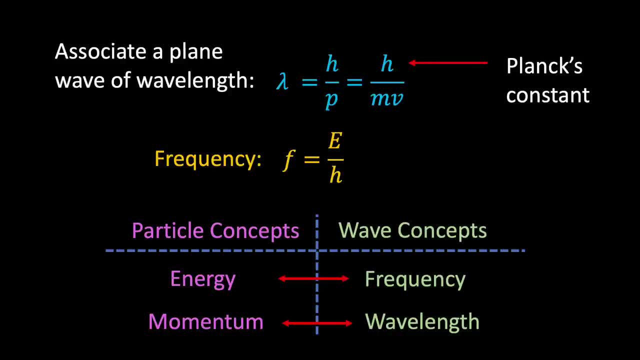 step of assuming that these two relationships hold for all matter, particles, including electrons, and it was this suggestion that ultimately spurred on Schrödinger to develop his wave equation, which I've covered in a different video titled What is the Schrödinger equation. But in this video I want to take 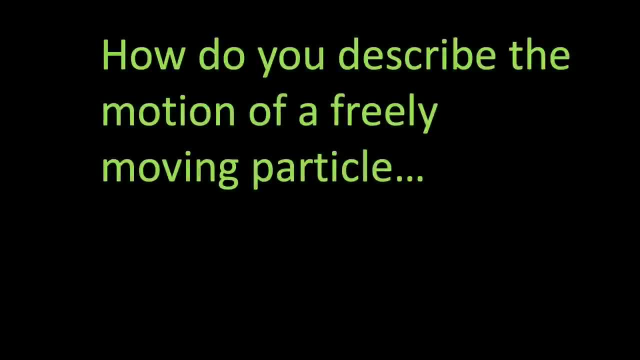 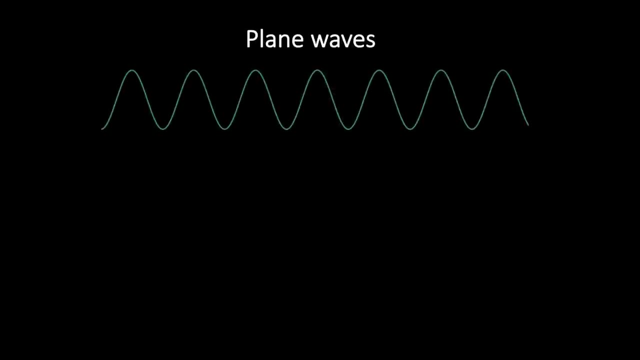 a different direction. So let me now refine the question I posed a moment ago. How do you describe the motion of a freely moving particle if it is to be described by a wave? If you're interested in the answer, stay tuned. Given that the de Broglie-Einstein postulates allow us to assign both a wavelength and frequency, 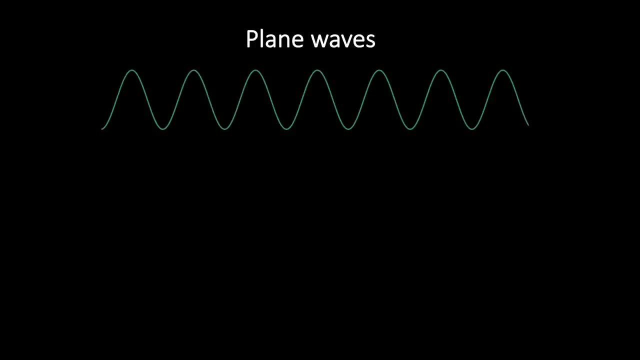 to our quantum particle. our first guess might be to describe our quantum particle using a plain wave wavefunction of the following form, where the symbol psi is used to represent the wavefunction. k equals 2 pi over lambda represents the wave number of the wave, which. 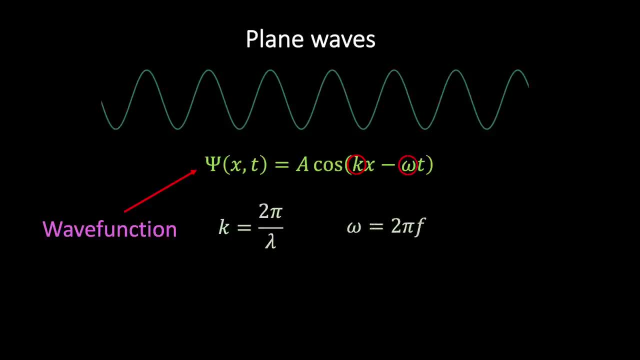 is simply the spatial frequency, and omega equals 2 pi. f is the angular frequency of our wave. The velocity of this travelling wave can be calculated by dividing the coefficient of t by the coefficient of x, and if we sub in the explicit expressions for omega and k. 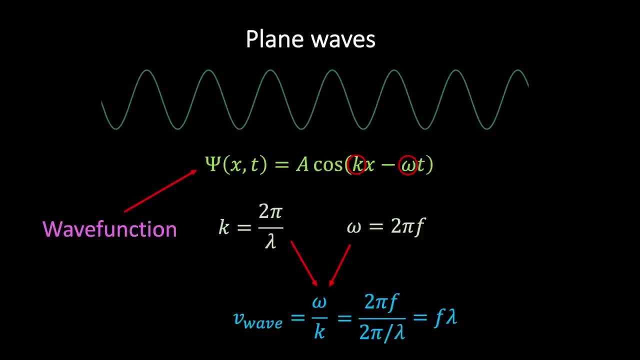 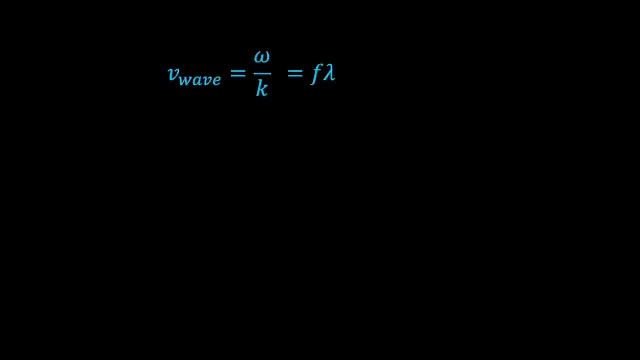 we recover the familiar relationship: v equals f lambda, which relates the wave speed, wave frequency and wavelength. Next, if we take the Einstein-De Broglie relations and rewrite them in terms of f and lambda, then we should be able to re-express the wave velocity in terms of the f lambda which is. 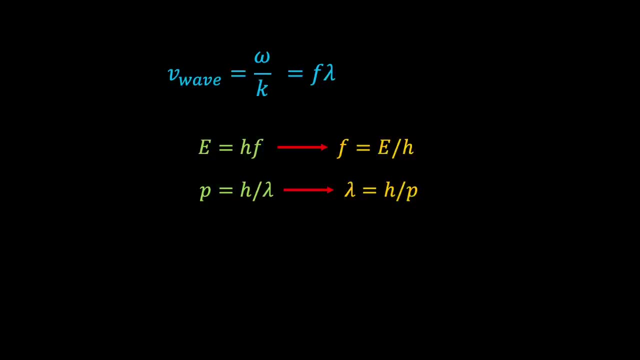 the energy and momentum of the associated particle. If we sub in the expressions for f and lambda, we find the following expression: and if we simplify, we find that the wave speed is equal to e over p. Now if we wish this travelling wave to somehow describe our freely moving particle, then 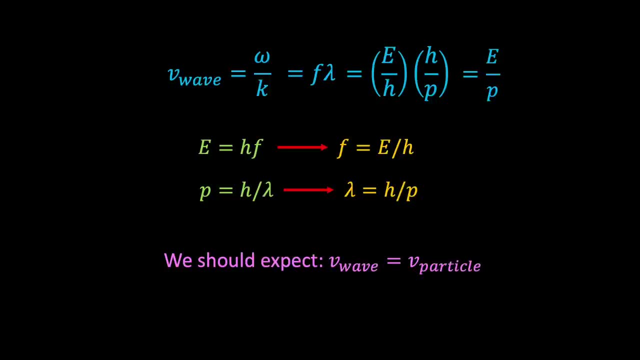 we would expect that the velocity of our wave is equal to the velocity of our particle. So is this the case? Yes, In a particle with mass m travelling at velocity v, subscript p, where p stands for particle. we know that the energy of the particle is given by. e equals half m vp squared and the 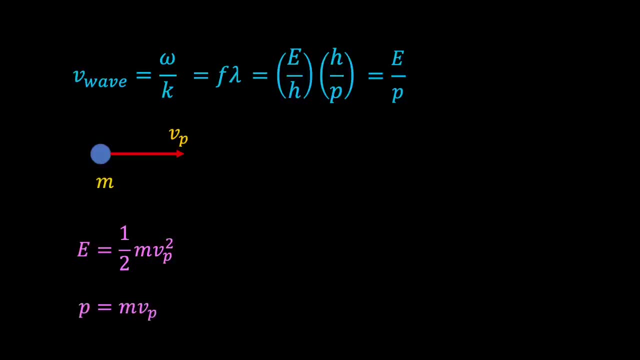 momentum of the particle is given by: p equals m, vp, And if we sub these expressions into the wave velocity equation and then simplify, we find the rather startling result that the velocity of the wave is equal to half the velocity of the particle. And so we see that we have a bit of a problem. 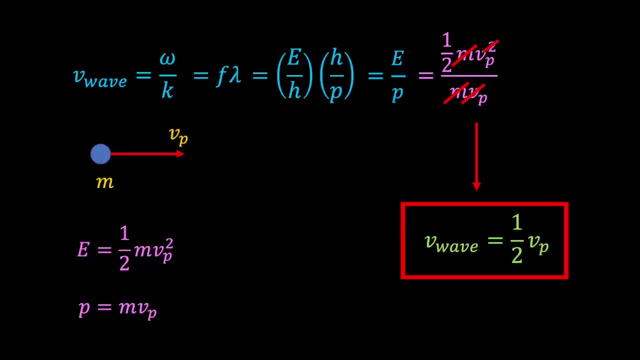 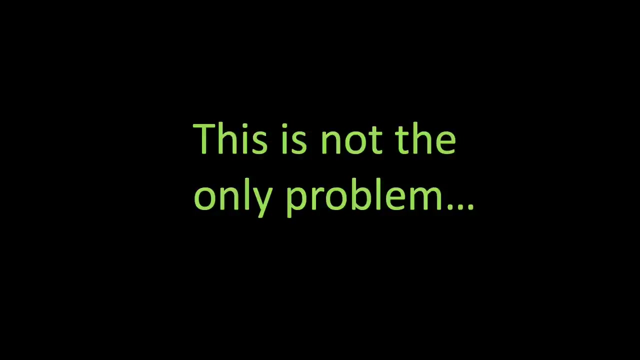 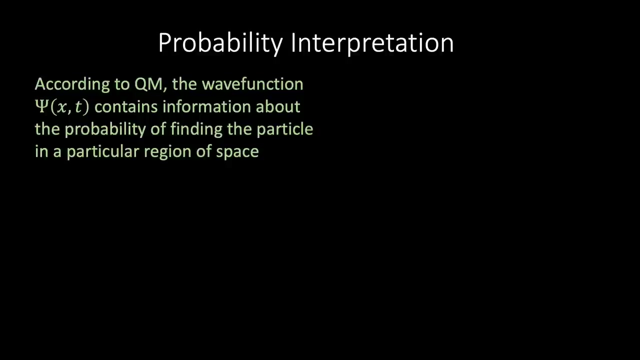 Apparently, the quantum mechanical wave function travels at half the speed of the particle that it's meant to represent. So what has gone wrong? Unfortunately, this is not the only problem associated with describing a particle with a plane travelling wave. According to quantum mechanics, the wave function psi of xt provides information about the 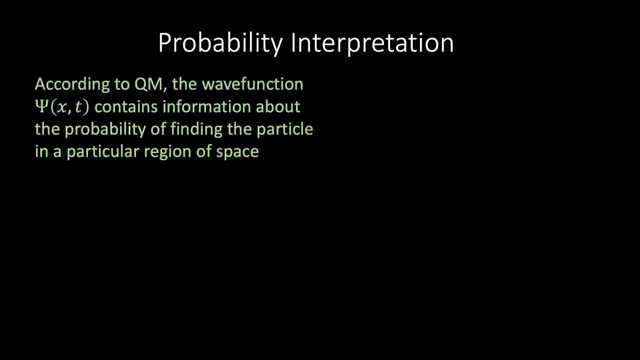 probability of finding a particle in a particular region of space. In other words, if at some instant in time, t, a measurement is made to locate the particle associated with the wave function, then the probability that the particle will be found at a coordinate between x and x plus dx, is equal to the modulus squared of the wave function. 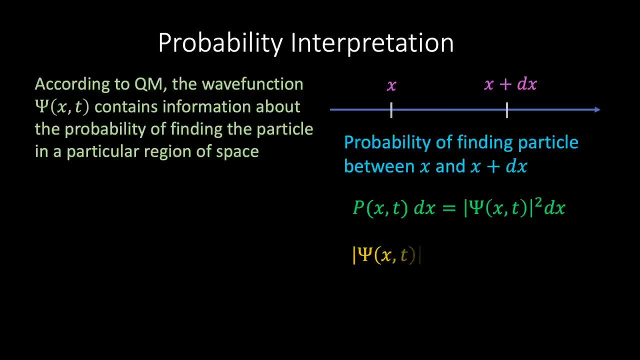 multiplied by dx, where, if you recall, the modulus squared is equal to the complex conjugate of the wave function multiplied by dx. If we then want to find the probability that the particle is located within a given region, we simply need to integrate the modulus squared. 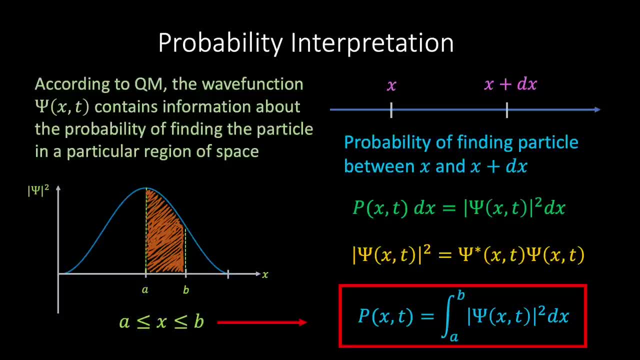 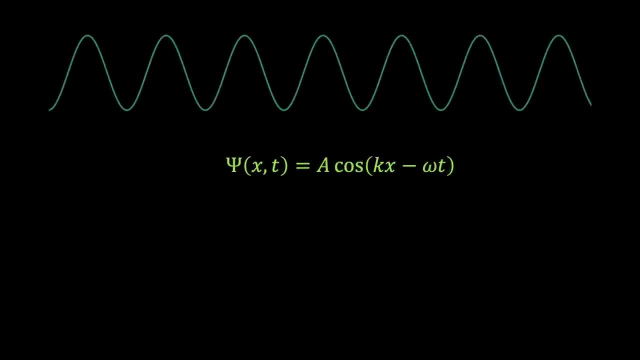 So, for example, the probability of finding a particle located in the region x is greater than or equal to a and less than or equal to b would be given by the integral from a to b of the modulus squared dx. So what does this imply for our proposed plane wave wave function? a, cos, kx minus omega. 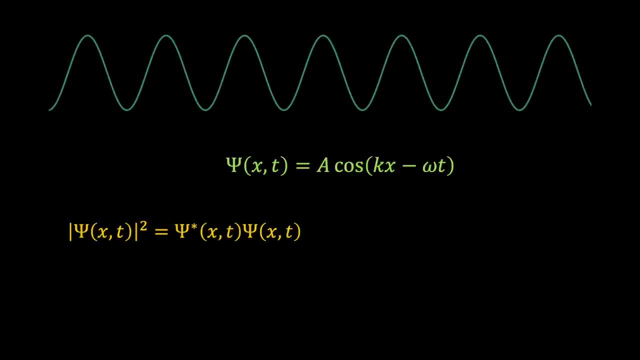 t. Well, if we take the modulus squared of this function, we find the answer of a squared cos, squared kx minus omega t. Now, assuming that our particle must exist somewhere in space, we would expect that the integral of this expression, evaluated from minus infinity to plus infinity, must be equal. 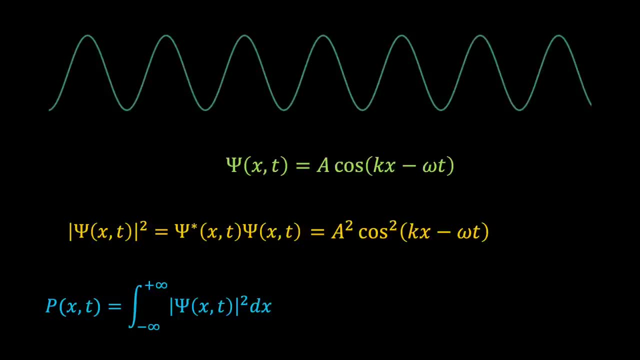 to one. However, if we perform the integral, we see that the integral must be equal to one. So, if we perform the integral, we see that the integral of this expression, evaluated from minus infinity to plus infinity, must be equal to one. 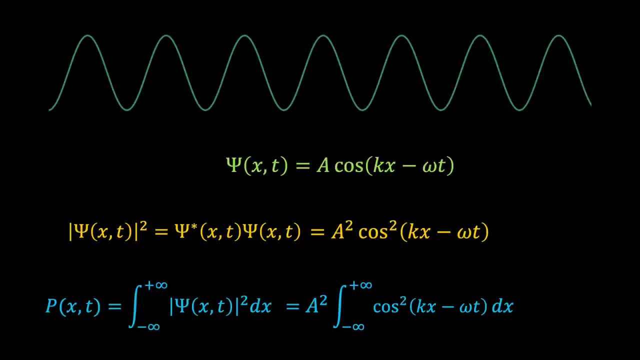 We see that we end up integrating cos squared kx minus omega t, from minus infinity to plus infinity, And since cos squared is always positive, the integral does not converge and we would get an infinite result. In other words, the plane wave wave function is non-normalisable. 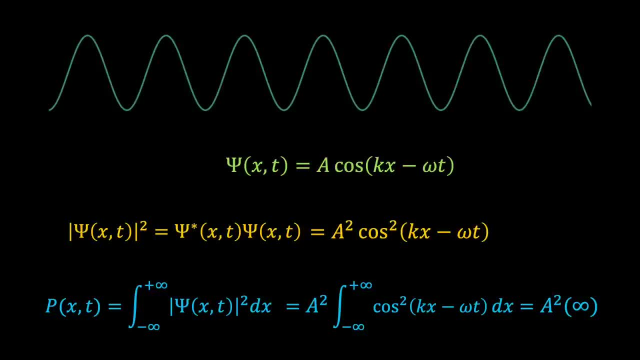 And so we see that in the case of a free particle, a plane wave wave function does not represent a physically realisable state. So in the case of a free particle, a plane wave wave function does not represent a physically realisable state. 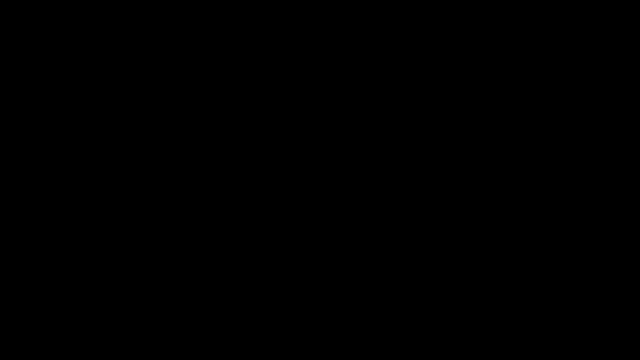 Something has gone wrong. So, to summarise, we've just seen that a plane wave wave function leads to an incorrect velocity and a non-normalisable wave function. So what is the cause of these problems? Well, the source of the problem is the plane wave wave function that we've been using. 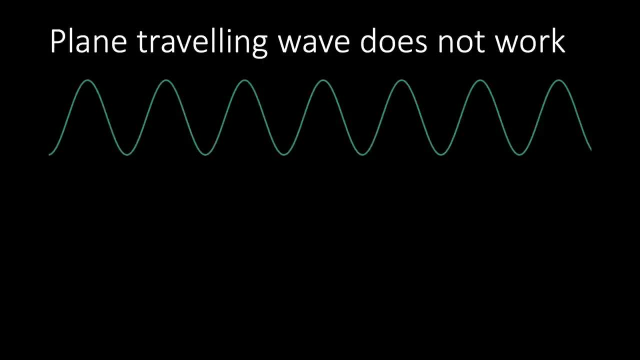 to describe our freely moving particle. Not only did this lead to a nonsensical probabilistic interpretation, it also led to the ludicrous result that the wave must be travelling at half the speed of the particle it's meant to represent. Now, since a particle is, by definition, an object that is localised in space, it is perhaps 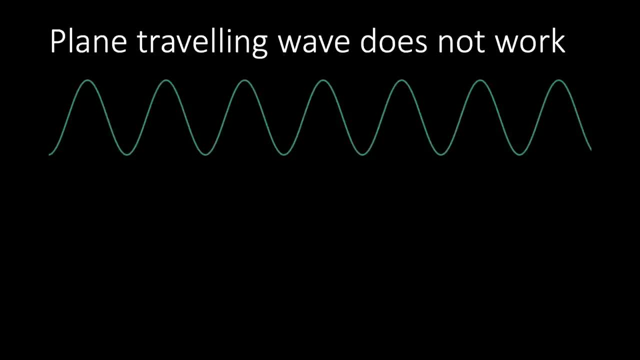 not surprising that our spatially extended plane wave has failed to do the job, Since the wave function tells us information about where we are most likely to find our particle. perhaps the solution to our problem is to construct a wave function that is localised in space. 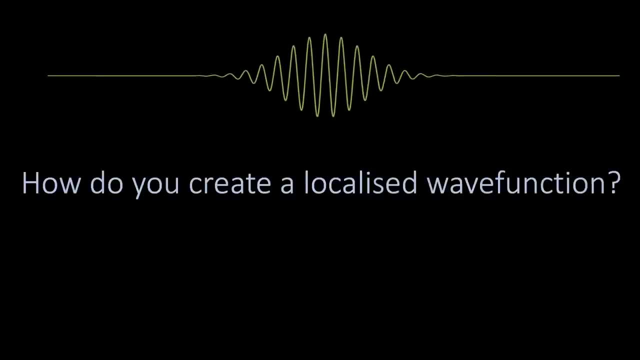 So how exactly do you create a localised wave function? Well, the answer turns out to be incredibly interesting: To create a single, isolated wave packet, we need to add together multiple waves with slightly different wavelengths, using the principle of superposition. To show how the principle of superposition works, consider adding together two wave functions. 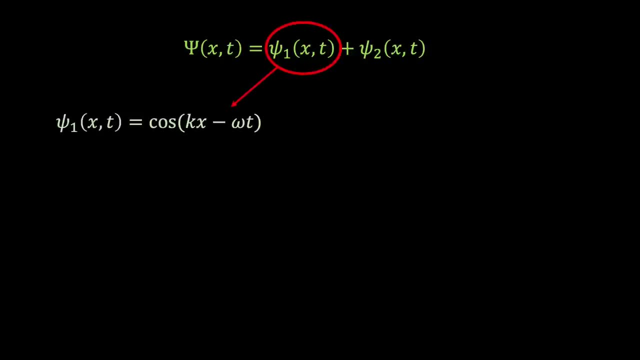 psi 1 and psi 2.. Where psi 1 equals cos kx minus omega t and psi 2 equals cos k plus delta kx minus omega plus delta omega t. In other words, the wave number of the second wave function is shifted by a small amount. 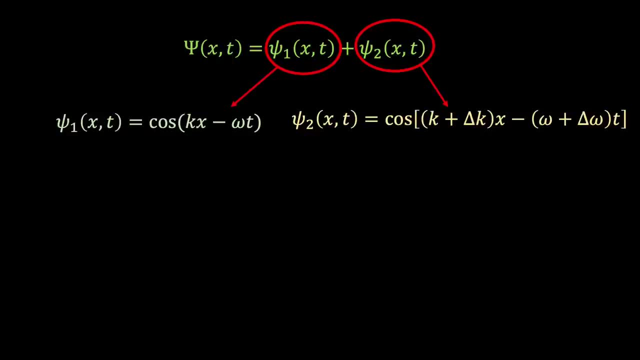 delta k relative to the first wave function, and the angular frequency is shifted by a small amount delta omega. Next, we can combine psi 1 and psi 2 by making use of the following trigonometric identity: Applying this to our two wave functions, we find the following yellow expression: 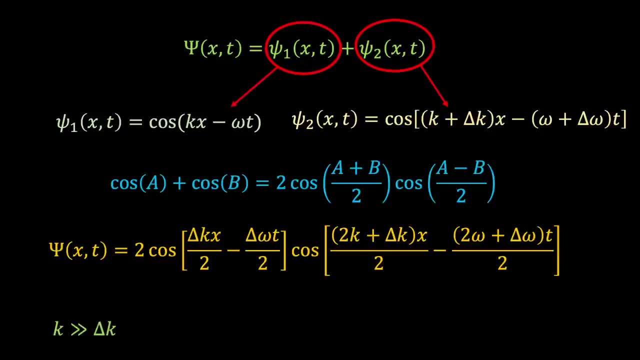 Next, if we assume that delta k and delta omega are very small compared with k and omega, then we can write that 2k plus delta k is roughly equal to 2k and 2 omega plus delta omega is roughly equal to 2 omega. 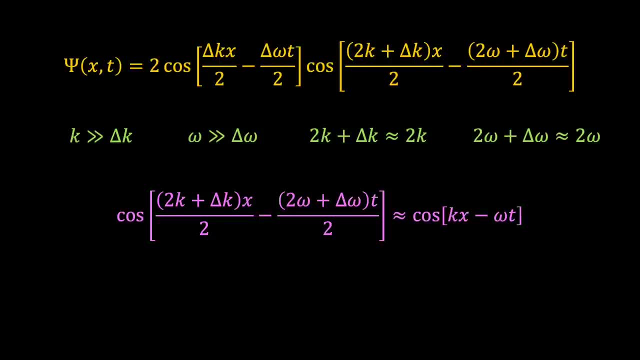 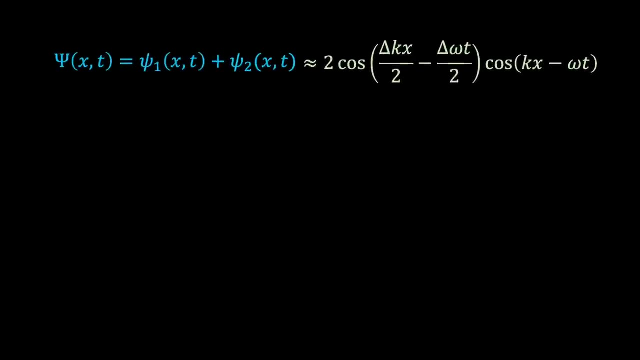 If we then sub this back into our expression, we see that the second cosine term that we're using dramatically simplifies and, as a result, our combined wave function expression takes the following simple form: So what does this combined wave function look like? 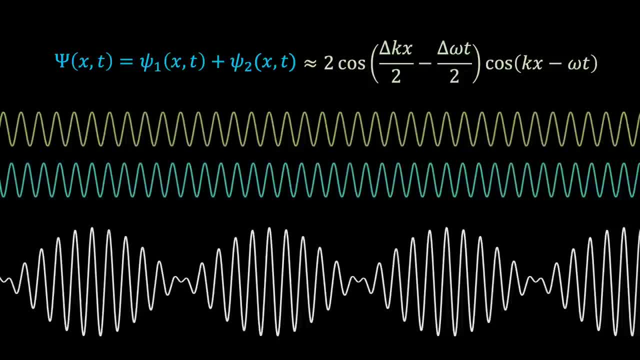 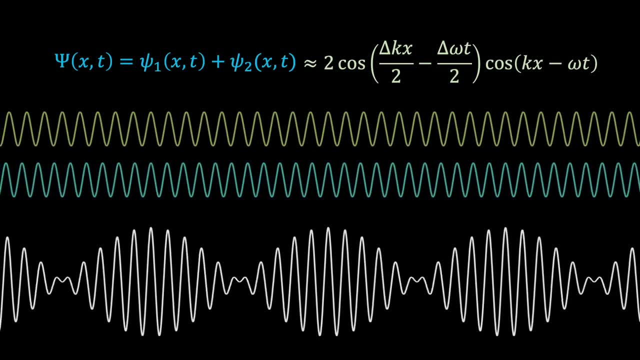 If we plot the two separate wave functions and then the combined wave function underneath, we find the following result: We see that the effect of combining the two wave functions is to produce a series of wave packets that move at a different velocity to the other side of the wave function. 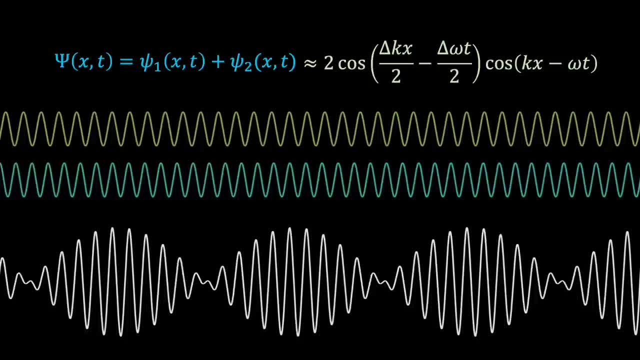 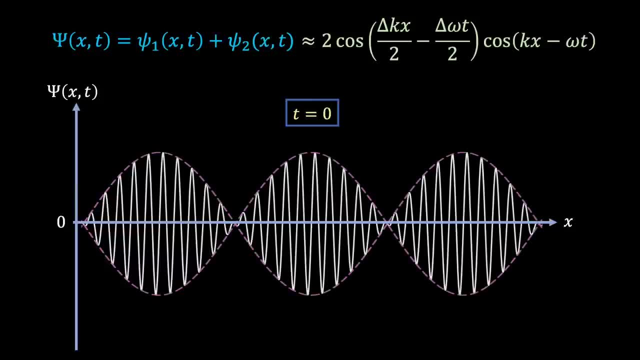 So what does this mean? It means that the two wave functions have the same velocity to the individual waves comprising them. Let's take a closer look and plot this function. at a fixed time, t equals 0.. We notice from the combined wave function expression that there are two cosine terms. 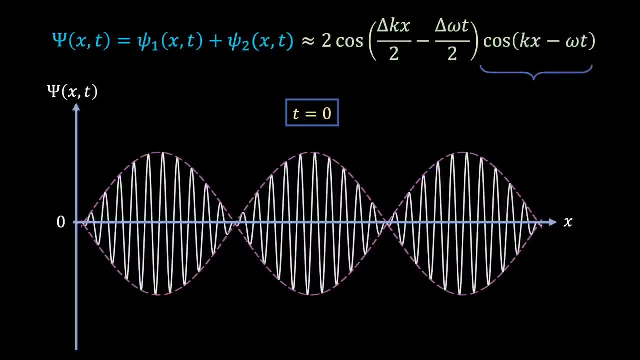 multiplying each other. The second cosine term, cos kx minus omega t, is exactly the same plane wave expression that we had earlier. However, the presence of the first cosine term modulates the amplitude And, as a result, the oscillations fall within a periodic envelope defined by the first. 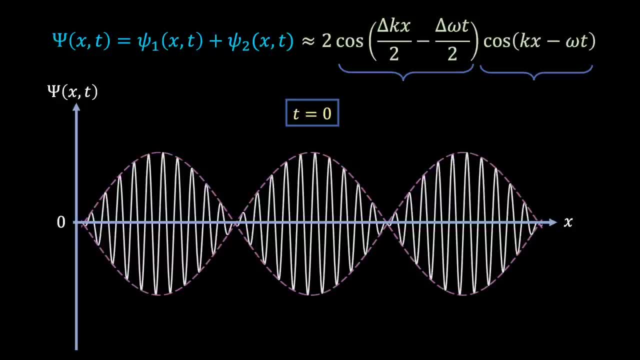 term. This is due to the fact that the two component wave functions have slightly different values of k and omega and therefore alternately interfere and reinforce in such a way as to produce a succession of groups. These groups and the individual waves they contain are both moving in the same direction. 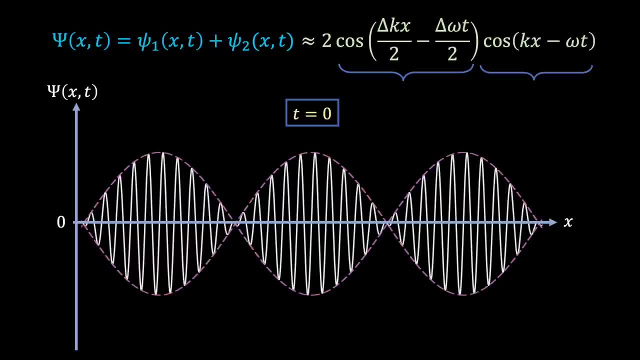 of increasing x. Furthermore, we notice that the velocity of the two wave functions is the same as the velocity of the two wave functions. This means that the velocity of the individual waves is different to the velocity of the whole group. So our next task is to investigate this difference. 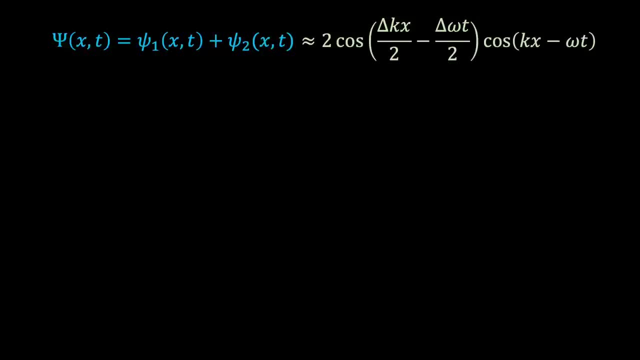 The velocity of the individual waves can be evaluated by considering the second cosine term. As we've already seen, the velocity of these waves can be calculated by dividing the coefficient of the t term by the coefficient of the x term, in which case we have that the velocity. 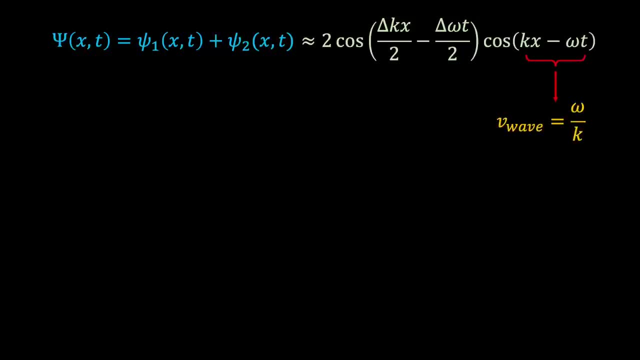 of the wave is equal to omega over k. To find the velocity of the group, we look at the first cosine term and again divide the t coefficient by the x coefficient, in which case we get the following result: Now, in the limit that delta omega and delta k go to zero, we can write the group velocity. 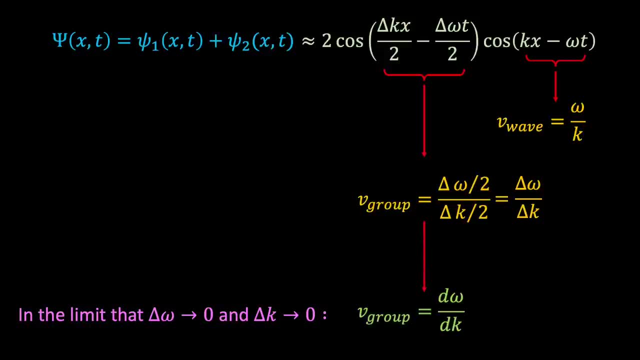 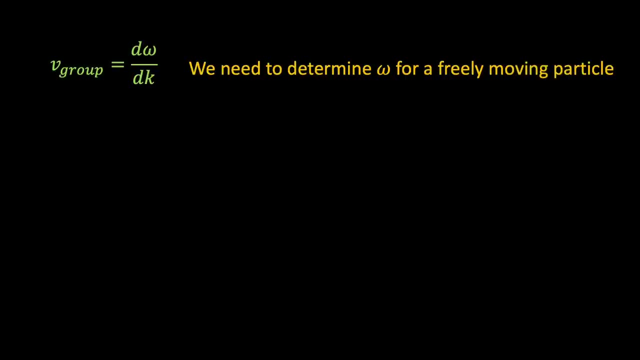 as the derivative of the angular frequency with respect to the wave number. So can we calculate this? Well, need to determine omega for a freely moving particle. To do this we can combine e equals hf with omega equals 2 pi f, and we see that omega equals e over h bar. Next, we know that for a 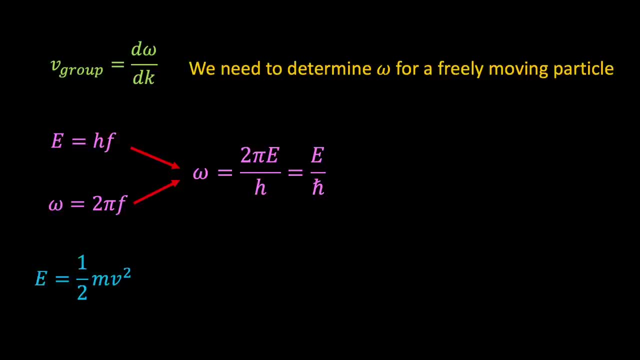 freely moving particle. e equals half mv squared and p equals mv, and therefore we can write the energy as e equals p squared over 2m. If we then substitute this into our expression for omega, we find that omega is equal to p squared over 2m h bar. Next, if we combine the de Broglie relation, 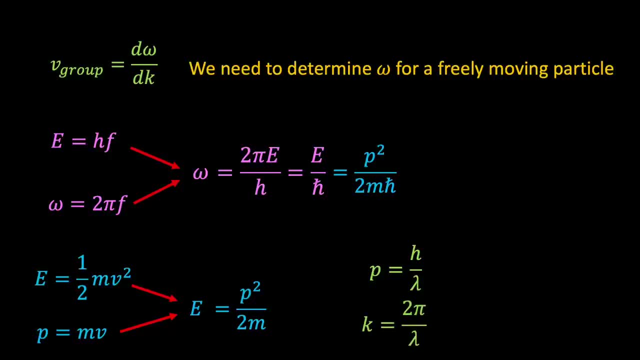 p equals h over lambda. with the wave number definition, k equals 2 pi over lambda. we see that the momentum can be written as: p equals h bar k and if we sub this into our omega equation, we find that omega is equal to h bar k squared over 2m. 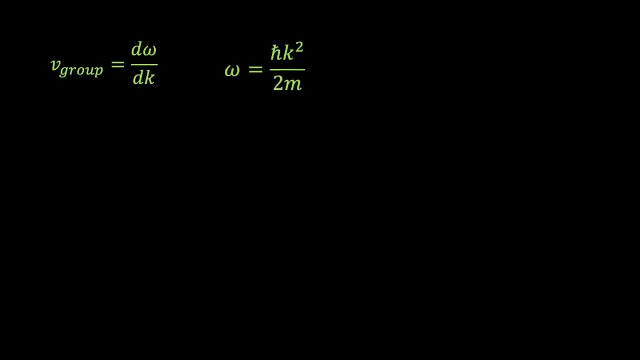 And so, now that we have an expression for omega in terms of k, we can substitute this into our group velocity equation, in which case we have the following expression: Next, if we perform the differentiation, then we find that the group velocity can be written as h bar k over m, and because h bar k is equal to p, 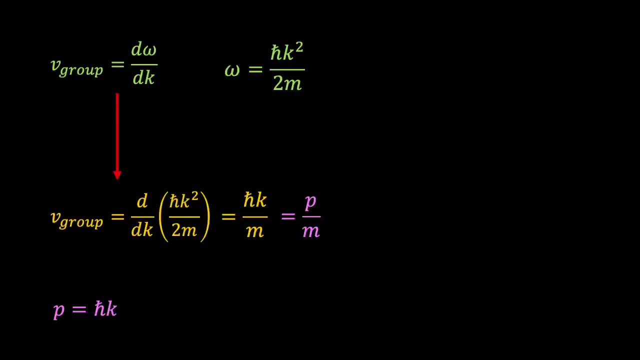 we see that the group velocity can be written as p over m. And finally, because for a freely moving particle the momentum p can be written as the mass of the particle multiplied by the velocity, it follows that the group velocity is equal to mvp over m, which simplifies to vp. 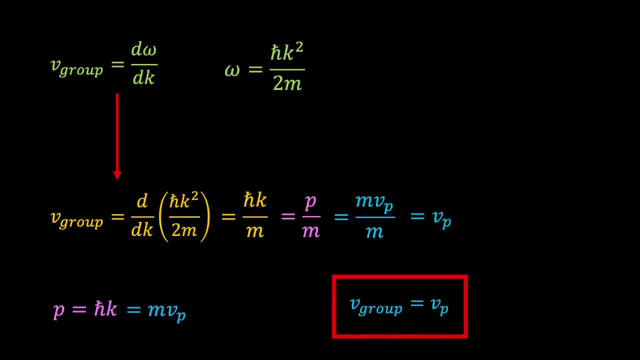 In other words, we have just shown that the group velocity of the wave packet is equal to the velocity of the particle that it's meant to represent. And so, to summarise, we see that when we form a group of waves using the principle of superposition, 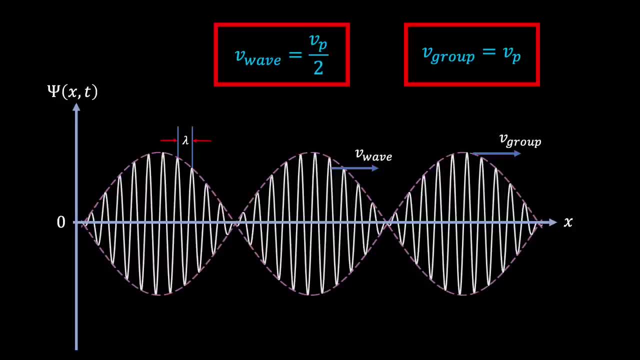 then, although the individual waves do not travel in the same direction with the velocity of our particle, the group itself does. We do, however, still have a problem. If the wave function describing our particle represents information about where the particle is likely to be located, then our previous analysis is: 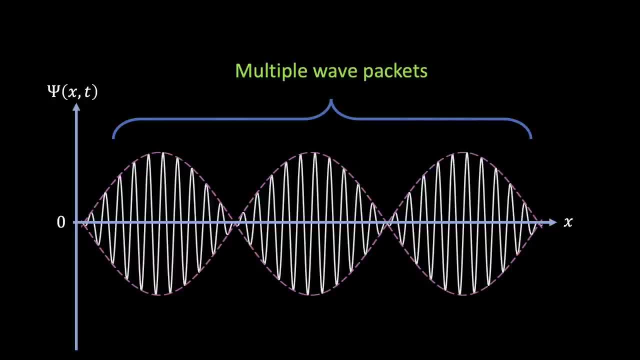 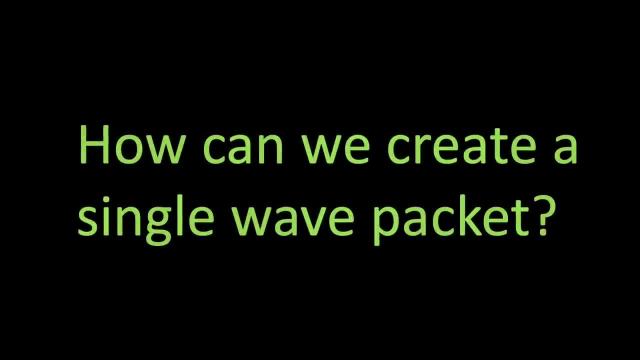 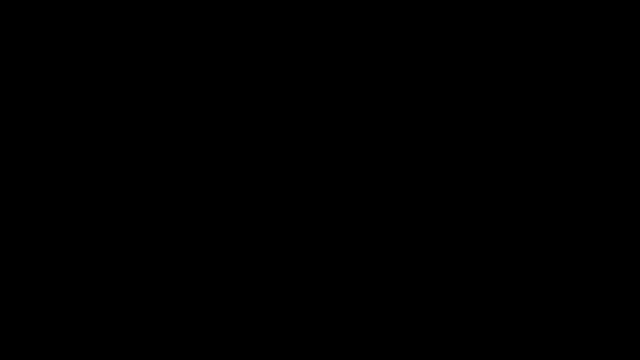 insufficient, as we have multiple wave packets rather than a single isolated wave packet. So how can we create a single wave packet? To answer this question, we will begin with a simple example. Let's consider the superposition of five waves each of the form a, cos, k, x. 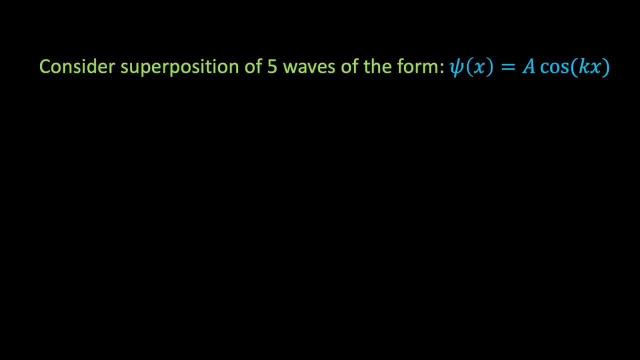 To simplify our analysis, we will set t equal to zero, which is why there is no time dependence inside the cosine expression. This simply means that we are considering a fixed moment in time. We will consider the more subtle question of time evolution at the end of the video. 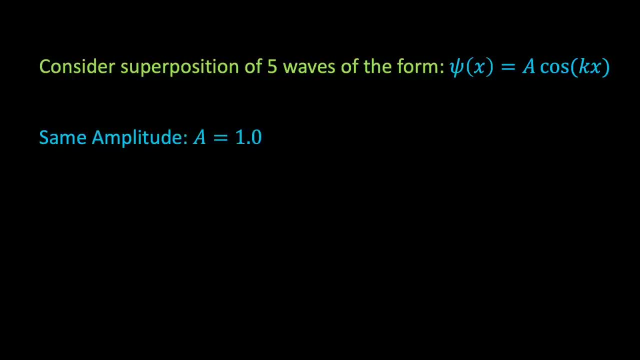 Next we will look at the problem of time. We will assume that all of our waves have the same amplitude, which we will take to be 1.0 in some arbitrary unit system, which is not important for the time being. We will also assume that the k values of each wave differ by pi radians per meter. 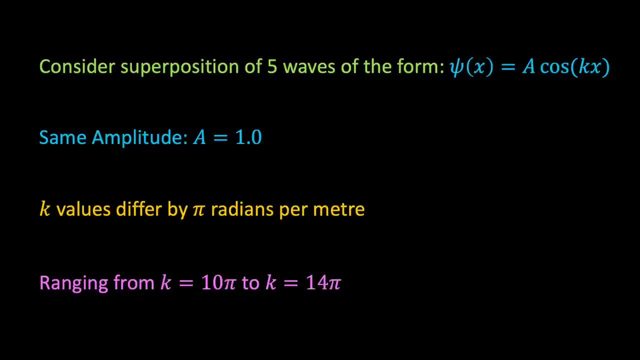 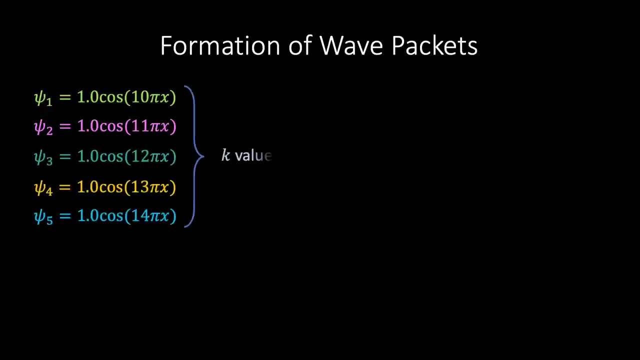 ranging from k equals 10 pi to k equals 14 pi. To make this explicit, let's write out the individual wave functions for each of the five waves. What we now want to do is form a superposition of five waves, each of the form a, cos, k, x. To make this explicit, let's write out the individual wave functions for each of the five waves. What we now want to do is form a superposition of five waves, each of the form a, cos, k, x. What we now want to do is form a superposition of five waves, each of the form a- cos, k, x. 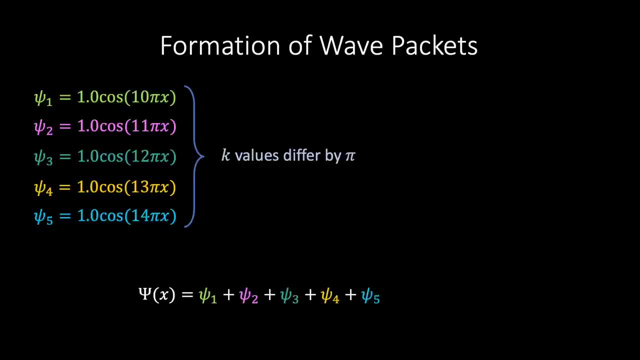 Which simply means we want to add together the individual wave functions. We can write this in a more compact form as: the sum from n equals 1 to 5 of a, n, cos, k, n, x, where the a? n's and k? n's take the following values: 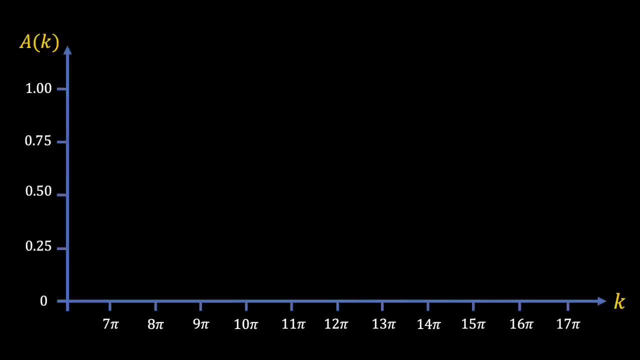 Now. it will prove useful for our analysis later to show how we can represent this superposition of waves graphically by plotting a graph with amplitude on the y-axis and wave number on the x-axis. For our example, we have five equal amplitude waves with wave 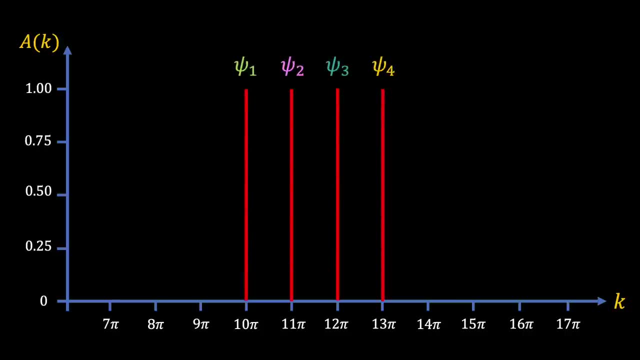 numbers of 10 pi, 11 pi, 12 pi, 13 pi and 14 pi respectively, corresponding to each wave function, And we see that this corresponds to five equal height lines on our amplitude versus wave number graph. This is often referred to as the k-space representation of the superposition. 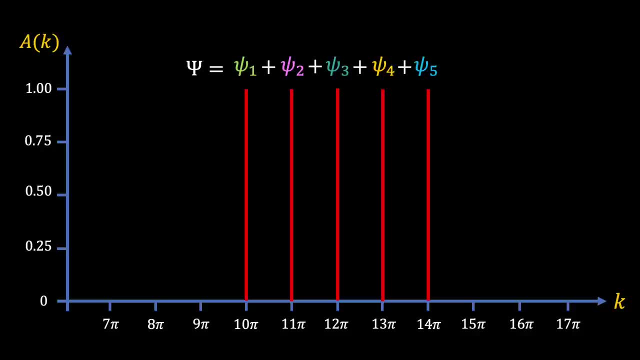 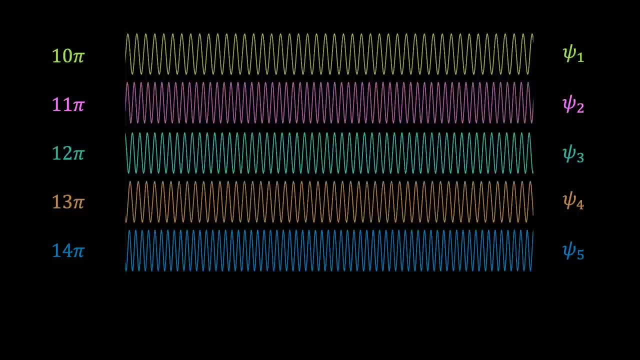 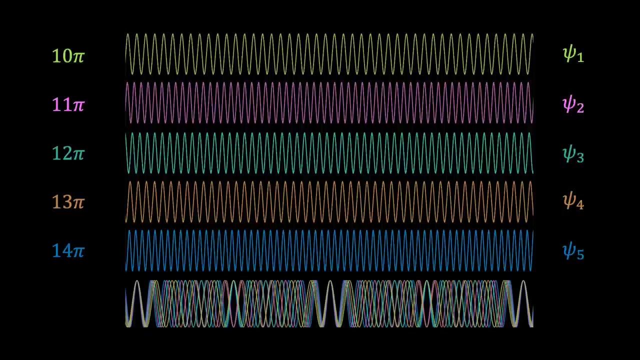 Since we are plotting the wave number k on the x-axis. So let's now see what happens when we add these five waves together. We notice that, due to the difference in k values between the five waves, when we superimpose the five waves on top of each other, there are regions where the waves 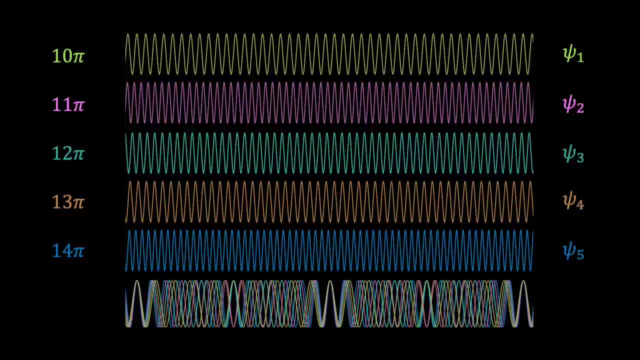 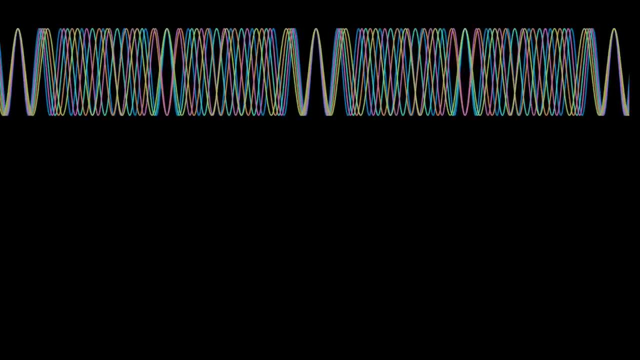 perfectly overlap and there are regions where the peaks of some of the waves coincide with the troughs of other waves. According to the principle of superposition, the waves will add together where the waves overlap perfectly and they will tend to cancel out where peaks and 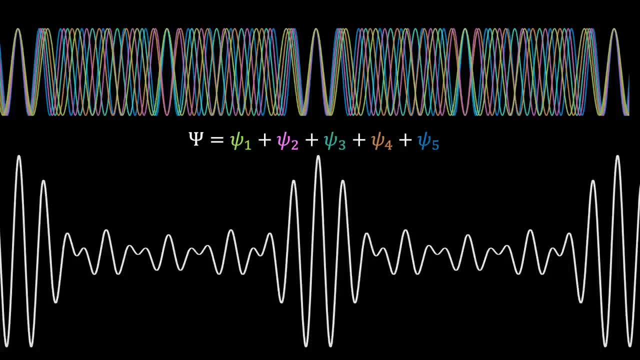 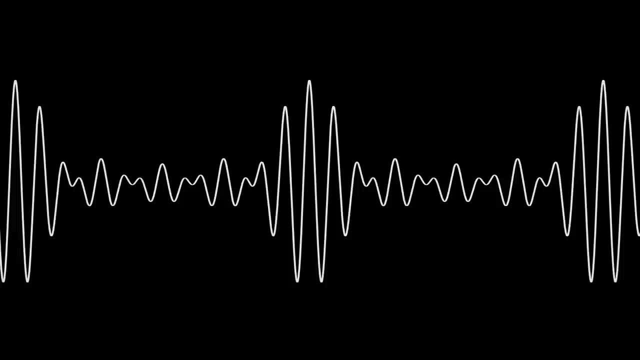 troughs coincide and the net result will be like the pattern shown. We see that the result of adding five waves with k values differing by pi radians per meter has been to create a series of spatially separated wave packets. We also notice that in between the wave packets there are smaller 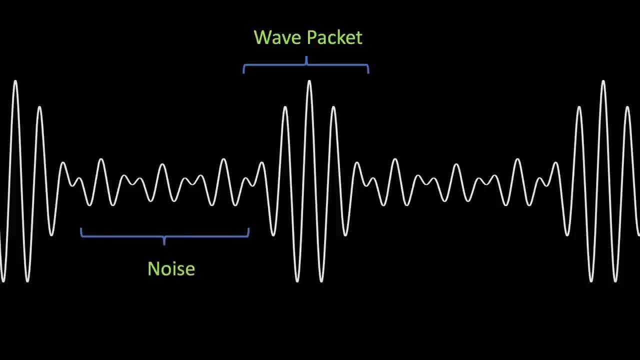 oscillations, And these occur because, when we added together the five waves, they did not perfectly cancel in these regions, And so we have two problems that require a solution. Firstly, how do we get rid of the smaller fluctuations in between the wave packets? 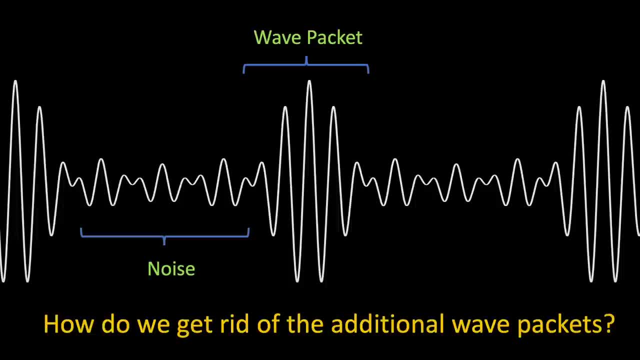 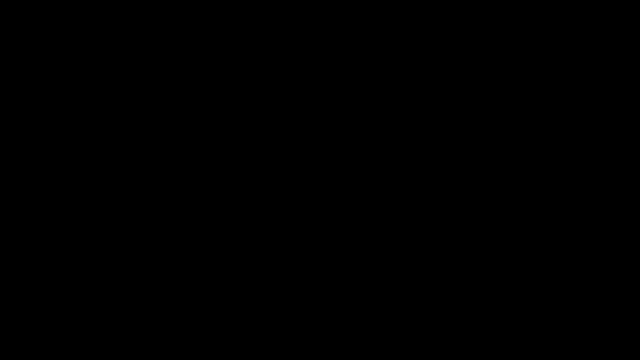 And secondly, how do we get rid of the additional wave packets? To answer these questions, we will have to develop our understanding of the superposition of waves. But to begin with, let's see what happens if we simply add more waves together and reduce the. 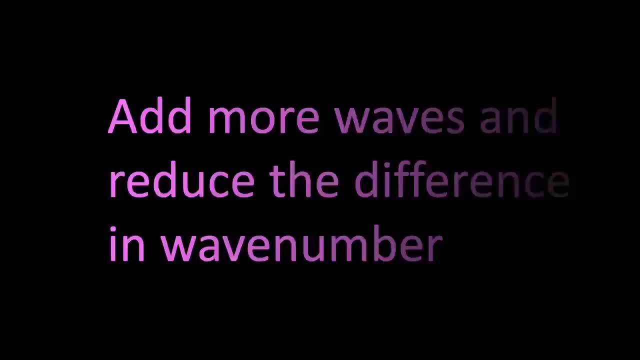 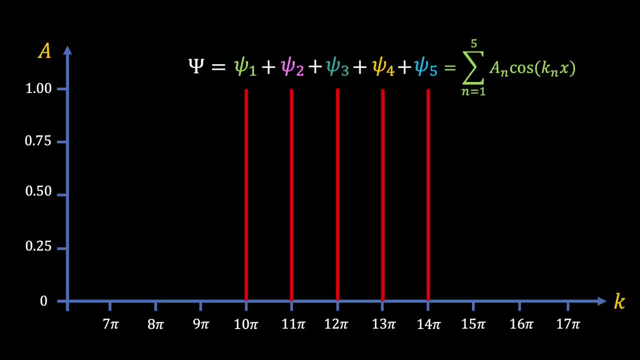 difference in waves between the waves. Previously we considered the superposition of five equal amplitude waves with k values that differed by pi radians per meter. Let's now add an additional four waves, such that the difference between each is pi over two radians per meter. You can see this represented in k-space on our graph. 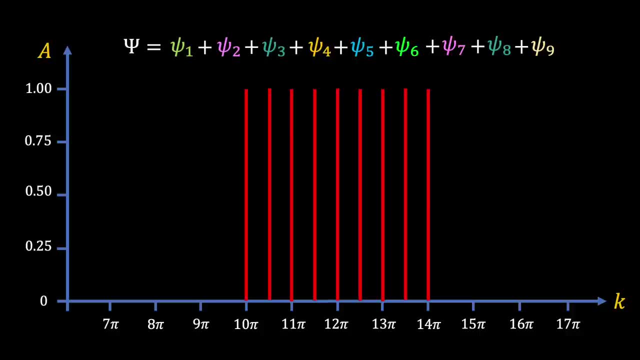 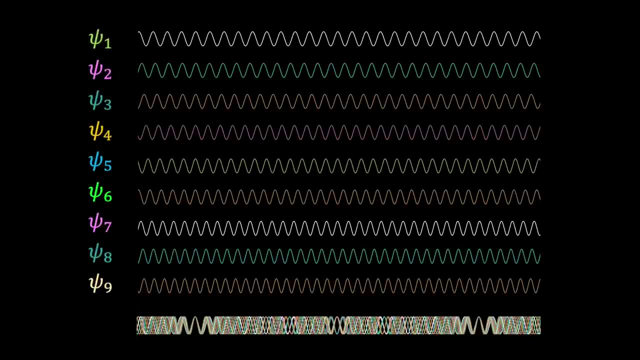 by the nine equal length vertical lines. And, as before, we can write this superposition of waves as the sum of a, n, cos, k and x, where now n runs from one to nine, If we line up each of these nine waves and then superimpose them on top of each other. 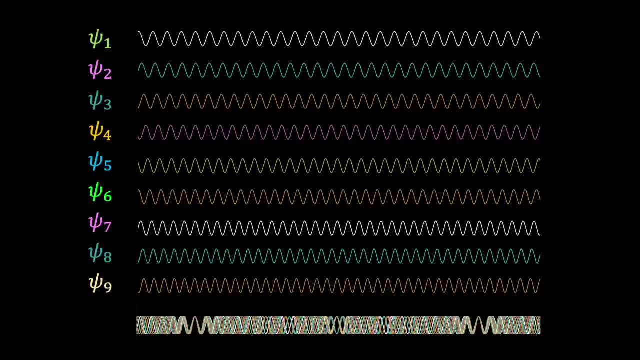 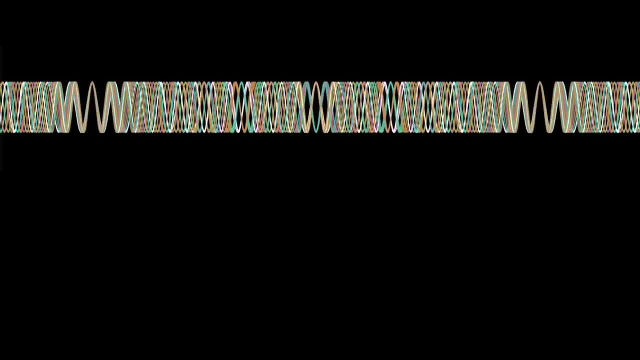 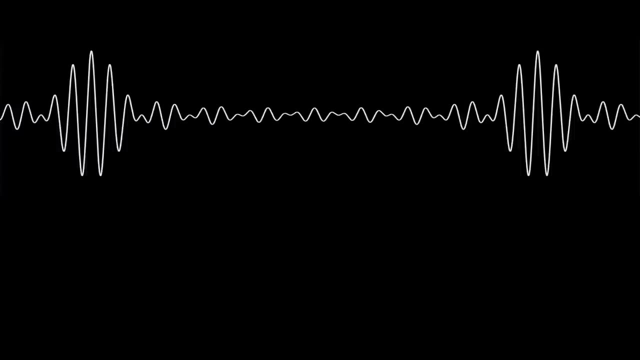 we again see that there are regions where the waves coincide and regions where they do not. If we then explicitly add these waves together and look at the net amplitude, we find the following pattern: If we then compare this with our previous five wave pattern, we see that the net effect of adding more waves within the same k range 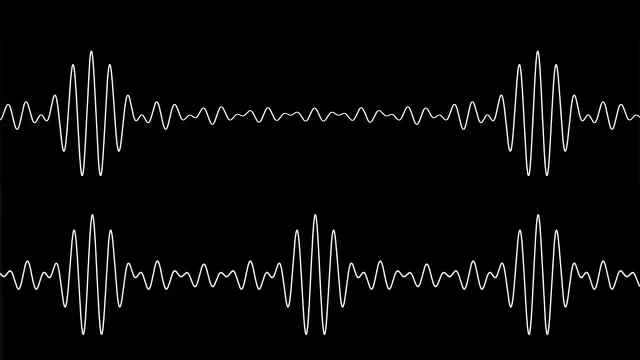 but with a smaller difference in k values, is that the wave packets are now more spread out, with a greater space between individual wave packets, So perhaps this is hinting at a strategy for producing a single isolated wave packet. We simply need to add more waves and reduce. 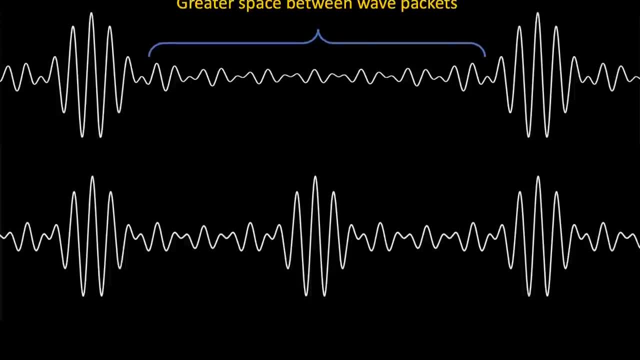 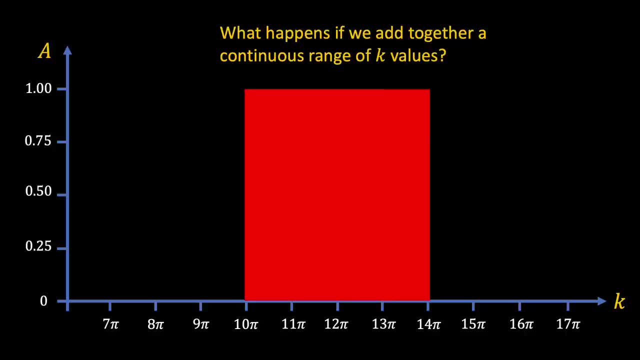 the difference in wave number between the waves. So a natural question arises: what happens if we add together a continuous spectrum of k values within the same range as before? Can we explicitly calculate what the net result of this superposition would be? Well, thankfully, the answer is yes, so let's do that. 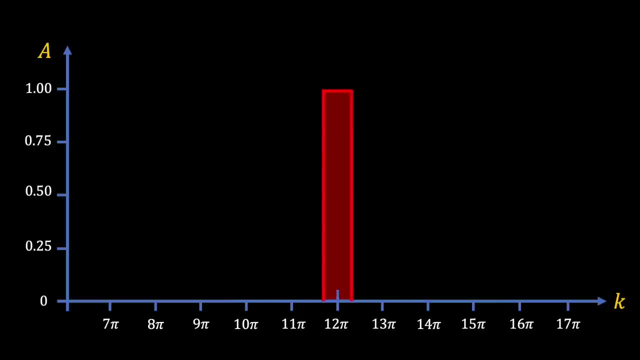 Let's consider a situation in which we have a small range of k values, labelled delta k, centred around a k value that we will label k naught. It then follows that the lowest k value will be equal to k naught minus delta k over 2,. 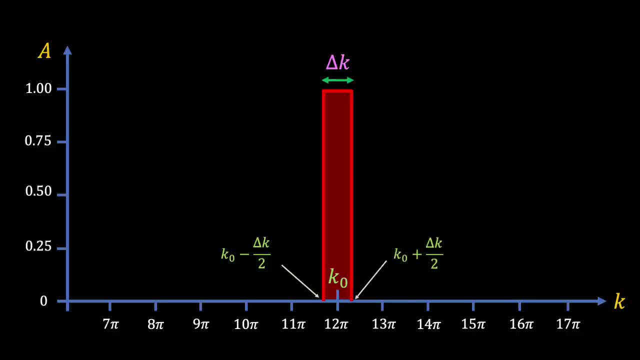 and the highest k value will be equal to k naught plus delta k over 2.. We will again assume that all of our waves have the same amplitude, and so we can specify the continuum of k values by stating the following condition: that a of k is equal to 1 in the given range and a of k is equal to 0 for all other k. Our task is to 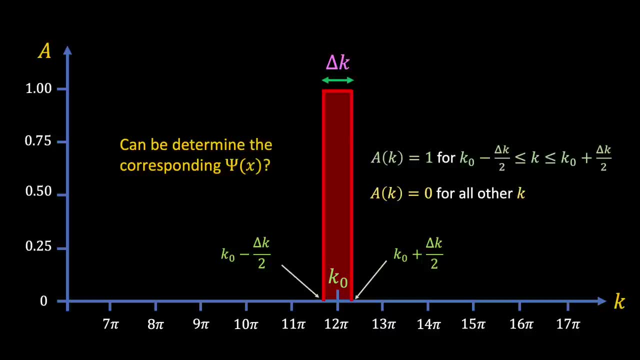 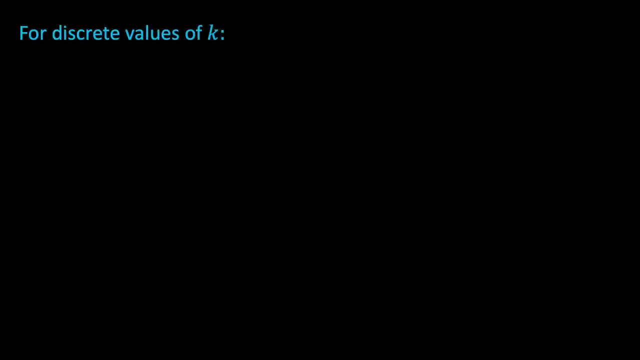 now find an expression of the net effect of adding more waves within the same range as before. So how do we do that? If you recall, when we were dealing with discrete values of k, we were able to calculate the superposition of our wave functions by simply adding together the separate functions. 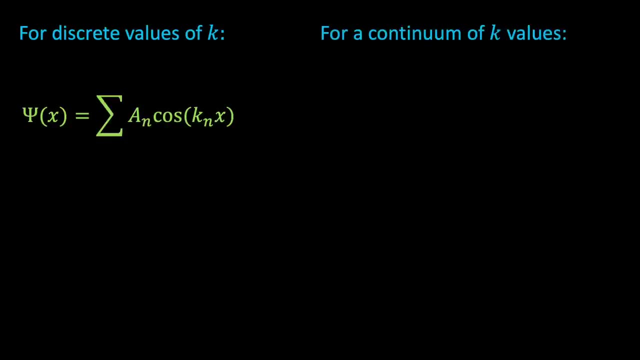 However, when dealing with a continuum of k values, we need to replace our discrete sum with a continuous integral of the following form: We recognise that this has the same general strength, and so we need to replace our discrete sum with a continuous integral of the following form: 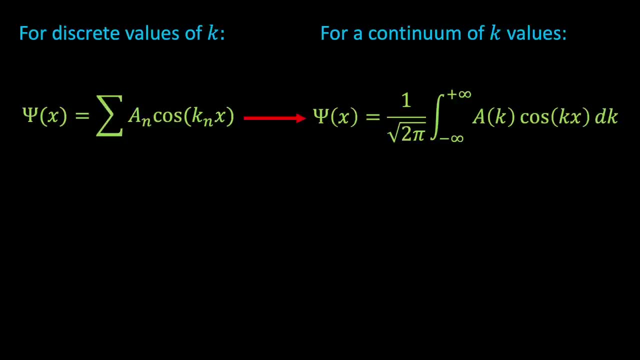 We recognise that this has the same general structure as before. only now our amplitude is a function of the wavenumber and we write this as a of k. Furthermore, instead of summing over n discrete k values, we integrate over all k values from. 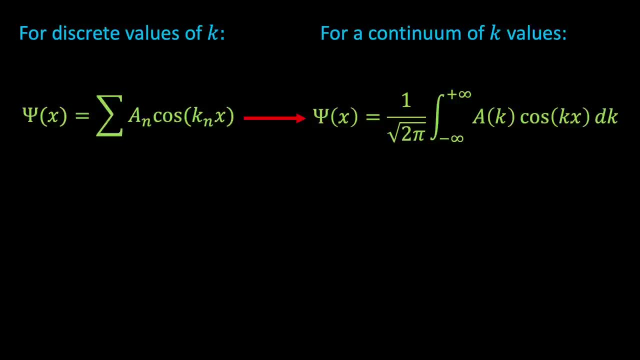 minus infinity to plus infinity. And finally, we include a standard 1 over the square root of 2, pi normalisation factor. This expression actually has a name. it is referred to as a Fourier transform and this general type of integral plays a key role in. 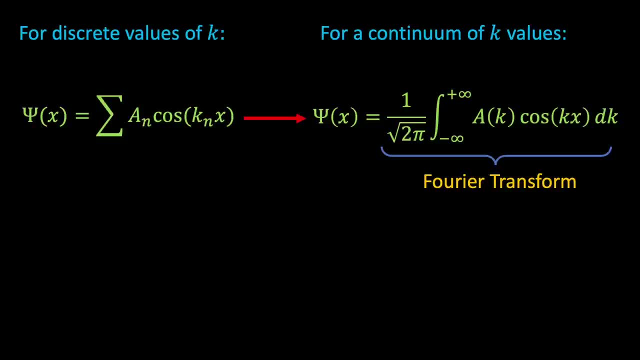 the mathematics of waves and vibrations. Our task is to now use this integral expression to calculate the resultant wave function corresponding to the amplitude function we have just specified. If we sub in a of k equals 1 and change the limits of our integral, we arrive: 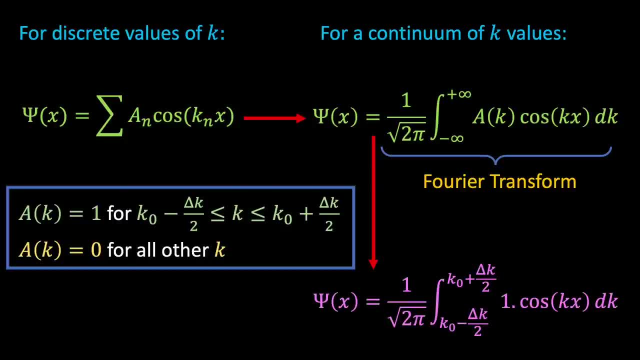 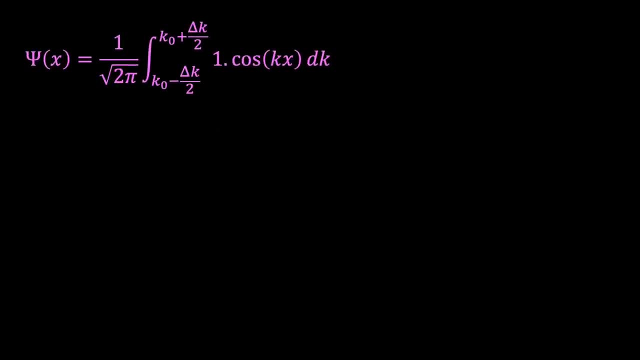 at the following expression: So our next task is to calculate this integral. Well, thankfully this is a relatively straightforward task. we are integrating cos with respect to k, and so when we perform the integral, we get sine of KX over X. If we then sub in the limits of our 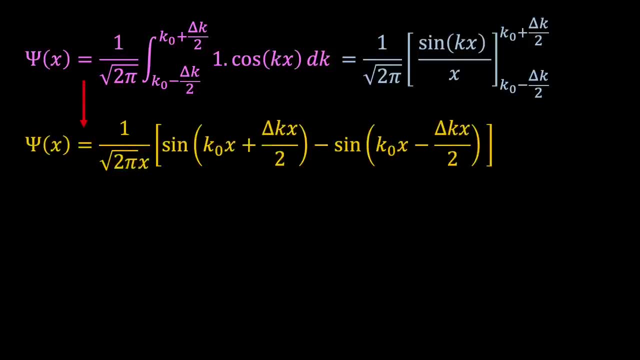 integral, we find the following yellow expression: We can simplify this by making use of the following well known formulas that are called X-ă cycles trigonometric identity. Applying this to our wave function, we find the following result: The final step is to multiply the top and bottom of this expression by. 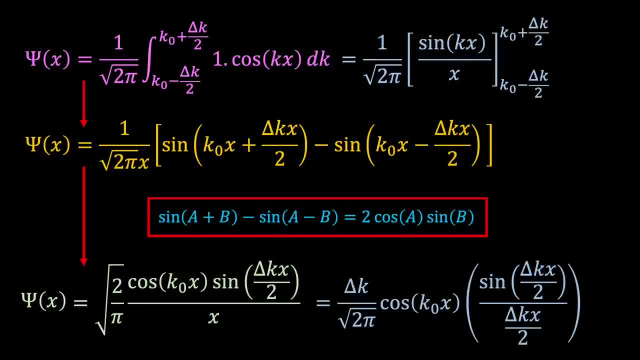 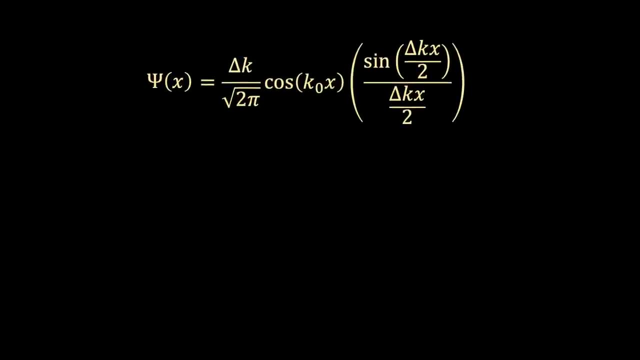 delta k over 2, in which case we find that the wave function can be written in the following equivalent form: So let's take a closer look at this function. We see that it comprises a cosine term multiplying a term in brackets, involving sine of delta k x over 2, divided by delta k x over 2.. If we 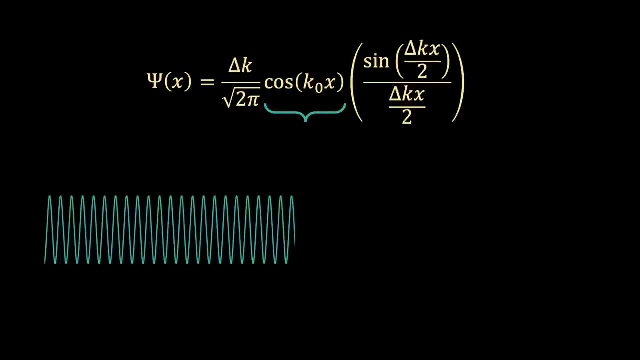 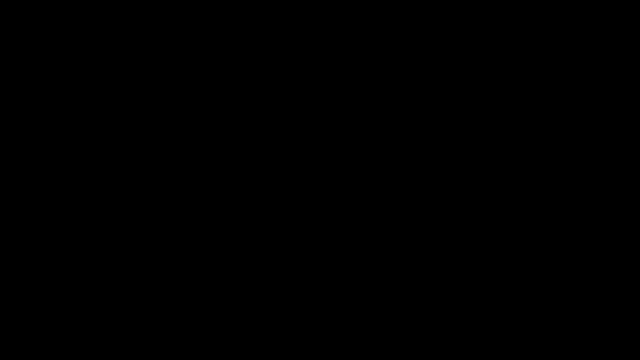 were to plot the first cosine term on its own, we would find something that looks like this, whereas if we were to plot the term inside the brackets, we would find something that looks like this: So what would the product of these two terms look like? To answer this question, let's plot a graph of our wave. 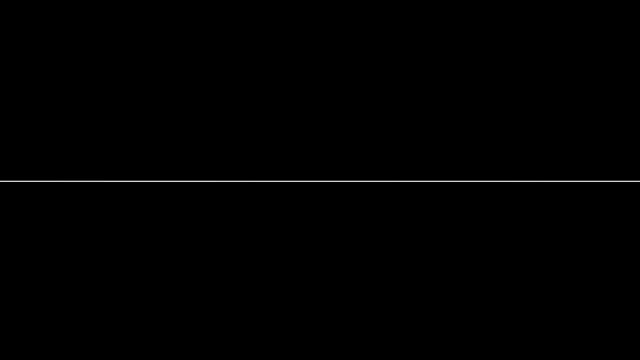 function with the x-axis representation, The y-axis representing the value of our wave function. If we then plot the wave function, we find the following pattern. We see that we have a large central wave packet lobe with a series of much smaller side lobes to the left and right. 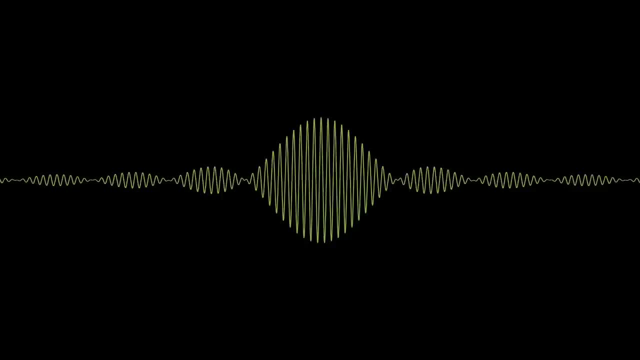 At first glance this does not look any better than our earlier attempts to create an isolated wave packet. However, if we zoom out a bit and then a little bit more, we see that the large central lobe and side lobes are indeed localized in space and as we move off in the positive or negative x. 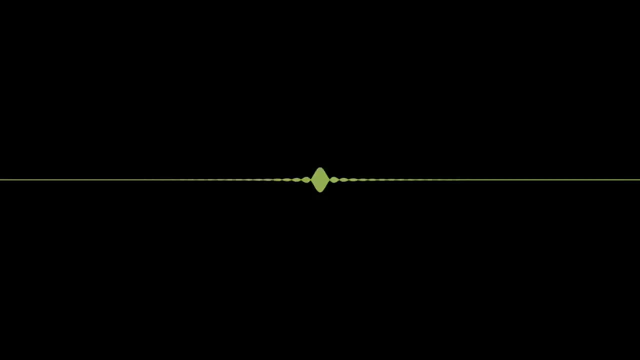 direction, the amplitude of the wave function reduces to zero, And since the wave function tells us information about where we are most likely to find our particle, we have at least partially succeeded in confining the particle to a smaller region of space than when we had a periodic series of wave packets. 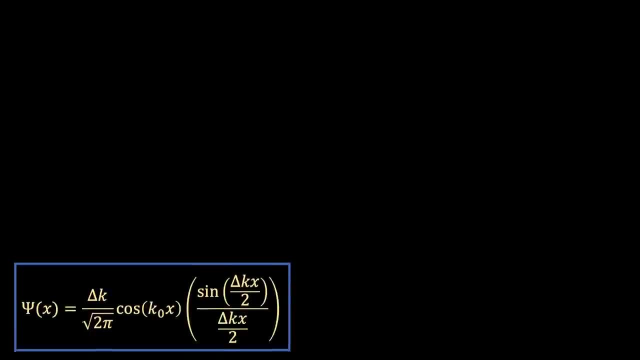 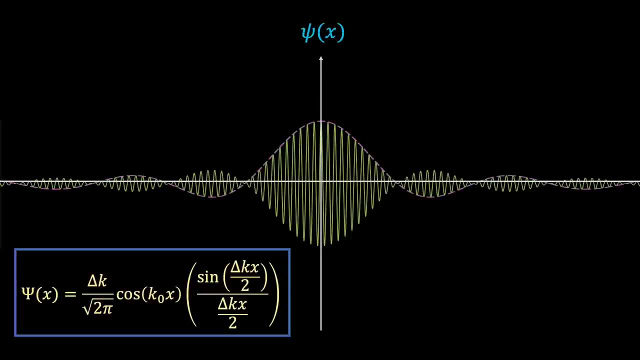 spreading throughout all of space. So let's pause a moment and take a closer look at this localized wave function. If we plot the function, then we notice that the rapidly oscillating green wave corresponds to the cosine term in our wave function, whereas the dashed purple line corresponds to the sine term inside the brackets. Next notice: 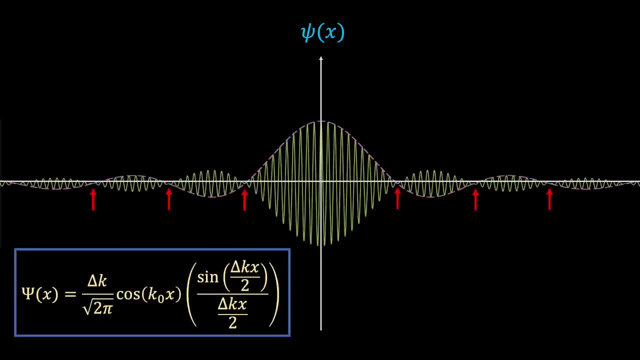 that there are a series of points along the x-axis between the lobes where the wave function reduces to zero. These zeros correspond to the locations where the sine term inside the bracket reduces to zero. If we label the zeros either side of the central lobe as minus x-naught and 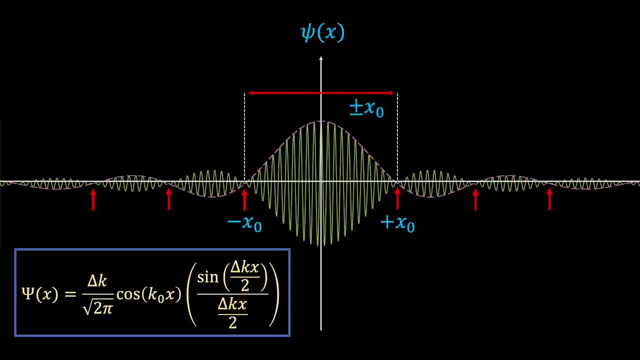 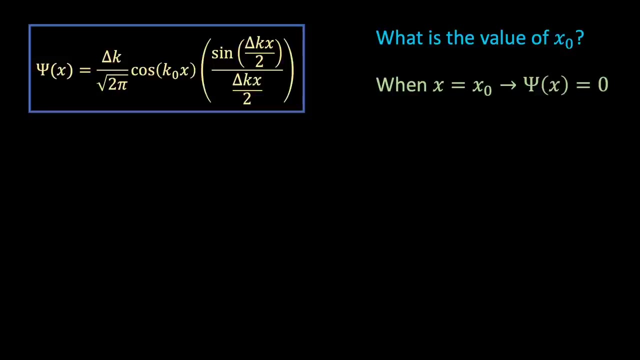 plus x-naught, then we can use these points to specify the width of our central wave packet. So can we actually determine this width by calculating the value of x-naught? Well, as already mentioned, when x equals x-naught, our wave function psi of x equals. 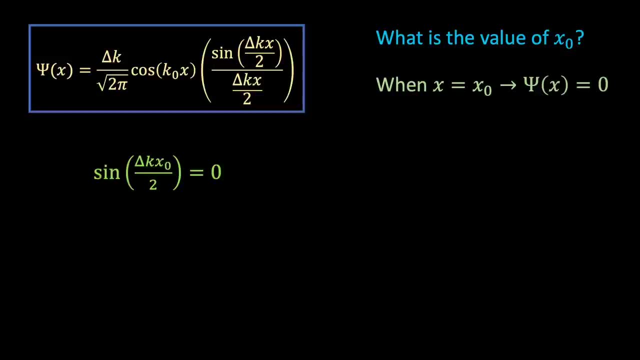 zero, And this occurs when sine of delta k x-naught over 2 equals zero. And, as you probably know, this first occurs when the argument of the sine function is equal to pi radians, In other words, when delta k x-naught over 2 equals pi, And this 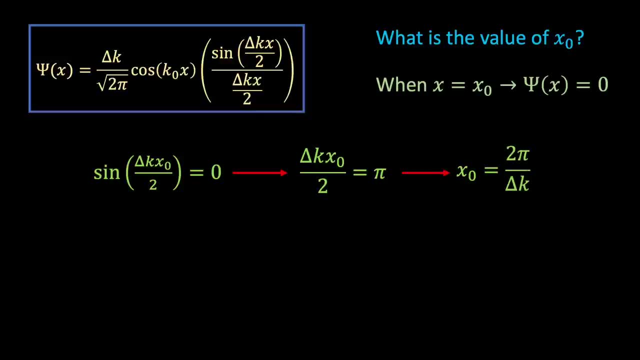 implies that x-naught equals 2 pi over delta k. Ok, but what is this x-naught relationship telling us? Well, if you recall, x-naught tells us the width of the central wave packet, And if we look at the x-naught relationship, we see that as delta k. 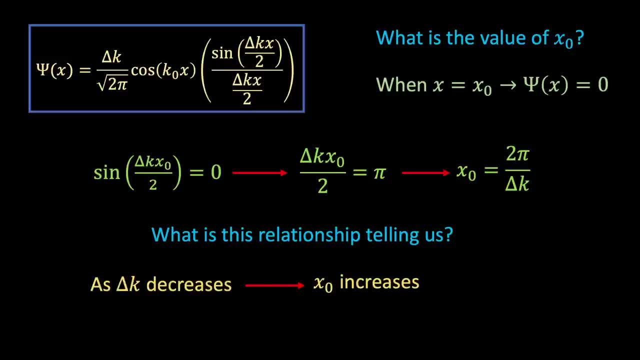 decreases, x-naught increases, Which is to say that the width of our wave packet increases. And since the wave packet tells us information about where we are most likely to find our particle, if the width of the wave packet increases, our uncertainty in where the particle is located must also increase, And we label. 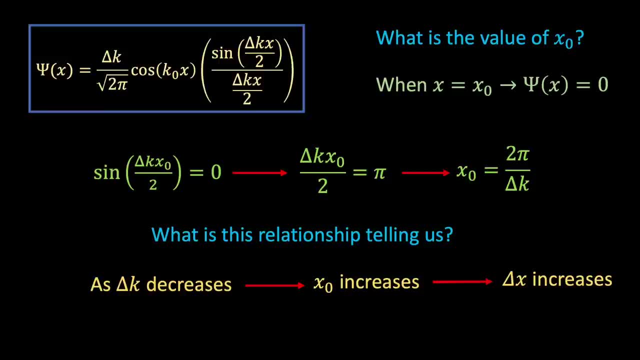 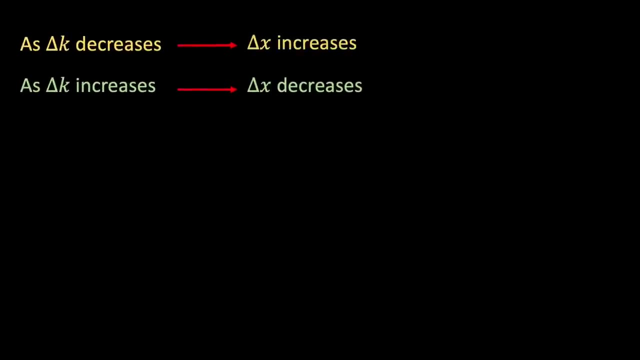 this uncertainty, delta x, Likewise as delta k increases, we see that x0 decreases and therefore our uncertainty in where our particle is located also decreases. We can summarise this result by saying that the product of delta k and delta x is equal to a constant, so that as one increases, the other decreases and vice versa, as can be seen. 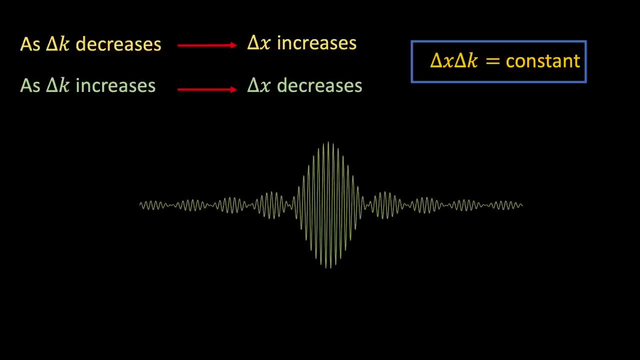 in the animation below. This is telling us that if we use a smaller range of k values, then when we superpose these waves, the resultant wave packet will be broader than if we had used a wider range of k values. We also notice that when delta k is equal to zero, this corresponds: 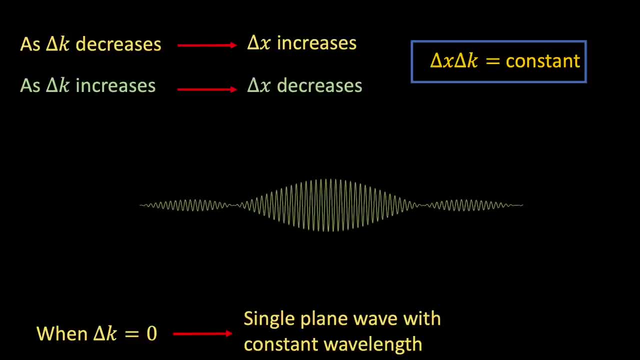 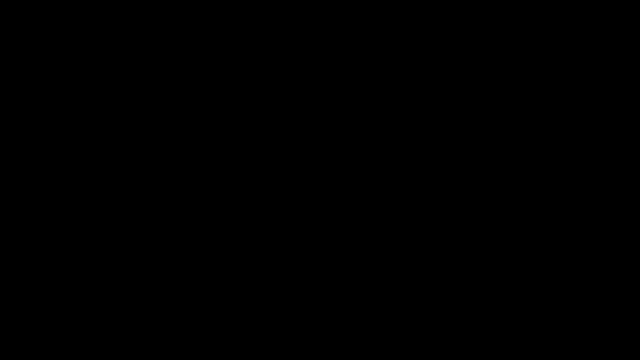 to a single plane wave with constant wavelength, in which case there is no superposition and our wave will extend throughout space, meaning that the uncertainty in the particle position would be infinite. Now, at this stage, it's worth noting that we can recast the condition that delta x times. 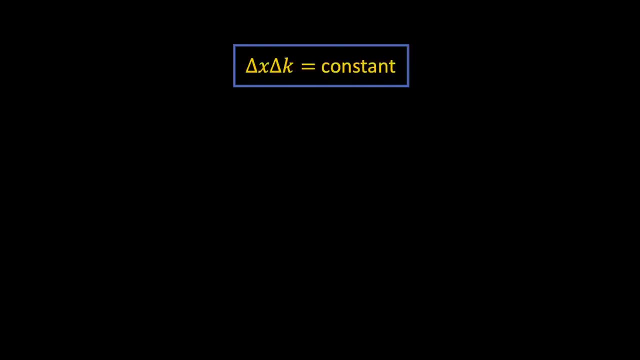 delta k is equal to 0.. We can then use our notation to calculate the density of the wave packet. We delta k equals a constant into a more suggestive form. If you recall, the momentum of a particle can be related to its wave number via the relation: p equals h bar k and therefore it: 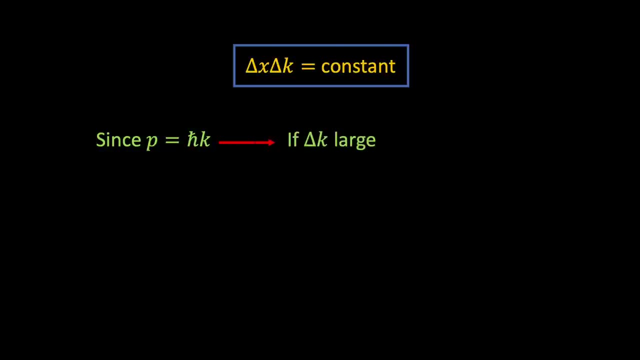 follows that a large range of k values amongst our component waves corresponds to a large range of possible momentum values of our particle, and so we see that we could equivalently write our delta x- delta k condition as delta x times delta p equals a constant, In other words, 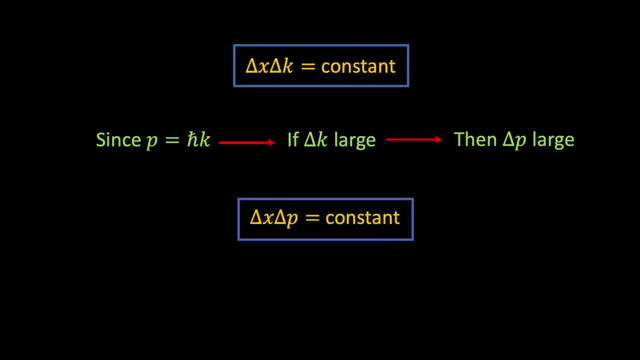 the uncertainty in the position of the particle multiplied by the uncertainty in its momentum is equal to a constant. This is telling us, for example, that if we have a narrow wave packet, which corresponds to a small uncertainty in where our particle is located, then this: 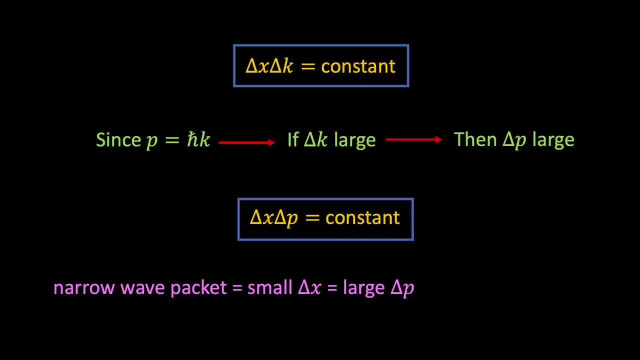 will correspond to a large uncertainty in the momentum of our particle, and vice versa. Now, the sharp-eyed amongst you will recognise this condition as being reminiscent of Heisenberg's uncertainty principle, and you wouldn't be wrong. We will certainly have more to say. 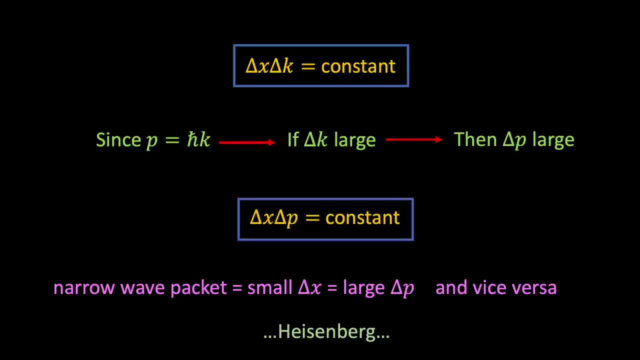 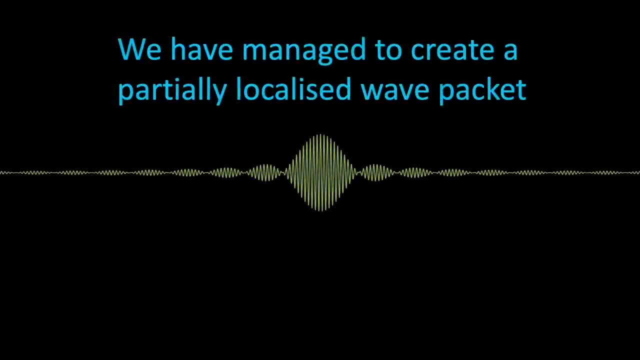 about this later, but before we get ahead of ourselves, we still have a few issues that require fixing. We have just seen that by using a continuous range of component wave functions, each with the same amplitude, we have managed to create a partially localised 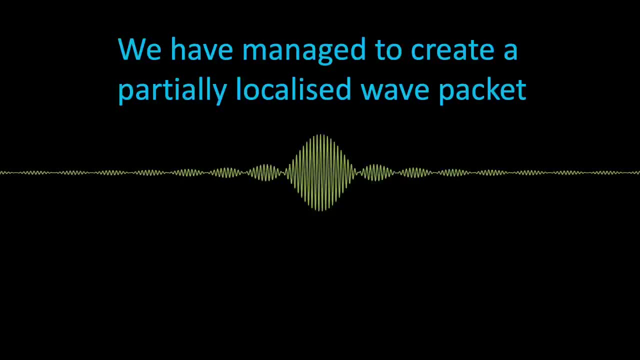 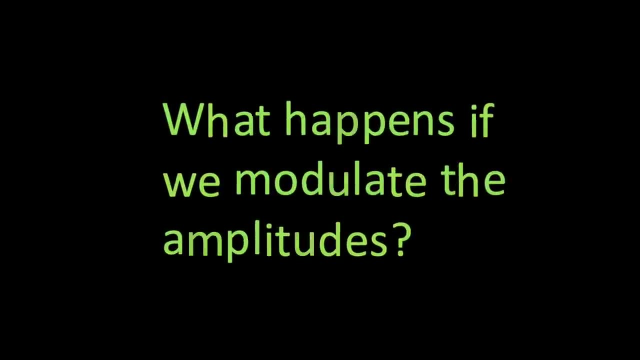 wave packet which is equal to delta x, delta k. Now if we have a large central lobe consisting of a large central lobe and multiple smaller side lobes, then the next question is: how do we get rid of the side lobes? Well, one. 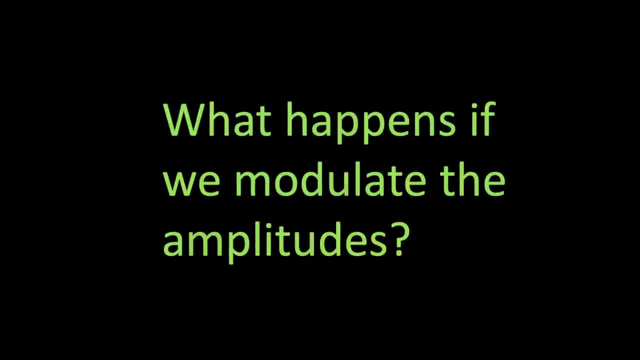 thing that we haven't yet considered is what happens if our component waves do not all have the same amplitude. In other words, what happens if we modulate the amplitude of our waves? So let's find out. To start with, let's return to our 5-wave example, with k values differing by pi radians. 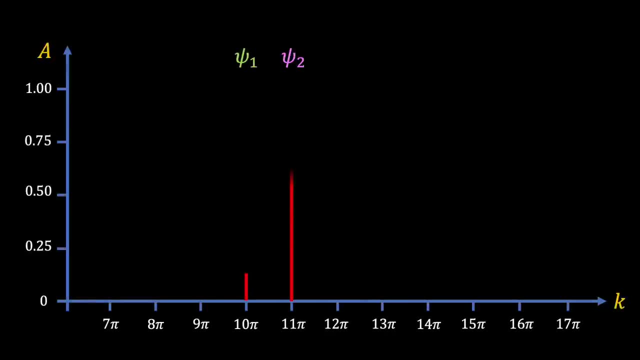 per metre And plot a graph in k-space. only this time we will modulate the amplitude of our waves so they fit inside a Gaussian curve. I'll have more to say about Gaussian bell-shaped curves a bit later, but for now simply notice that, for example, psi 1 and psi 5 have very 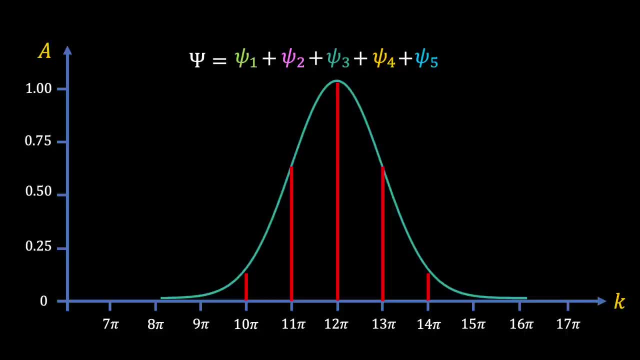 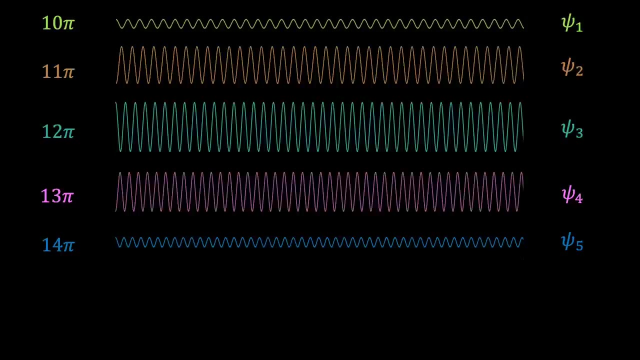 small amplitudes, and so they will not contribute as much to the net wave function, whereas psi 3 has a larger amplitude and therefore will contribute a greater amount when we add all the waves together. We can visualise each of the component wavefunctions in position space by plotting the corresponding 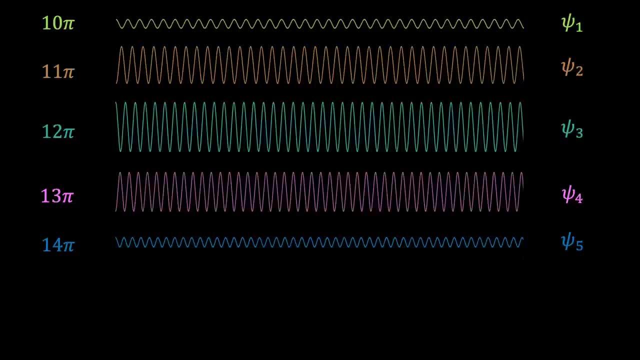 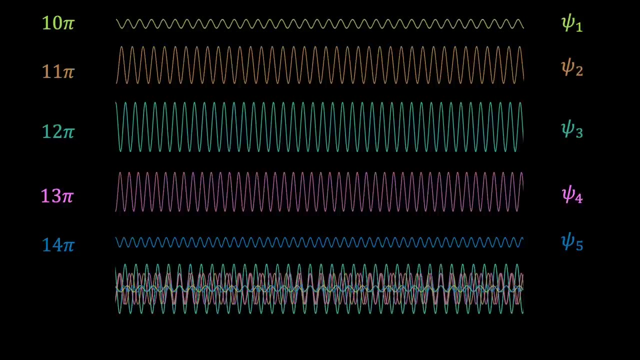 cosine waves, and this makes the differences in amplitudes manifest. If we then superimpose the waves on top of each other, we see that there are regions where the waves perfectly overlap and regions where they do not. What we now want to do is calculate the superposition. 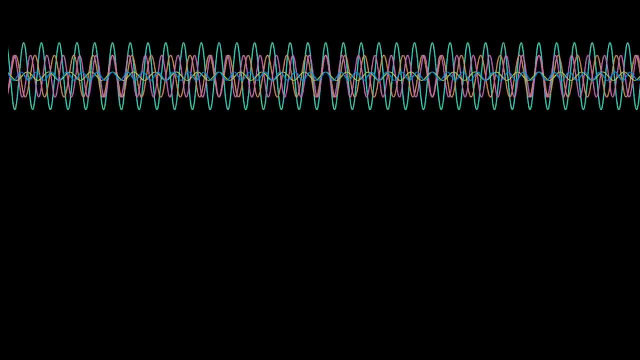 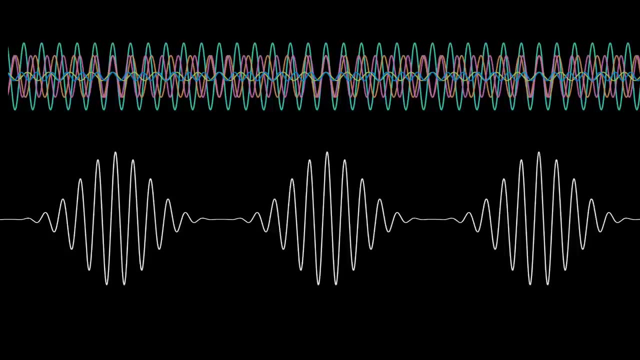 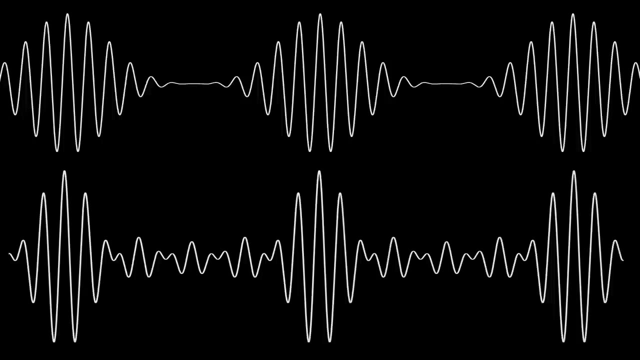 of these 5 waves. If we use the principle of superposition to add together the waves, we find the following resultant wavefunction pattern. Now it's worth comparing this with the constant amplitude 5 wave example we looked at earlier. We see that the effect of modulating the amplitude of our waves is to remove the small fluctuations. 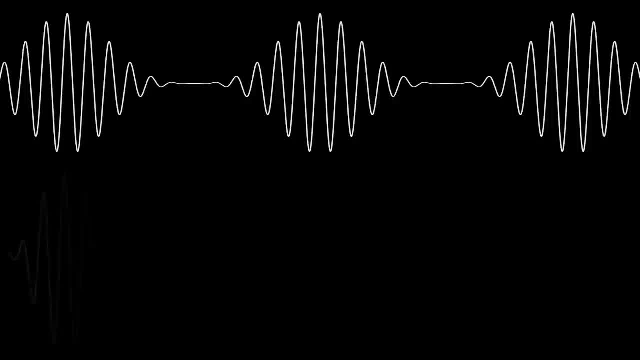 that existed between each wave packet, And so we see that the resulting wave packets are more clearly defined in space. However, we encounter the same issue that we previously encountered when considering 5 waves with equal amplitude, namely the fact that there are still multiple wave packets. 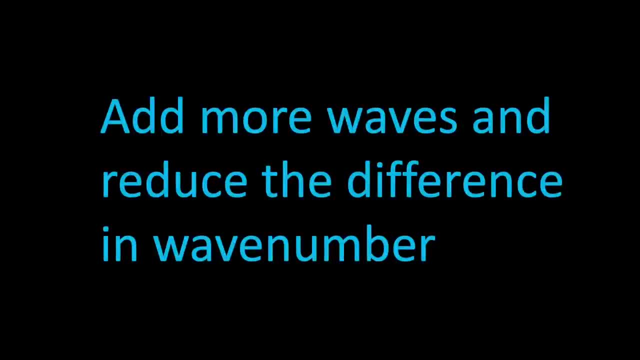 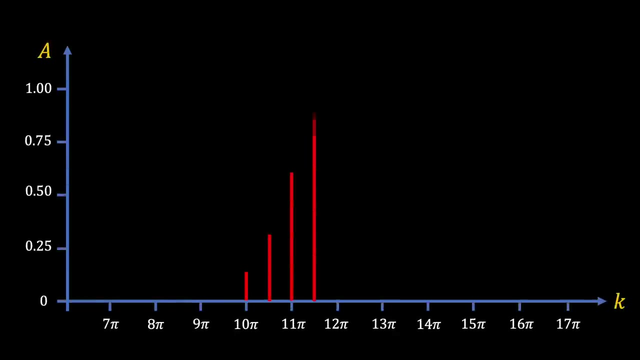 And so we will follow the same logic as before and improve our situation by adding together more waves and reducing the difference in wavenumber between the component waves. So let's do that. And so, if we take our modulated amplitude example, but this time consider the superposition. 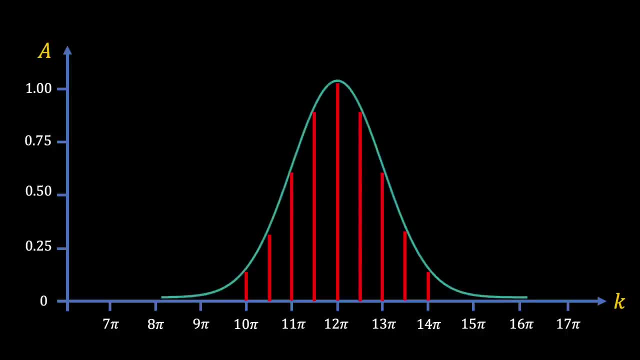 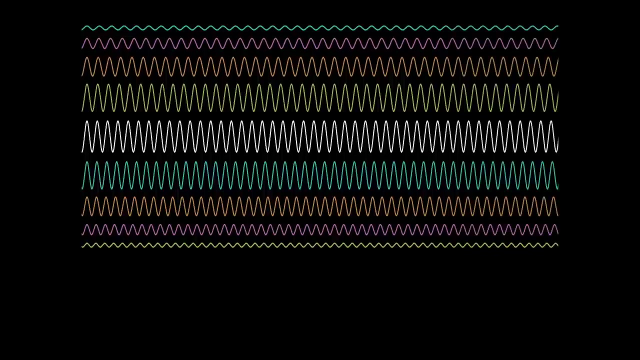 of 9 waves, each differing in k-value by pi over 2 radians per meter, then we can represent this in k-space using the following Gaussian distribution of amplitude values. If we were to visualize each of the component waves, we would see the following distribution: 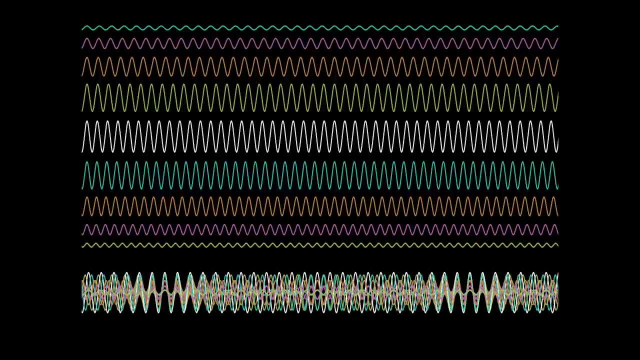 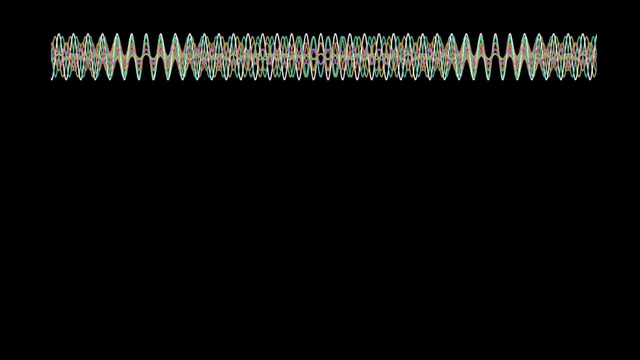 and if we superimpose these on top of each other, we again notice regions in which all the component waves perfectly overlap and regions where they do not. If we then apply the principle of superposition to add together the waves, we will see that the waves are 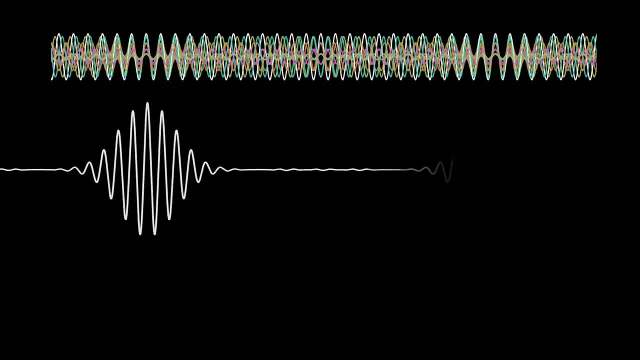 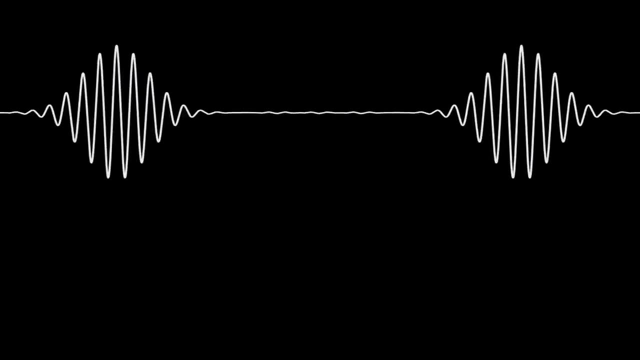 more clearly defined in space and that the waves are more clearly defined in space. And if we add these component waves together, we find the following resultant wavefunction pattern. And if we compare this to the 5 wave modulated amplitude example we saw earlier, then we: 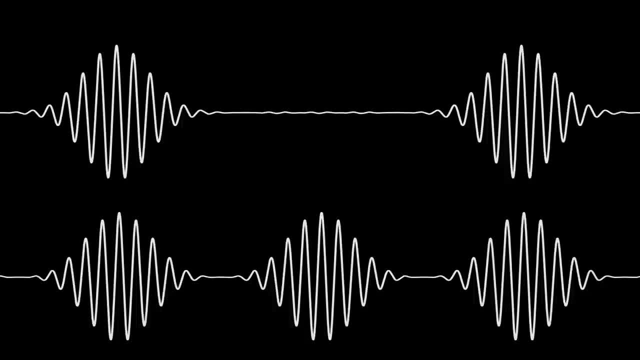 see that by increasing the number of component waves to 9, and by reducing the difference in wavenumber between the waves, we have managed to increase the space between adjacent wave packets whilst at the same time minimizing the small fluctuations between the wave packets. 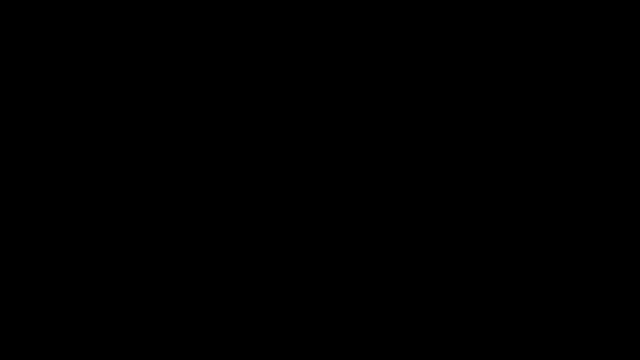 And so, hopefully now it should be obvious what the next logical step is. To obtain a single, well defined, isolated wave packet, we need to add together an infinite number of waves that differ infinitesimally from each other in their k-value. 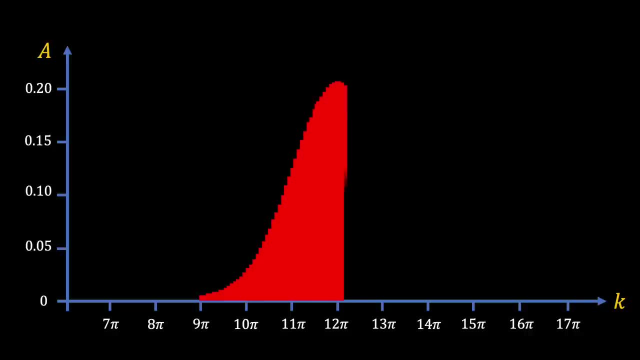 From a case-based perspective, this would correspond to adding a continuum of k values with amplitudes that fit inside a Gaussian envelope. We would then have to add some values to this random wave, So we would then have to multiply the values respectively and then. 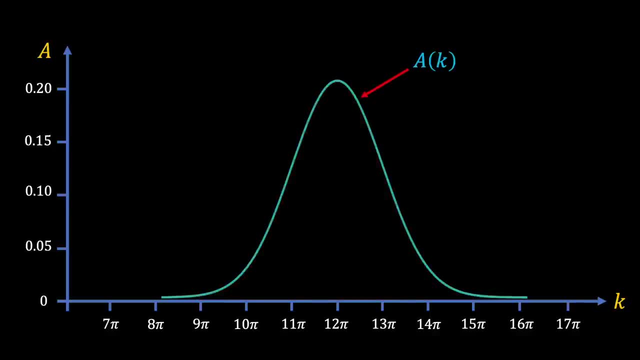 do the same thing all over again. The Gaussian envelope represents the entire loop that fits into the Gaussian envelope. The Gaussian envelope represents the entire loop and therefore the represents the amplitude function a, which tells us how the amplitude of our component waves are modulated for different k values. And so, to summarise, our claim is that the 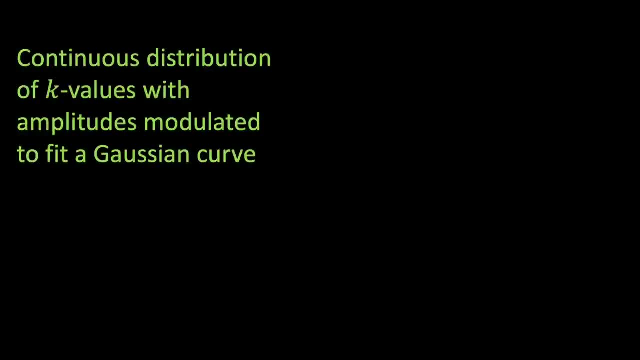 superposition of a continuous distribution of k values, with amplitudes modulated so that they fit inside a Gaussian curve, will lead to the creation of a single, well-defined, isolated wave packet, and that this wave packet will provide probabilistic information about where we are most likely to find our particle. And so our next question is: how do we describe? 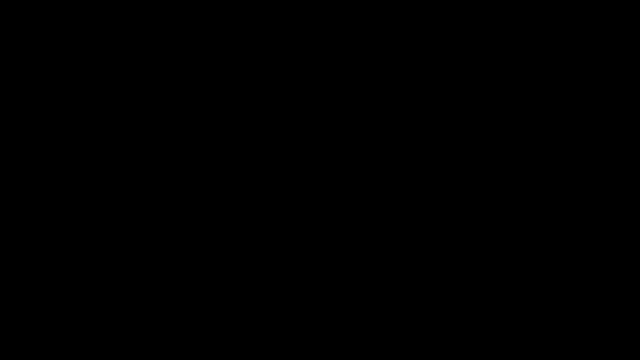 this wave packet mathematically Well, the good news is that we've already laid some of the foundations. We have already seen that for a continuous distribution of k values, the resultant wave function can be calculated using the following integral expression. Now 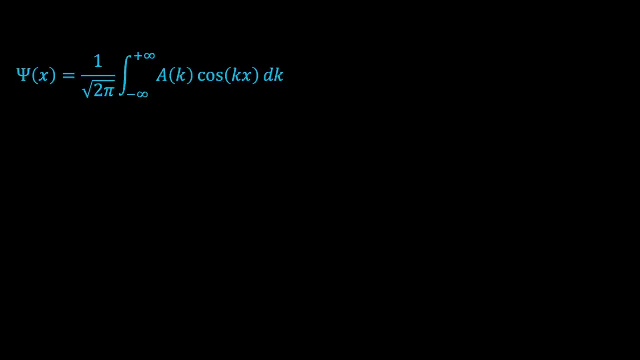 there is one small change that we will make to this equation, and this is a reflection of the fact that, in quantum mechanics, the wave function is generally a complex function involving imaginary numbers. As a result of this, we will replace the cos kx term appearing inside the integral with an e to the ikx term where, if you recall, 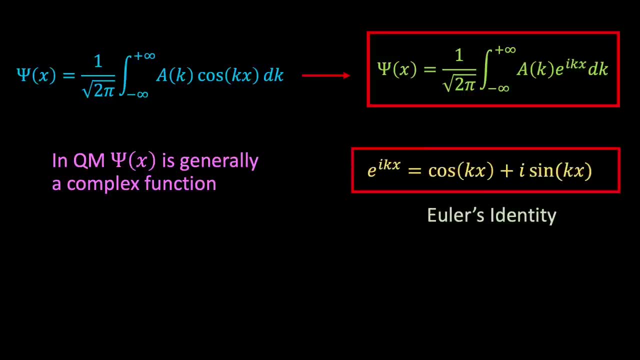 from my video on the Schrodinger equation. Euler's identity tells us that e to the ikx is equal to cos kx plus i sine kx, And so we see that if we take the real components of our composite wave function, then we recover the same expression that we had before. 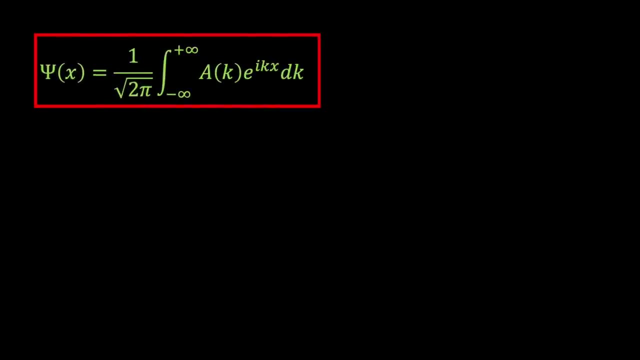 Our ultimate goal is to use this general integral expression to calculate the wave function corresponding to our localised wave packet. To do this, we first need to specify the form of the amplitude function, a, and, as I've already mentioned, we will be assuming that a is described by a Gaussian distribution. And so our next immediate 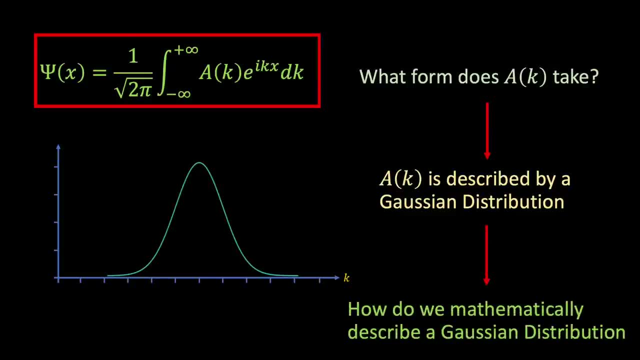 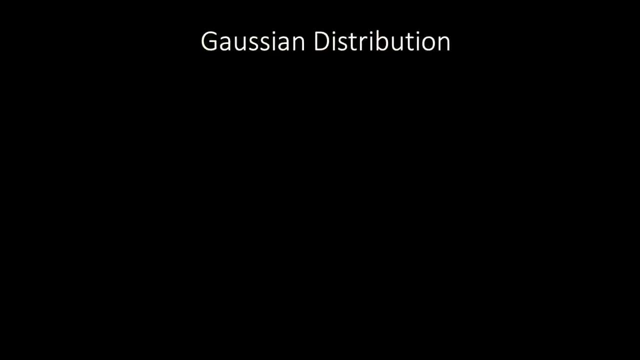 task is to understand how to mathematically describe a Gaussian distribution. So let's do that. A Gaussian distribution, also known as a normal distribution, is a characteristic bell-shaped continuous probability distribution and can be represented by the following rather ghastly mathematical function: where the mean value of x corresponds to the peak of, 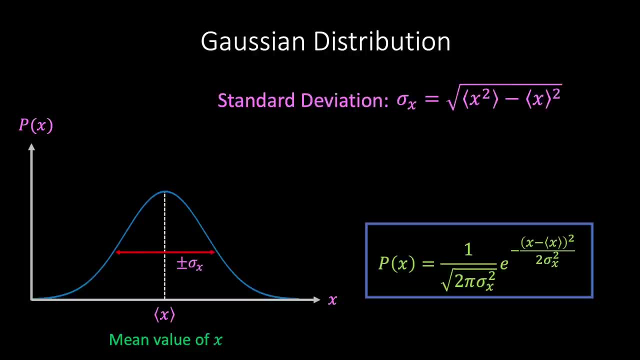 the curve, and sigma x represents the standard deviation of the Gaussian distribution which, if you recall, is defined as the square root of the difference between the mean of the square of x and the square of the mean of x. You can think of the standard deviation. 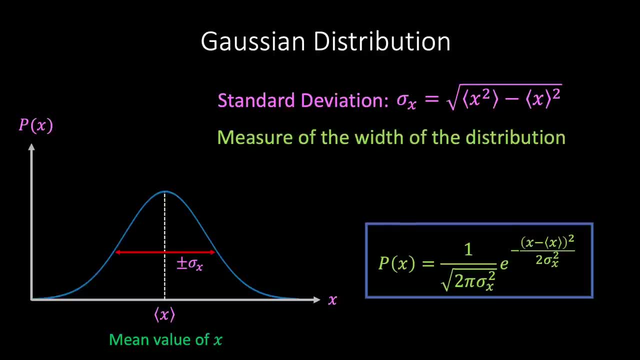 as a measure of the spread or width of the distribution and, within the context of quantum mechanics, the standard deviation in x is often referred to as the uncertainty in x, The function p is referred to as the probability density function. and if, for example, 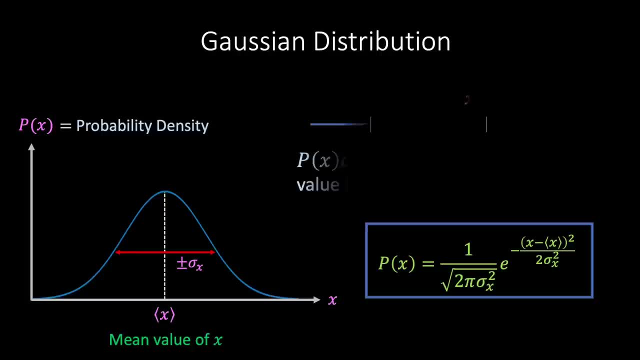 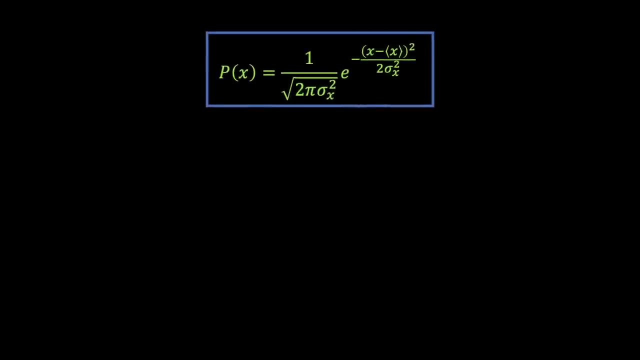 we wanted to find the probability that our x-value lies between a and b, then we would need to take the value of x and the value of x plus dx. then this would be equal to p times dx. What is important for us is the p function itself. 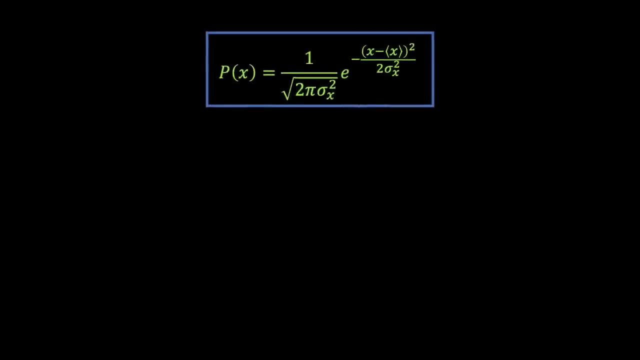 To emphasise the relationship between the standard deviation sigma x and the width of our Gaussian distribution, let's plot our Gaussian function and then slowly increase the value of sigma x appearing in our probability density function. We see that as sigma x is increasing, the width of our distribution increases, and so we can conclude that sigma 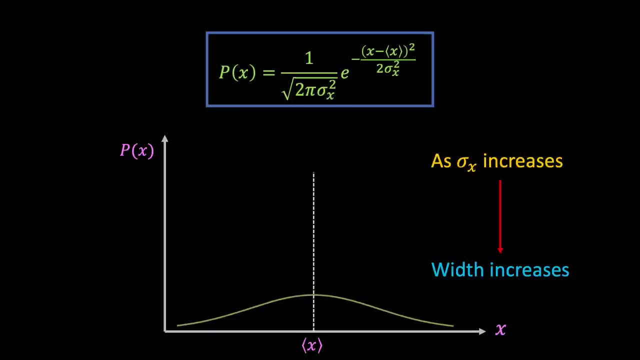 x is a good measure of the width of our Gaussian distribution, since it controls how quickly the exponential term appearing in the probability density function approaches zero. The final thing worth mentioning is that the constant coefficient term multiplying the exponential is a normalisation factor that ensures that, when we add up all of the probabilities, 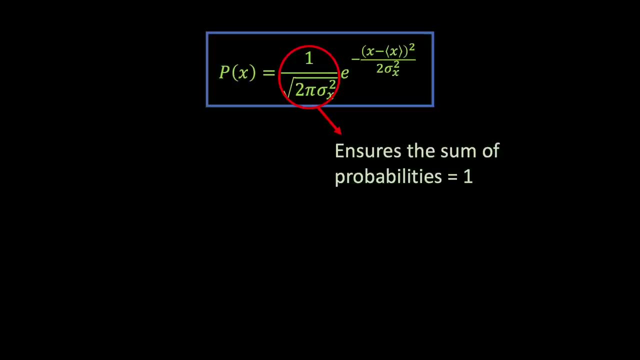 corresponding to each other, we get a constant coefficient. The constant coefficient is equal to the sum total of x, which is equal to 1,. as is required for a probabilistic interpretation, This is equivalent to requiring that the integral of the Gaussian distribution, evaluated from: 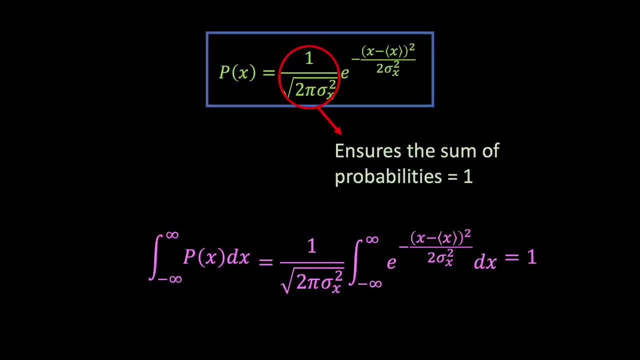 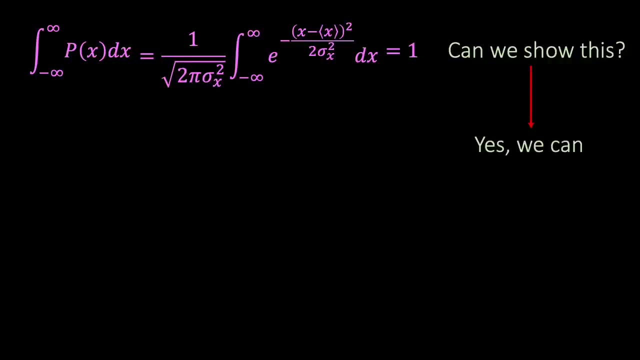 minus infinity to plus infinity is equal to 1.. So can we show that this is true? Well, thankfully, the answer is yes, but in order to do so, we will need to take a very quick detour and remind ourselves how to evaluate Gaussian. 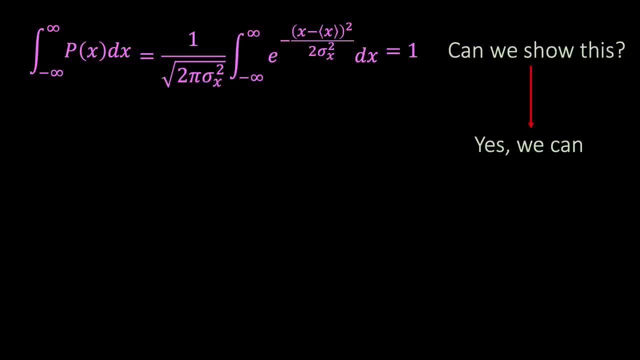 integrals. So let's quickly do that. Let's consider a simplified form of a Gaussian integral in which we define i as the integral of e to the minus x squared dx evaluated from minus infinity to plus infinity. To begin with, because of the symmetrical shape of 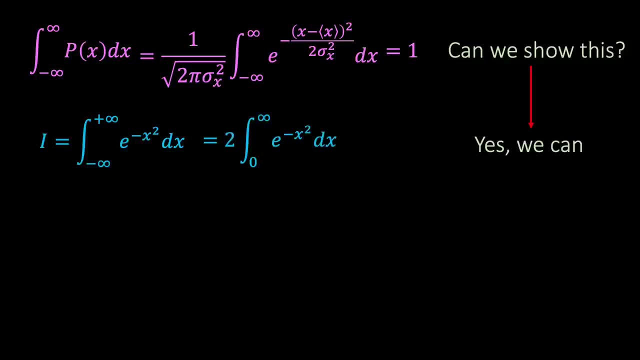 the function. we can write this as two times the integral of the same function, from 0 to infinity. Next, consider the square of this expression. i squared, In other words, the. consider multiplying the integral of e to the minus x, squared dx, by the integral of e to the. 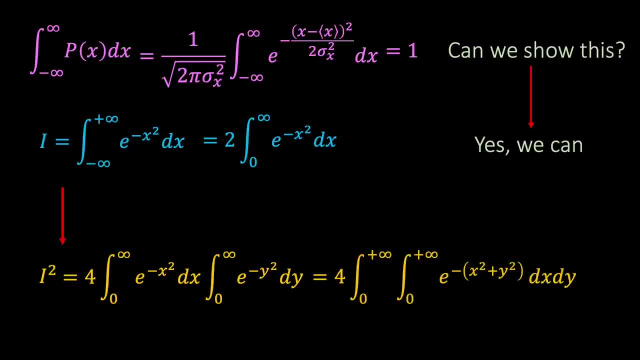 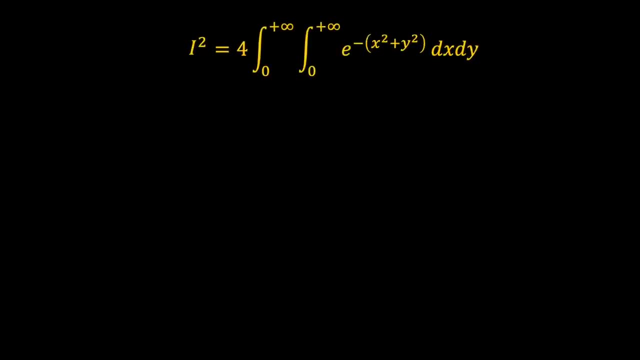 minus y squared dy. We can then combine the exponential terms and write i squared as a double integral. So how do we evaluate this integral? At first appearance, this doesn't look any better than the integral we started with, But there is a trick, and the trick is to. 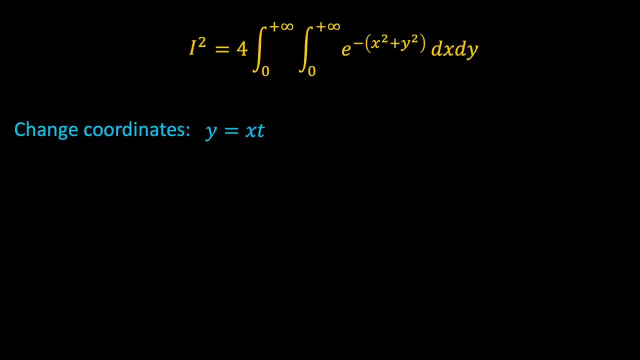 change variables. If we define y equals xt, then we see that t equals y over x and dy equals x, dt and the limits of our y integral change from y equals 0 and y equals infinity to t equals 0 and t equals infinity. If we then substitute this change of variables into our expression for i. 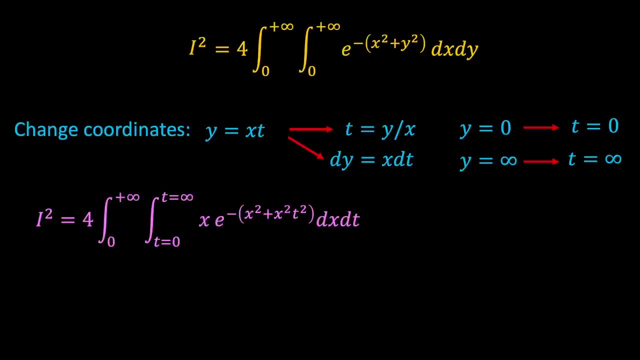 squared, we find the following pink expression: And if we then pull out a factor of x squared out of the bracket appearing in the exponential, we find the following green expression: Next we change coordinates again and let u equal minus x squared times 1 plus t squared, in which case du equals minus 2x times 1 plus. 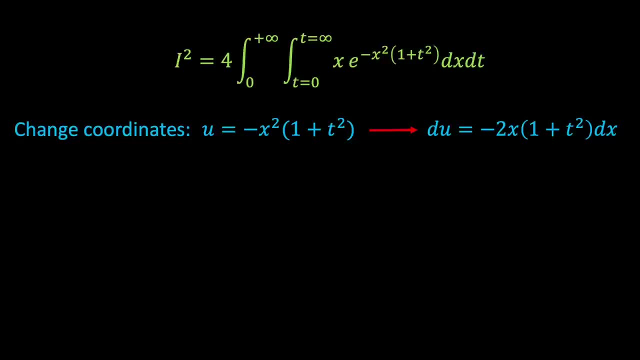 t squared dx. And, as a result of this change of variables, the integral limits will range from u equals 0 to u equals minus infinity. If we sub these relations into our expression for i squared, we find the following yellow expression: We can now perform each of the integrals separately. Firstly, 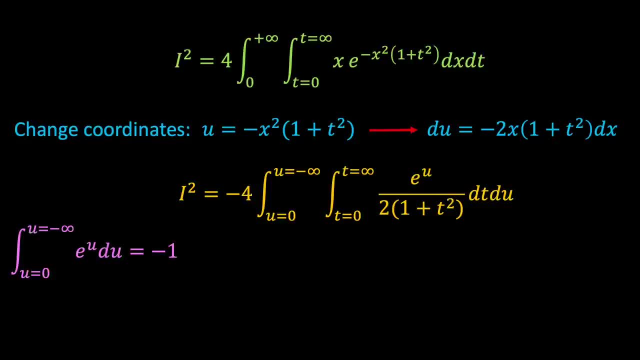 the integral of e to the u du from 0 to minus infinity, is equal to minus 1.. And that just leaves the integral of 2 times 1 over 1 plus t, squared, evaluated from 0 to infinity. This is a standard trigonometric integral which is equal to 2 tan to the minus 1 of t evaluated. 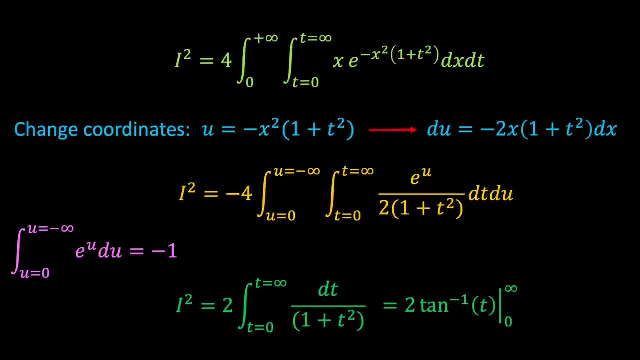 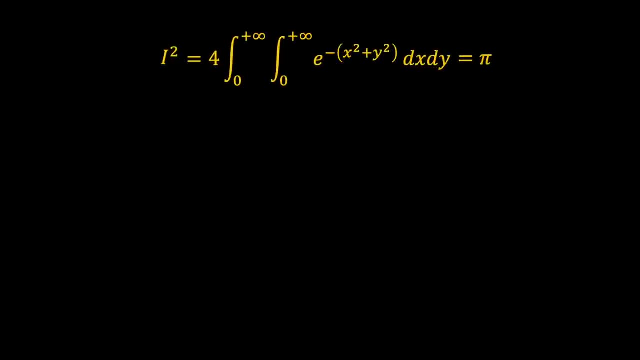 between the limits of t equals 0 and infinity, And this is simply equal to pi. And so, when the dust is settled, we see that i squared equals pi, and therefore it follows that our Gaussian integral i is equal to the square root of pi, And we arrive at one. 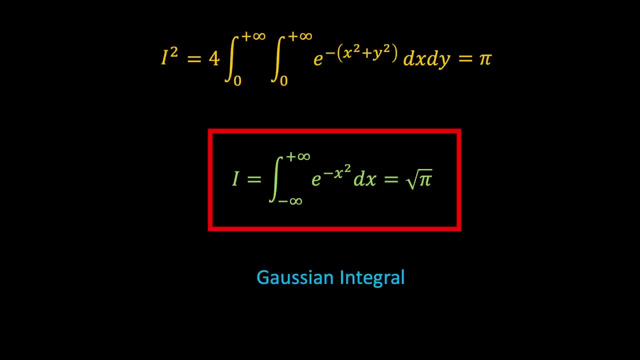 of the most famous results in mathematics, which is the fact that the integral of e to the minus x squared, evaluated from minus infinity to plus infinity, is equal to the square root of pi Gaussian integral. Now, it's a relatively straightforward exercise to generalize. 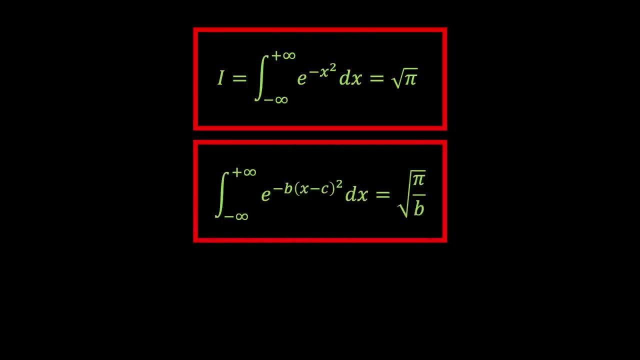 this analysis and consider the more general Gaussian integral where b and c are constants, and we find in this case that the integral is equal to the square root of pi over b, and this is the result we were looking for. We can now go back to the original Gaussian expression that we started with and use the result we've 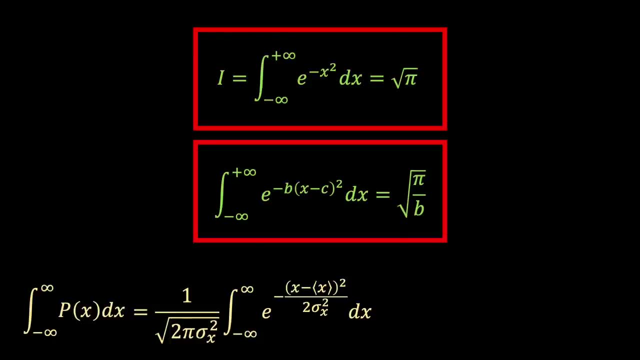 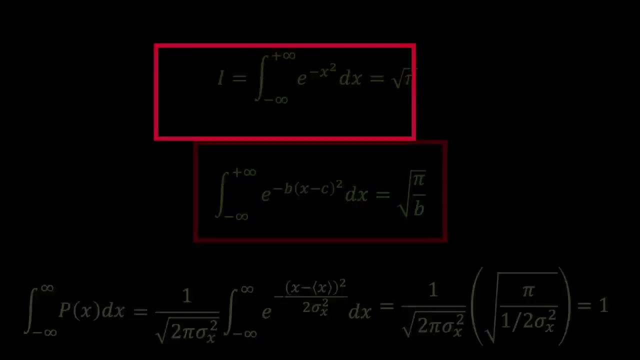 just derived. to show that the Gaussian function is normalized, We simply set b equal to 1 over 2 times sigma squared, in which case our integral takes the following form: and this just simplifies to 1, as required. Okay, so let's just pause a moment and take stock of where we are and what 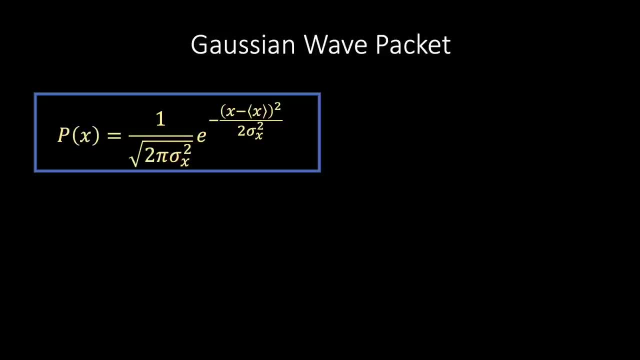 we've achieved so far. We have just had a crash course in Gaussian distributions and have found that the function p of x described a normalized Gaussian distribution and that the width of the function is characterized by the standard deviation sigma. If you recall the reason we were 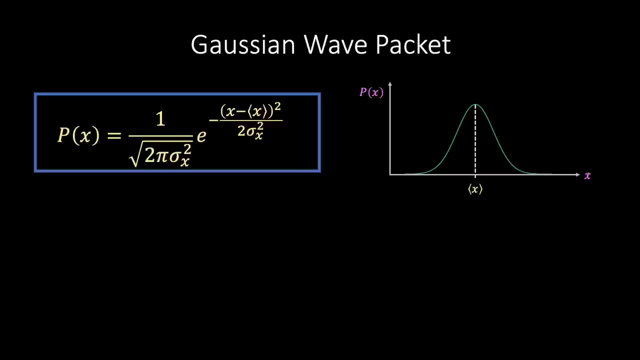 looking at Gaussian functions in the first place was because, when we were trying to construct a localized wave packet, it was necessary to add together an infinite collection of waves whose amplitudes differed in some way, and we found that if the amplitudes of the component waves were modulated according, 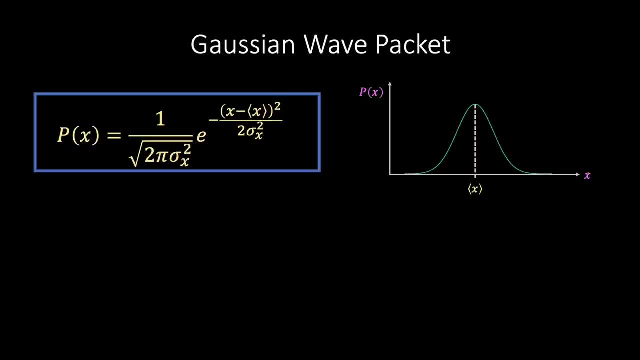 to a Gaussian distribution. then, when the waves were superposed, the resulting wave packet was localized in space. So what we now want to do is to show this explicitly by calculating the shape of the wave packet. in the case where our amplitude function a of k takes the form of a Gaussian. 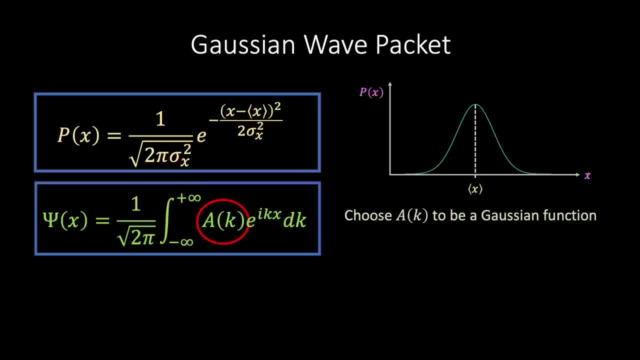 distribution. To do this, we will specify our a of k so that it takes a Gaussian form where alpha is a constant. The specific choice of coefficient will become clear shortly, Once we have constructed our wave function. So let's do that. We now have all the necessary ingredients to calculate our wave packet wave. 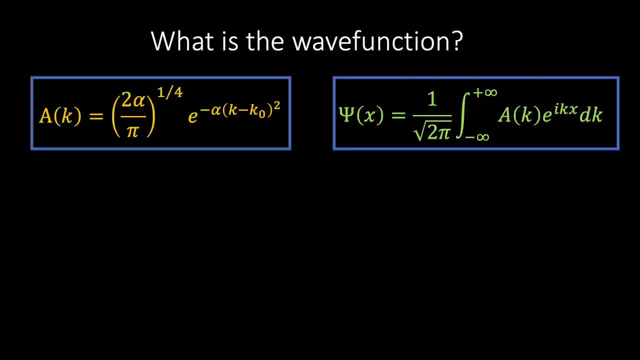 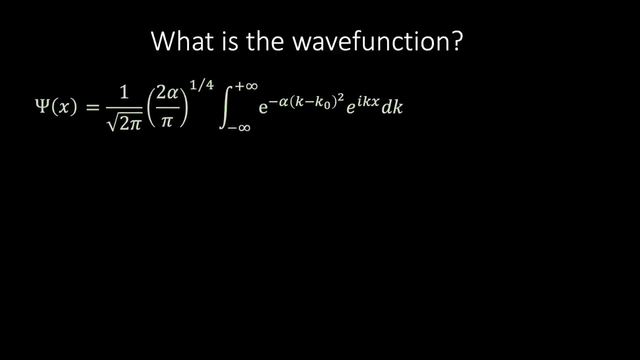 function. We simply need to substitute the explicit form of a of k into psi of x and calculate the resulting integral. If we perform the substitution, we find the following result: and this is what we now need to calculate. So how do we solve this integral? Well, the first thing that we can do, 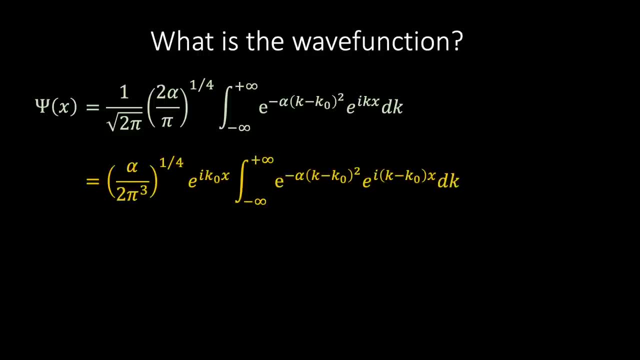 is rewrite the integral in an equivalent form, such that each exponential term includes a factor of k minus k nought. Next, we let k prime equal k minus k nought, in which case we see that dk prime by dk equals 1 and therefore dk prime is equal to dk. As a result of this, 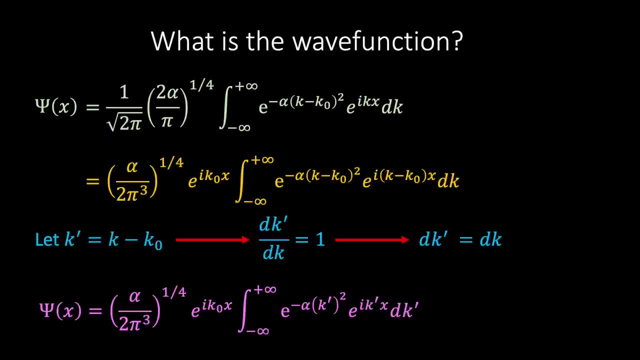 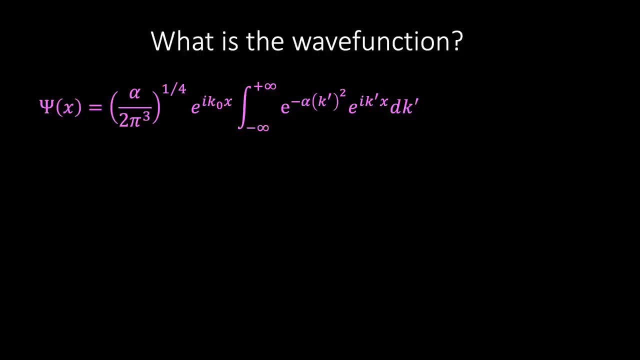 change of variables. our wave function takes the following form: So what next? Well, the trick is to combine the exponents in the two exponential terms and then strategically rewrite these terms in the following form: If we then insert this back into our integral, we can separate out the exponentials again. 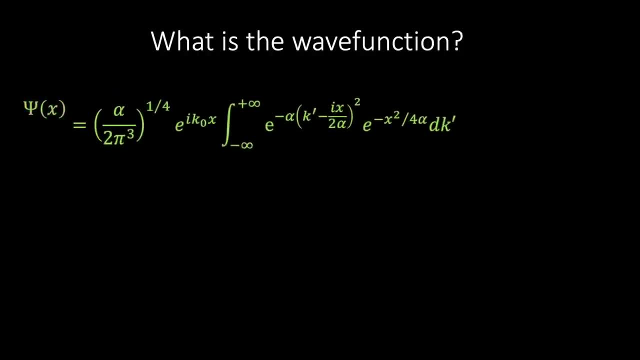 and we find the following green expression: Next, we can change variables again and define: k double prime equals k prime minus i, x over 2 alpha, from which it follows that dk double prime is equal to dk prime. If we then substitute this change of variables into our wave function, we find the following yellow expression: 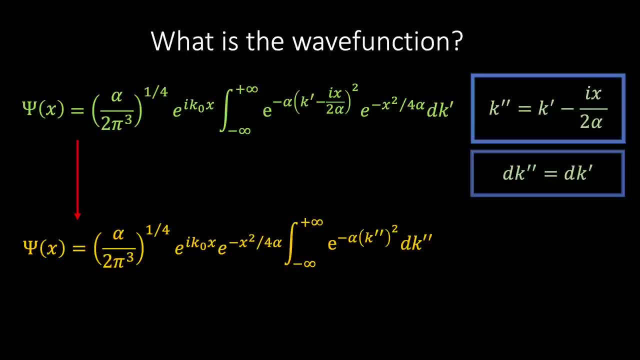 Next, we notice that, as a result of this change of variables, we are left with a standard Gaussian integral, and so we can use our result from earlier, which tells us that the integral will be equal to the square root of pi over alpha. And so, when the dust has settled, we see that. 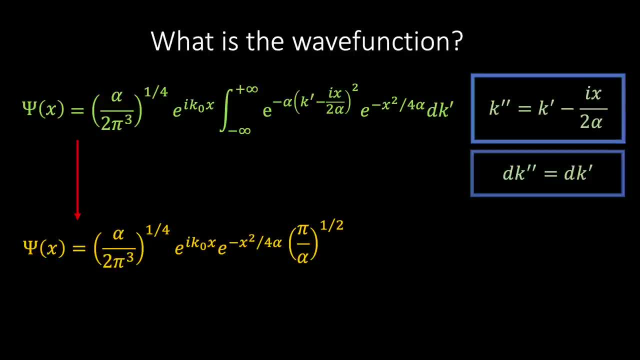 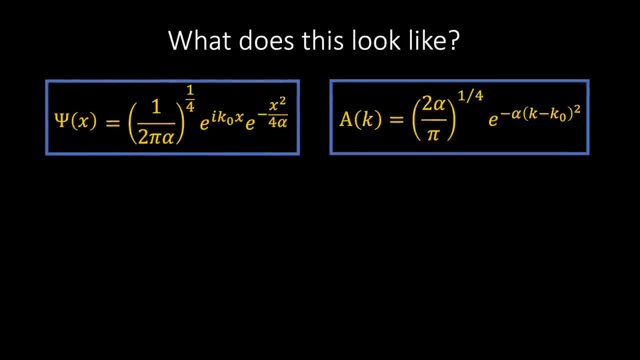 our wave function takes the following form, And if we simplify this expression, we finally arrive at the result that we were looking for. We have successfully managed to calculate an explicit expression for the wave function, for the example of a Gaussian amplitude function. So how do we interpret this result? What does 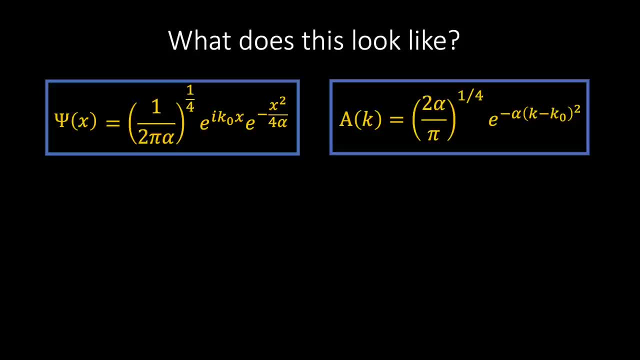 this wave function look like? Well, firstly, we notice that the wave function contains a complex exponential term as well as a Gaussian exponential term. We can visualise this function by looking at its real component, in which case we find the following result: Where we've made use of Euler's identity which, if you recall, says that e to the i kx. 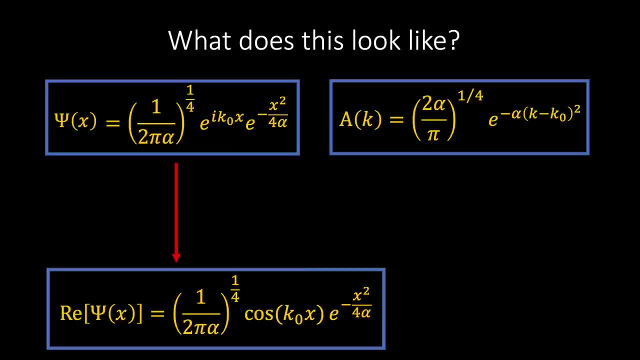 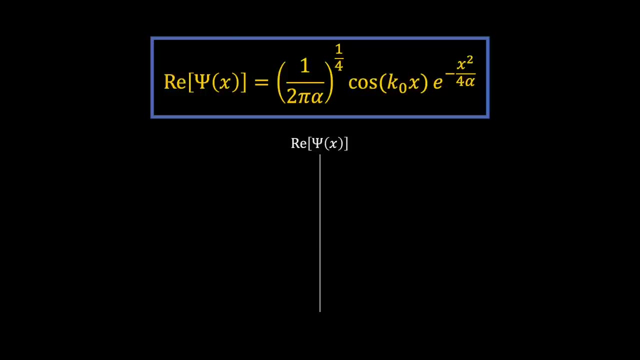 is equal to cos kx minus i sine kx, and the real part is the part that involves no factors of i. So let's now plot this function and see what we get. If we plot the real part of the wave function on the y axis and the x position on the x axis, then we get the following: 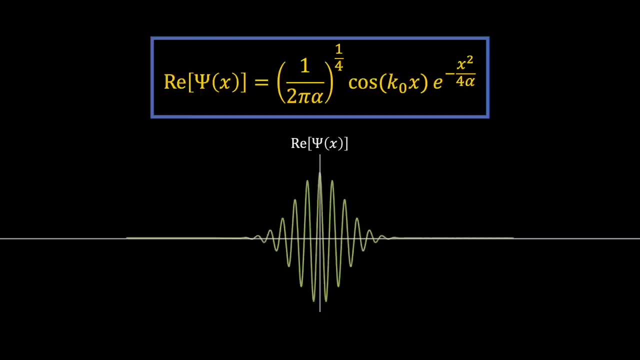 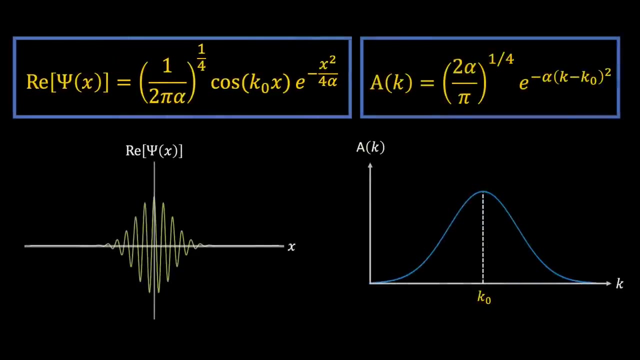 wave function distribution, And we can finally rejoice as we have managed to construct a well defined, isolated wave packet, which is precisely what we set out to achieve. Now, I'm not sure about you, but I find it incredibly satisfying to see the mathematical form of this wave function emerge from our detailed analysis. Our next step is to provide a physical 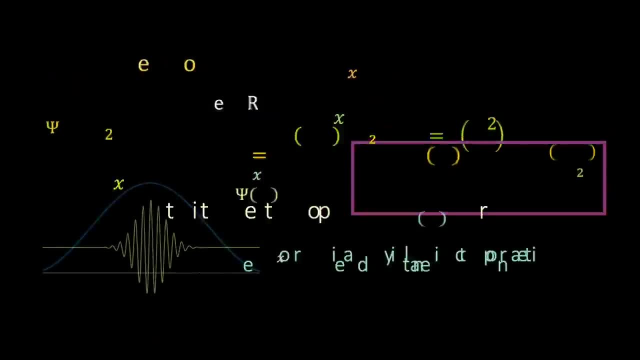 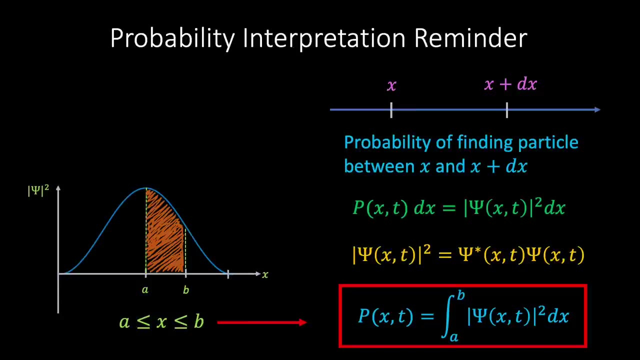 interpretation of this result. So let's do that. As mentioned earlier, according to the quantum mechanical framework, the position space wave function provides information about where we're most likely to find our particle And, as we've already seen, the probability of finding a particle between a location- x and x plus dx- is given by the modulus squared. 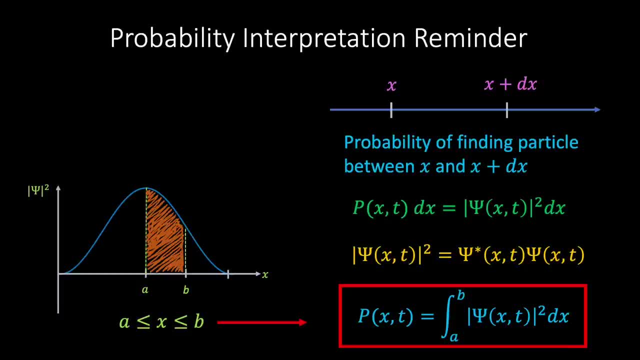 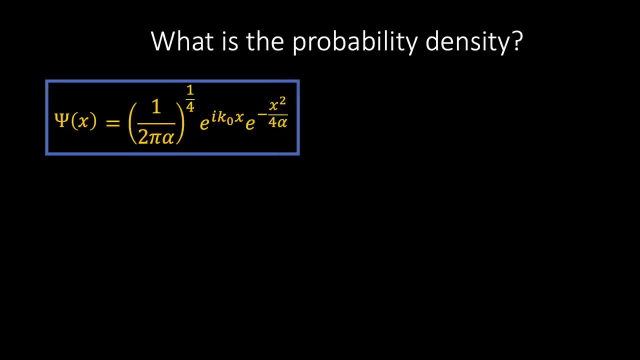 of the wave function, and this is crucially important, because it's actually the modulus squared of the wave function, rather than the wave function itself, that provides information about the probability of finding a particle in a particular region of space, And so our next task is to take the localized wave packet wave function that we've just 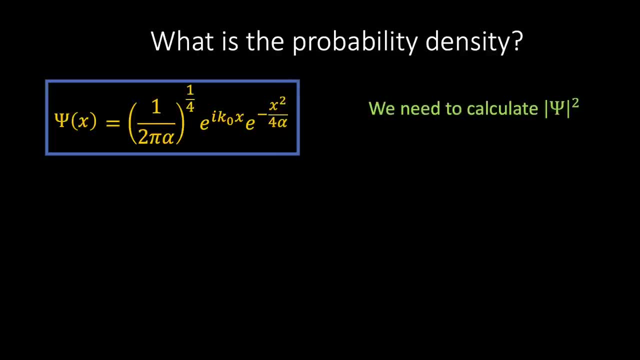 derived and calculate the modulus squared. To do this, we first need to calculate the complex conjugate of our wave function, and to do this we simply replace the i's with minus i's, in which case we find the following expression: If we then calculate the modulus, 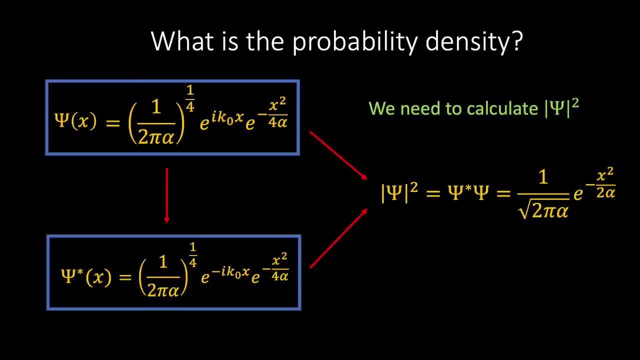 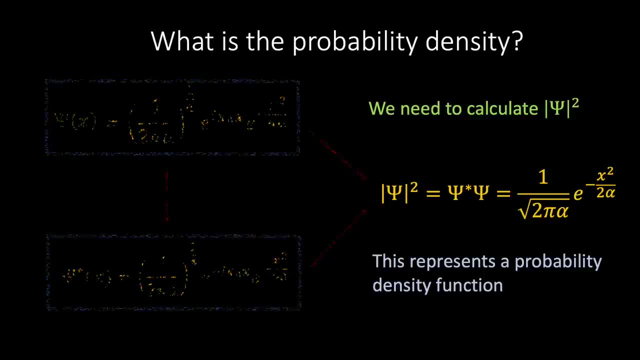 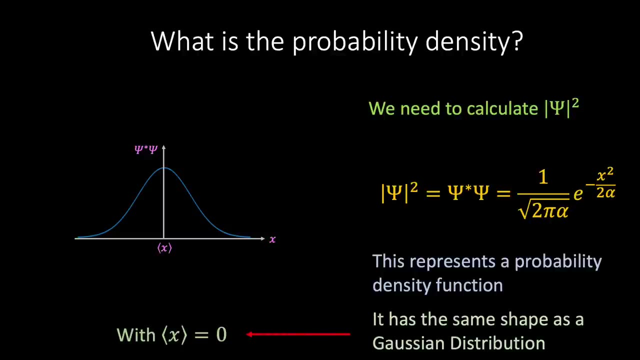 squared, we see that the complex exponentials have disappeared and we are left with a purely in probability density function which we can visualize by plotting the modulus squared on the y-axis and the position on the x-axis, And we see that the modulus squared function. 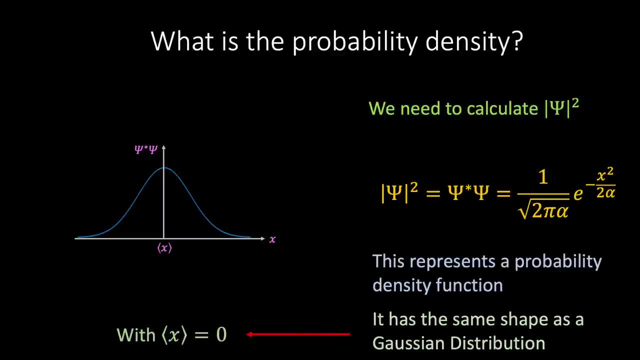 does indeed have the same shape as a Gaussian distribution, with the mean value centered at the origin, And it is the width of this distribution that we're interested in, as this will provide us with information about where the particle is likely to be located. 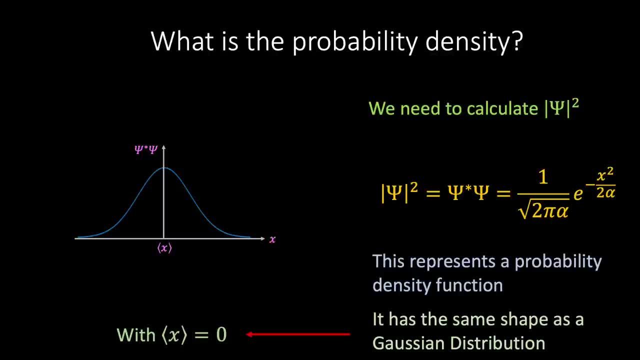 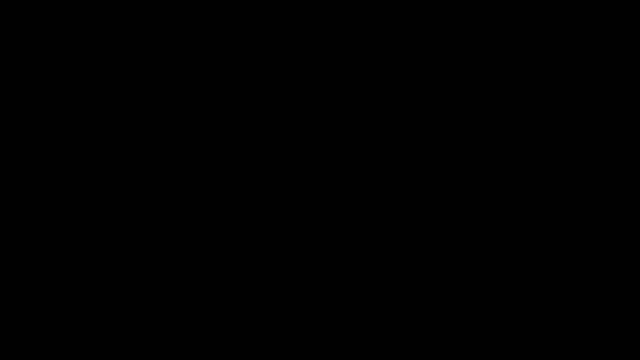 and therefore the uncertainty in the location of our particle. So let's just pause a moment and take stock of where we are. We have just seen that the modulus squared of our wave packet, wave function represents a probability density distribution that is Gaussian in shape. Furthermore, we saw earlier that a general Gaussian probability 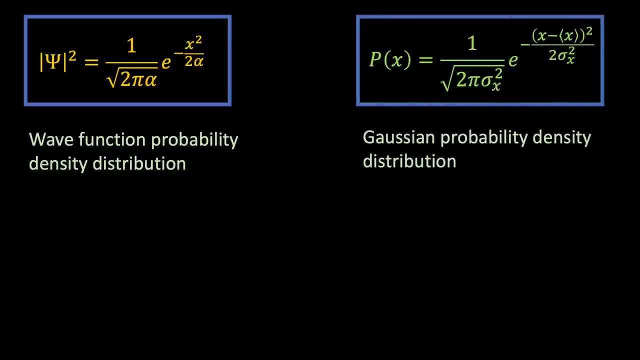 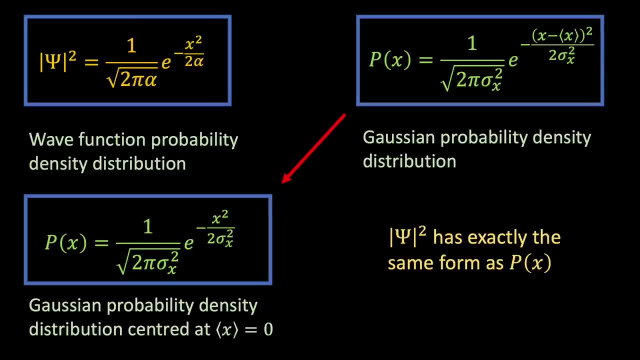 density distribution takes the following form: If we then assume that the wave packet wave function is centered at the origin, we see that our modulus squared wave function has exactly the same structure as the Gaussian probability density function p of x. And so let's see what happens. 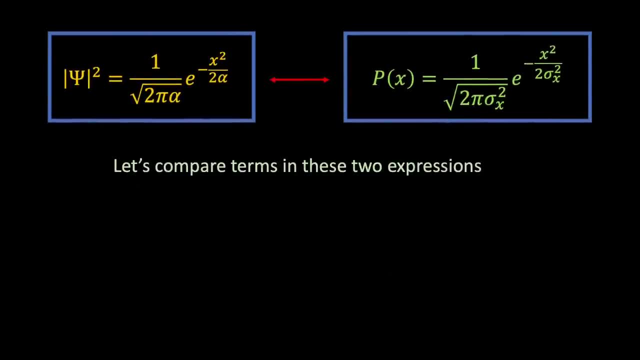 if we compare terms in these two expressions. A quick glance tells you that the two expressions are identical, provided that alpha equals sigma x squared, which implies that sigma x equals the square root of alpha. And so let's see what happens if we compare terms in these two expressions. 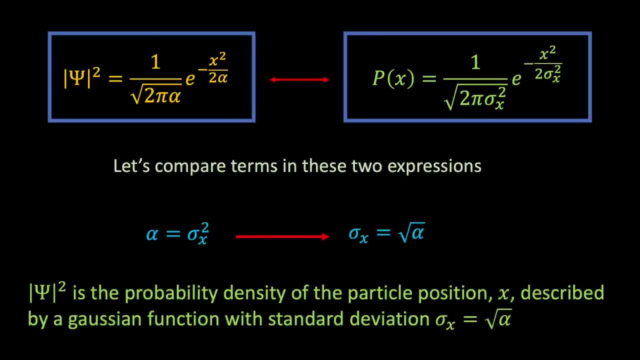 And so let's see what happens if we compare terms in these two expressions. And so let's see what happens if we compare terms in these two expressions. And so we see that the modulus squared of our wave function represents a Gaussian probability density distribution of our particle's position, with a standard deviation given by the square root of alpha. 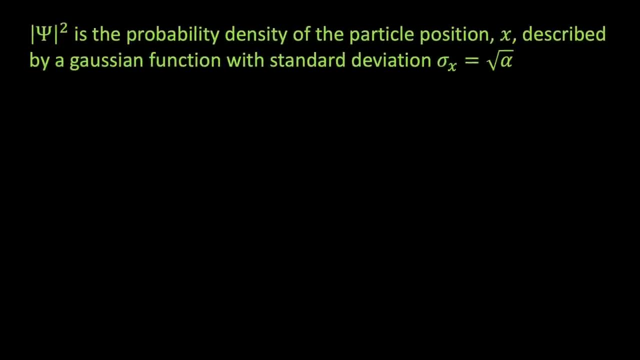 We will come back to this shortly Now. in much the same way that the modulus squared of our position space wave function provided information about the probability distribution of the particle's position, it turns out that if we take the amplitude function a of k, 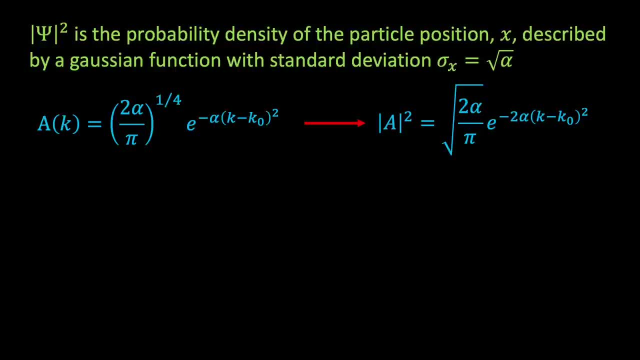 and calculate the modulus squared of this, then this represents the probability density distribution of the particle's wave number. We can see this explicitly by plotting the modulus squared of a on the y-axis and the k value on the x-axis, and we see that we do indeed get a Gaussian distribution. 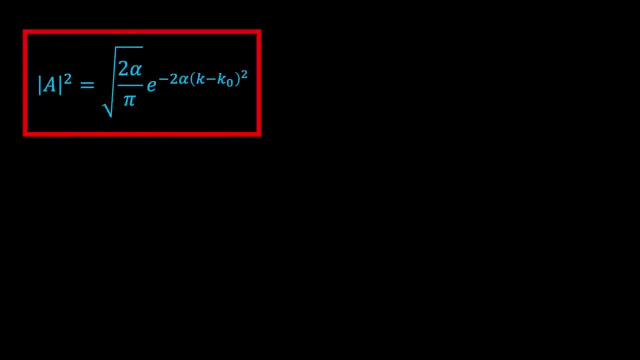 centered at k0.. It therefore makes sense to compare the modulus squared of our amplitude function with the general Gaussian probability density distribution of the particle's wave number. If we compare terms, then we see that the expressions are identical, provided that 2 alpha equals 1 over 2 times sigma k squared. If we rearrange this, we see that sigma of k. 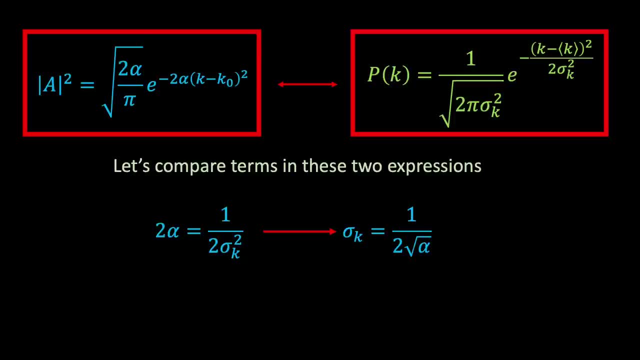 is equal to 1 over 2 times the square root of alpha, And so we conclude that the modulus squared of our amplitude function represents a Gaussian probability density distribution of the particle's wave number, with a standard deviation given by 1 over 2 times the square root of alpha. 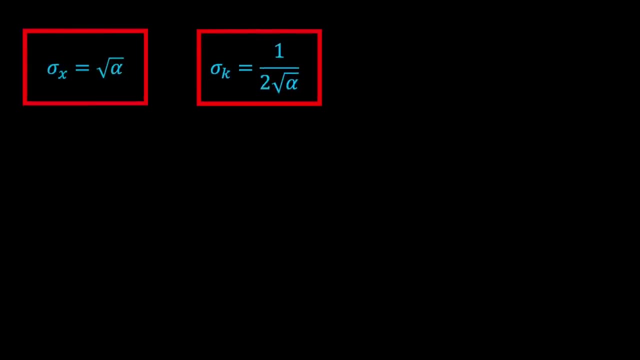 So let's pause a moment to gather our thoughts. We took the wave packet wave function and the amplitude functions that we determined earlier, and then we looked at the modulus squared of each, as these tell us something about the probability of finding a particle within a certain region of. 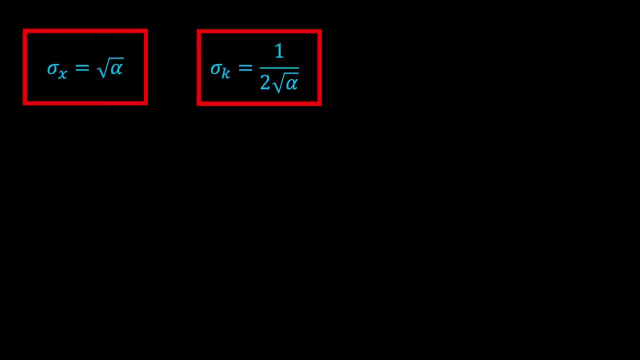 space or within a certain wave number of a particular region of space. We found expressions for the standard deviations of these probability distributions by comparing the modulus squared expressions with the general expression for a Gaussian probability distribution, and we found the following two results. Now, since the standard deviation provides information about the spread or width of the 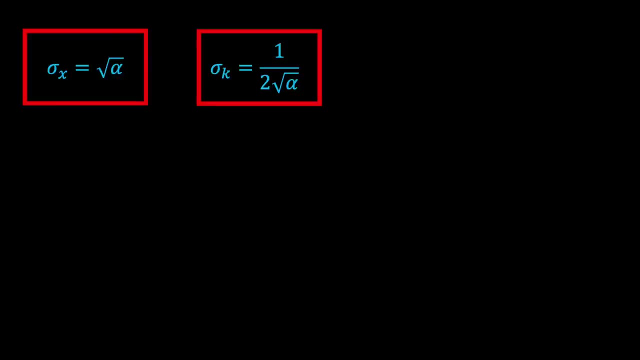 corresponding probability distribution. it is often referred to as the uncertainty, and so we will follow convention to determine the probability of finding a particle within a certain region of space. Now for the particleじゃない. we should write our set of values as both the delta x and delta k. 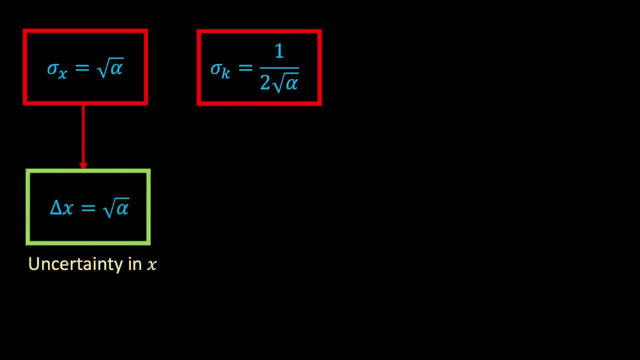 For the data acceleration. we can just use the delta x given at the bottom of our equation and then apply the delta x, and so we will take the delta x and the delta k together, which is two times the square root of alpha, and that will give us the value of delta x squared, which is 1 over. 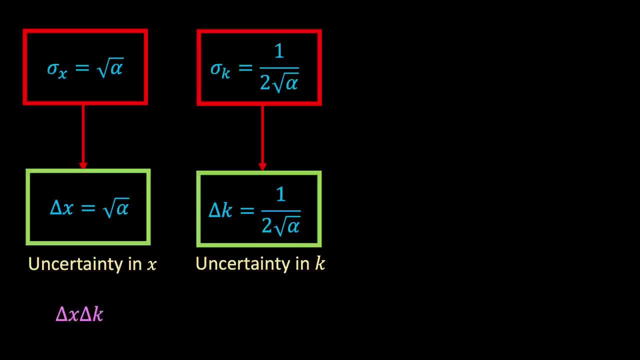 2 times the square root of alpha. Next, observe what happens if we multiply these two uncertainties together. We see that the product of the uncertainties is equal to half, and therefore we see that delta x times delta k equals one half. So what does this mean? Well, one way of visualising this result is to plot both the 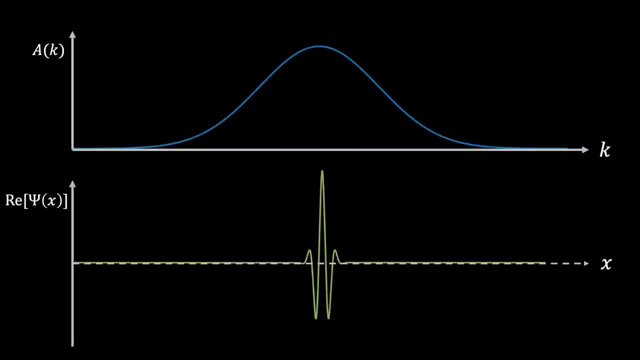 amplitude function, a, and the real part of the corresponding wavepacket, wavefunction, and then observe what happens to the width of the wavepacket as the width of the amplitude function decreases. We see that as a gets narrower, which corresponds to delta k getting smaller, the width of the wavepacket increases, which corresponds to delta x increasing. 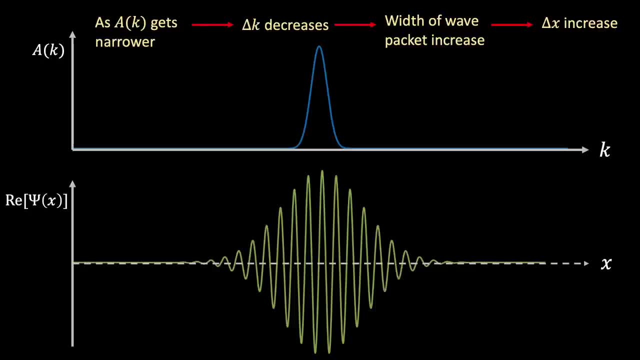 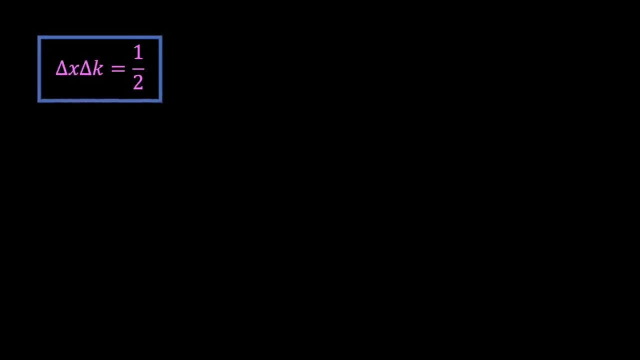 And furthermore, we see that the change in delta x and delta k are such that the product of these two always remains equal to one half. Now we saw earlier that the wavenumber is related to the momentum by the relationship p equals h bar k, and so it follows that delta p equals h bar delta k, and therefore we can. 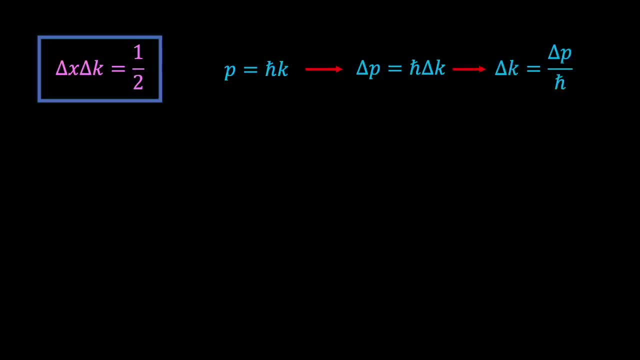 write, delta k is equal to delta p divided by h bar. And if we sub this into our delta x, delta k expression, we find that delta x times delta p over h bar is equal to one half. And if we rearrange this, we find a rather remarkable and perhaps familiar result. We see that the uncertainty 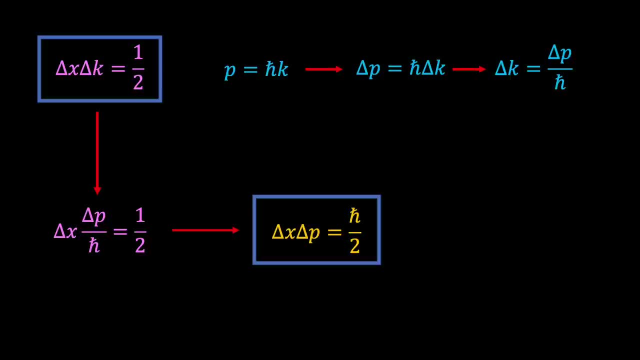 in particle position multiplied by the uncertainty in particle momentum is equal to the reduced Planck's constant divided by two. This expression is telling us that there is a fundamental limit to the precision with which the position and momentum of a particle can be known. We see that as we reduce the uncertainty in the particle's 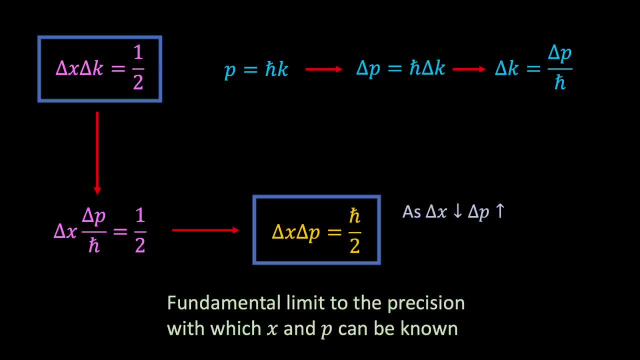 position, this leads to an increase in the uncertainty in the particle's momentum. And likewise, if we reduce the uncertainty in the particle's momentum, then we necessarily increase the uncertainty in the particle's position. And the beautiful thing is that we can now understand where this relationship comes from in terms of wave packets and the 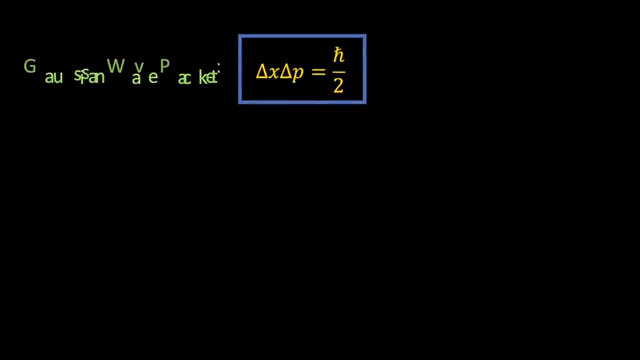 principle of superposition. Now it is worth emphasising that we have arrived at this result by considering a Gaussian shaped amplitude function. It turns out that if you repeat the analysis for any other amplitude function, then you will find that the product of the position and momentum uncertainties 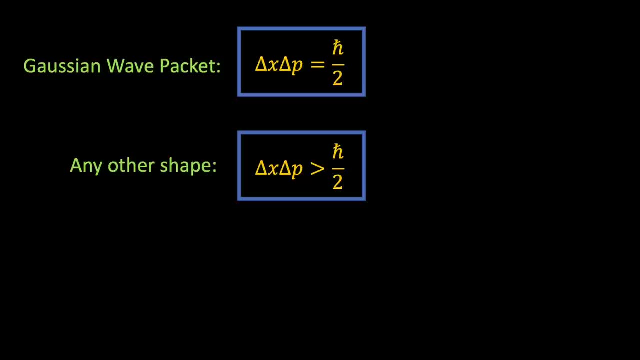 will be greater than h bar over 2.. And therefore the most general statement that we can write down is that delta x times delta p is greater than or equal to h bar over 2.. And this statement is known as Heisenberg's uncertainty principle. It is saying that precise knowledge of position. 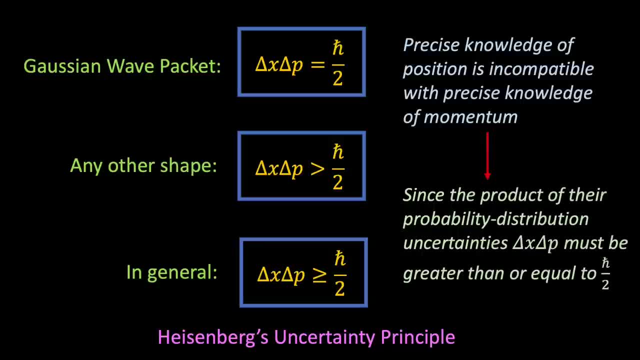 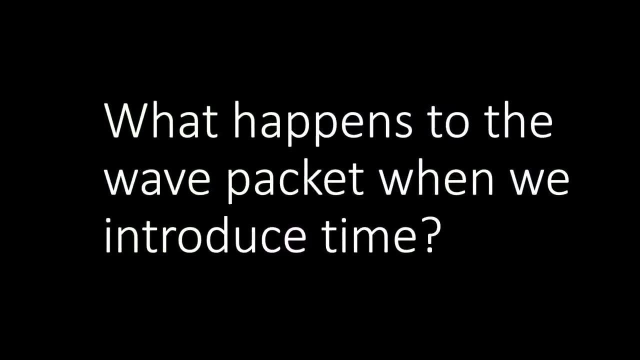 is incompatible with precise knowledge of momentum, since the product of their probability distribution uncertainties, delta x times delta p, must be greater than or equal to h bar over 2.. Now you might think that this would be a natural point to end the video, but we haven't actually. 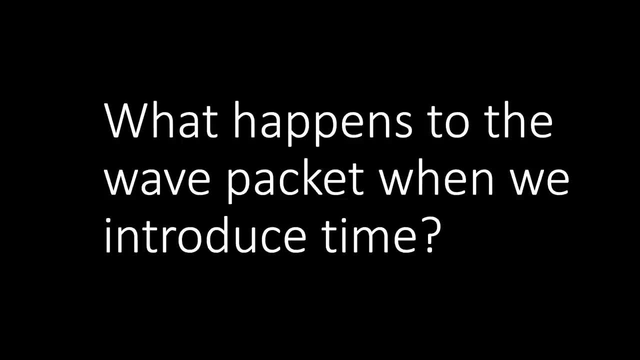 answered the question posed at the beginning, which was to find out how to describe the motion of a freely moving particle. So far, we've not included time in our analysis, And so, to end this video, I would like to briefly discuss what happens to our wave packet when we introduce the dimension of time. 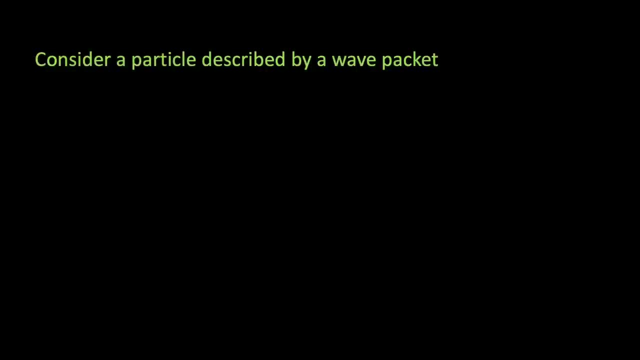 To begin with consider a particle moving in the positive x direction, which at time t equals zero, is described by a wave packet that has an initial uncertainty in position of delta x naught and an initial uncertainty in momentum of delta p. 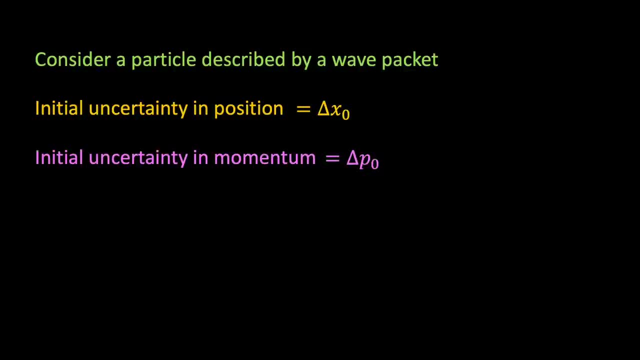 And we can relate this to the uncertainty in position using Heisenberg's uncertainty principle. Then the uncertainty in the particle's momentum leads to an uncertainty in the particle's velocity, given by delta. p naught over m, And if we sum in the expression for delta, 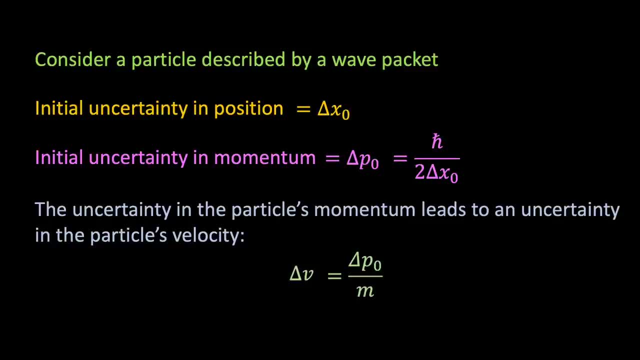 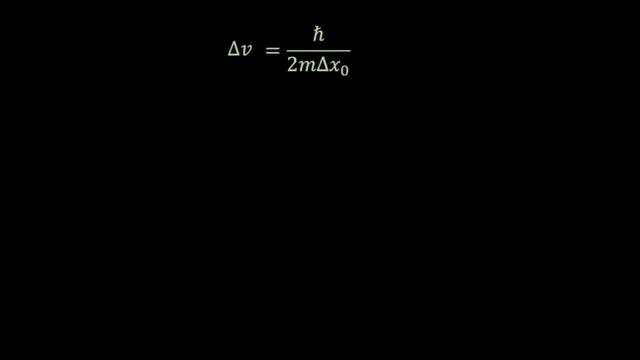 p naught that we just calculated. we find that the uncertainty in the particle velocity is given by h bar divided by 2m delta x naught. Now this uncertainty in the wave packet velocity means that different parts of the wave packet will move with different. 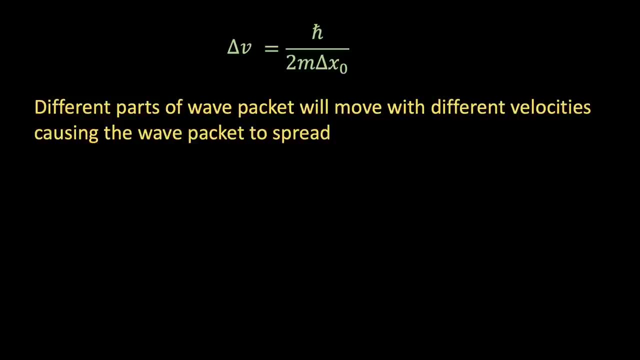 velocities causing the width of the wave packet to increase with time. After t seconds, we would expect the width of our wave packet, delta x of t, to be roughly equal to the uncertainty in the velocity multiplied by the time t, which gives a result of h bar. 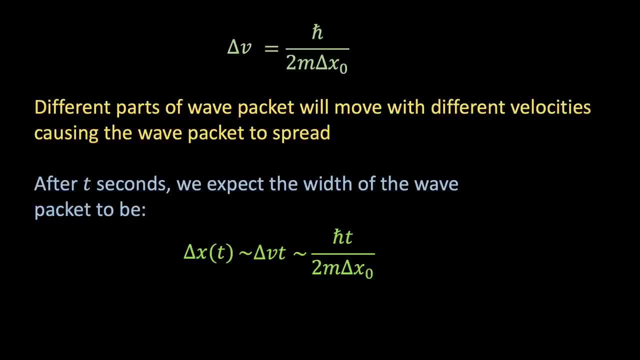 t divided by 2m, delta x- naught where, as you recall, delta x naught is the velocity of the wave packet and the velocity of the wave packet is the velocity of the wave packet. So delta x of t is the time t, which is the velocity of the wave packet when we multiply. 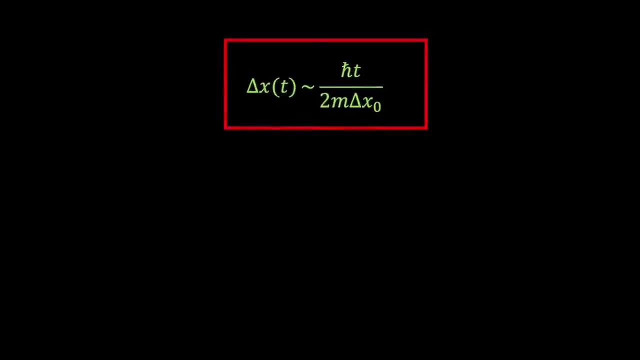 the initial width of the wave packet. This expression is showing us that as time increases, the width of our wave packet will also increase. And we also see that if we try to make the initial wave packet very small so that delta x naught approaches zero, then delta x of t 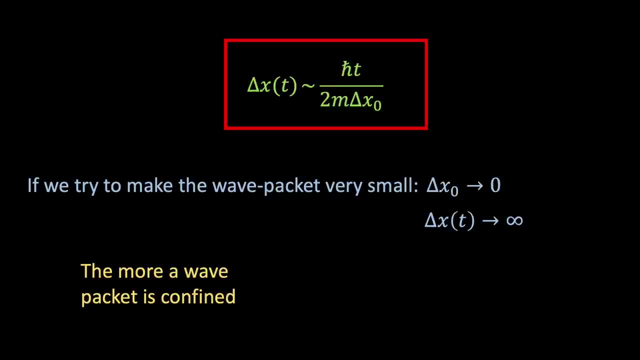 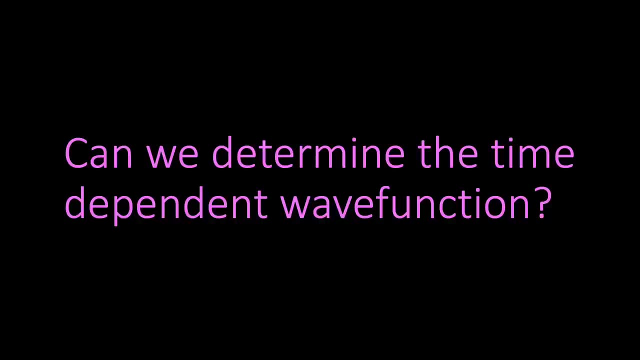 will approach infinity, and so we see that the more a wave packet is confined, the faster it will expand, And so our final task, before we end this video, is to ask the question: can we determine the time dependent wave function so that we can understand the evolution of our wave packet as time progresses? 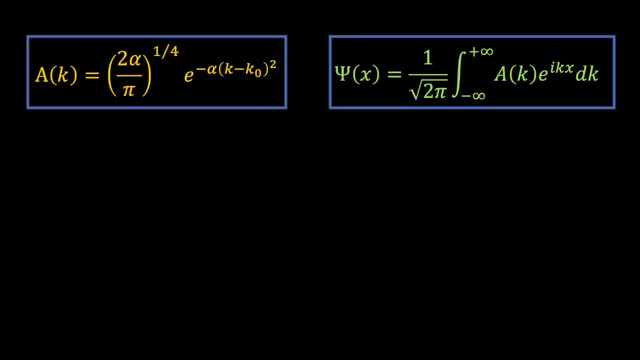 To begin with recall our earlier analysis where we were able to calculate the time independent wave packet wave function. psi of x by substituting in the Gaussian amplitude function and then solving the problem. Now we can introduce time dependence by simply multiplying our time. independent wave function. 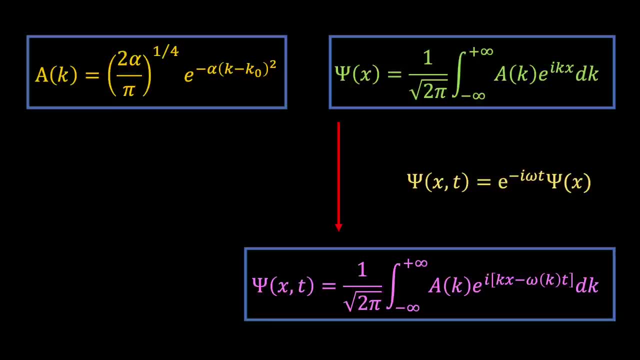 by the factor e to the minus i omega t, in which case we find the following expression for psi of x t, We see that the e to the i kx term has become an e to the i kx minus omega t term and we have written omega brackets k to highlight the fact that omega is a function. 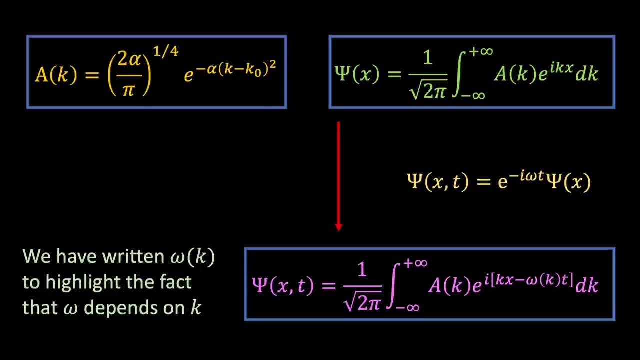 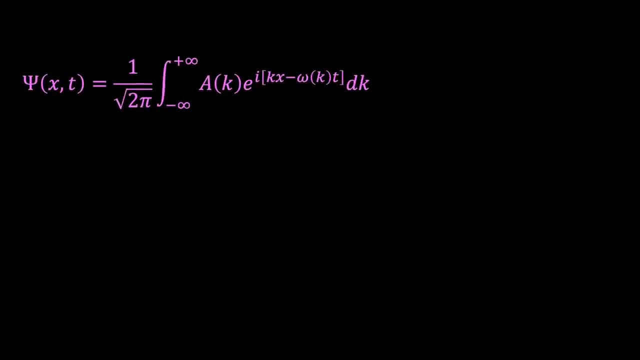 of k For our free particle. this simply means that the energy depends on the momentum. Next, if we sub in our Gaussian amplitude function a of k, we find the following green expression: Now, if you recall from our earlier analysis the trick to solving this integral: 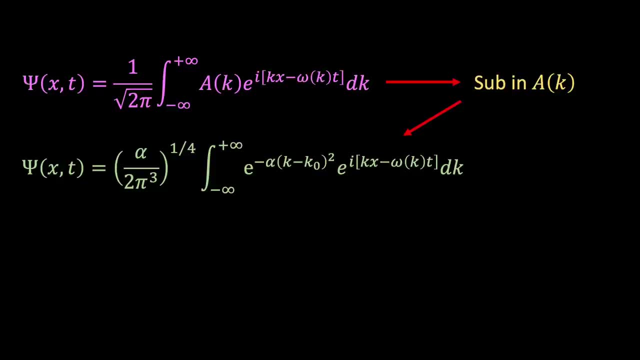 was to simplify the integrand by changing variables to k. prime equals k minus k- naught. However, we now have an e to the minus i omega t. Now we can simply multiply the integral by changing variables to k: prime equals k minus k- naught. However, we now have an e to the minus i omega t and we have written the following: 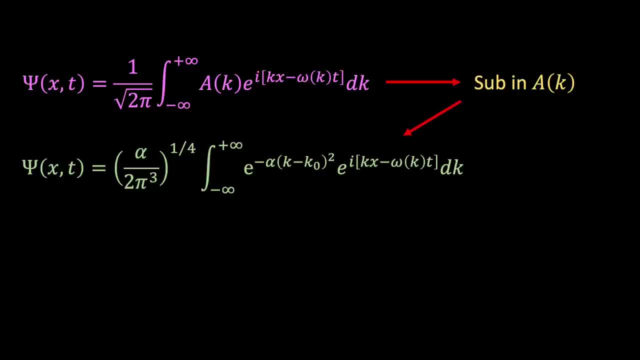 e to the minus i, omega t, term appearing in our integral, which we didn't have before. So what do we do? Well, the solution is to perform a Taylor series expansion of omega of k around the centre of the wave packet k naught in k space. In other words, we are 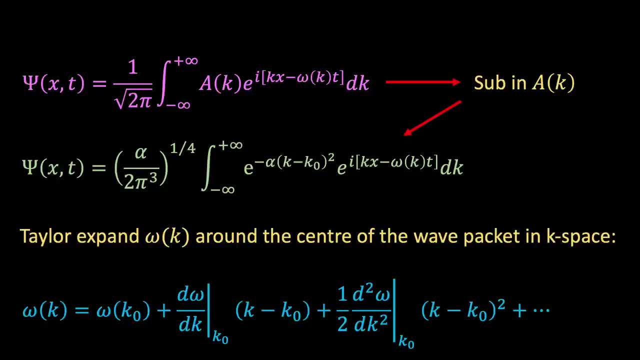 going to write. omega of k equals omega of k naught plus d. omega by d k evaluated at k naught times k minus k naught plus half times the second order derivative of omega with respect to k evaluated at k naught times k minus k naught, squared plus higher order. 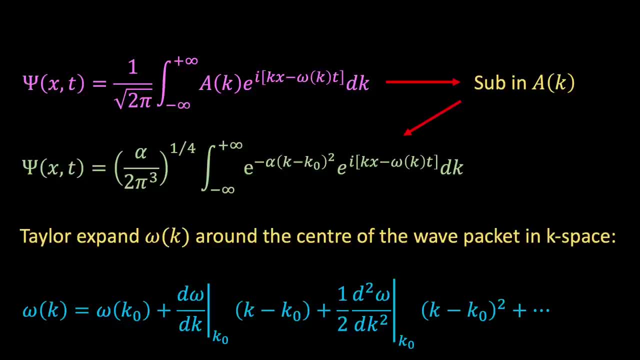 terms. Now, the reason for doing this is it allows us to express omega of k as a series of terms, each of which involves a factor of k minus k. naught, We will ignore the higher order terms at this stage, as their contribution will be negligible for the calculation that. 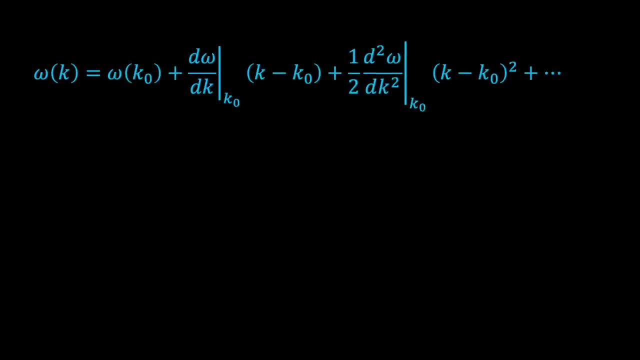 follows. Now we can neaten this up a little bit by noticing that the integral of omega of k equals omega of k minus k naught plus half times the second order derivative of omega with respect to k, evaluated at k naught times k minus k naught, squared plus higher. 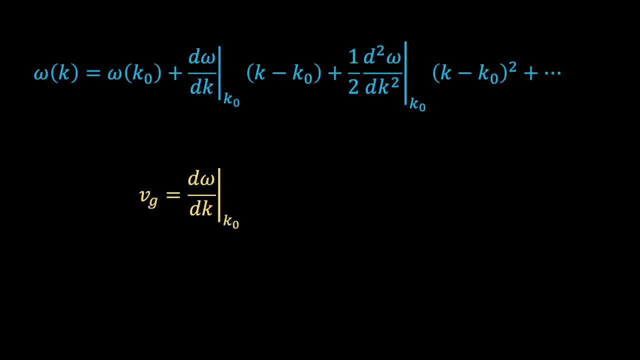 than the second order derivative of omega with respect to k is simply the group velocity of our wave packet, which we encountered earlier. And to streamline our notation further, we will also define beta as being equal to half times the second order derivative of omega with respect to k, and omega naught as being equal to omega of k naught. This then allows: 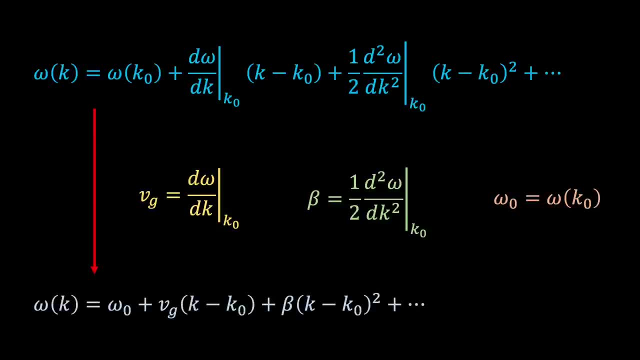 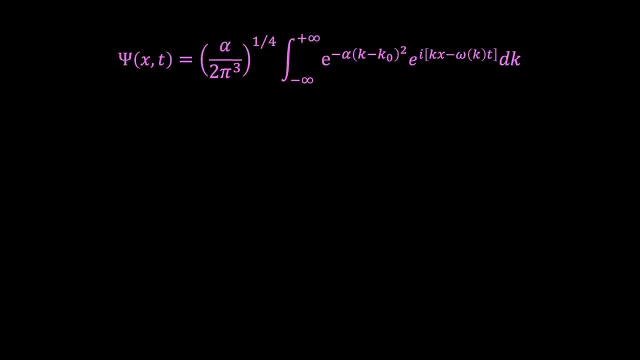 us to write the omega k expansion in the following form: If we then sub this expansion back into our wave function expression, we find the following yellow equation: And if we then make the substitution k prime equals k minus k naught, we can rewrite the wave function in the following: 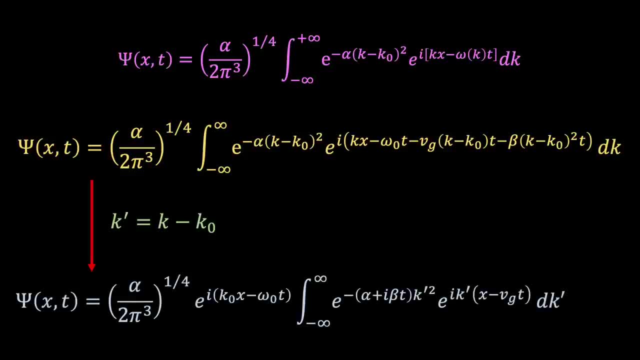 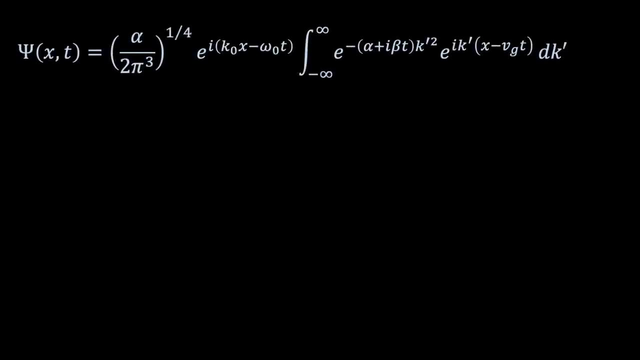 form where we have pulled out a factor of e to the i, k naught x minus omega naught t in front of the integral. Next, if we compare this rather horrendous expression with the time independent expression for psi of x we encountered earlier, which 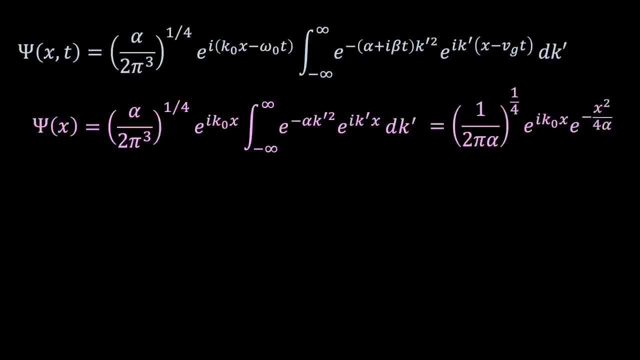 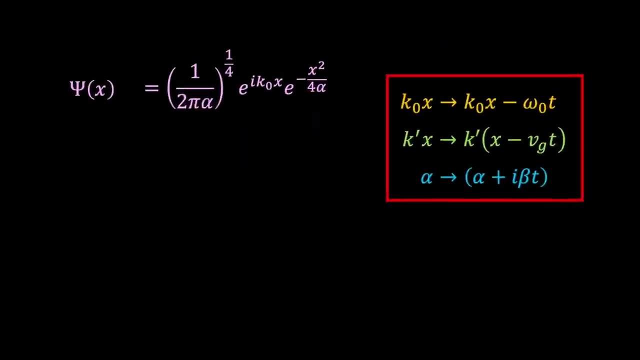 if you recall, had the following Gaussian solution. then we see that our time dependent wave function psi of x- t has exactly the same form as the time independent wave function psi of x, provided we make the following substitutions: And so, rather than having to go through the pain of solving our horrific time dependent, 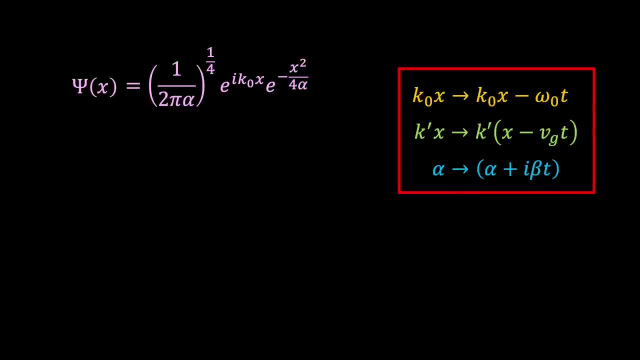 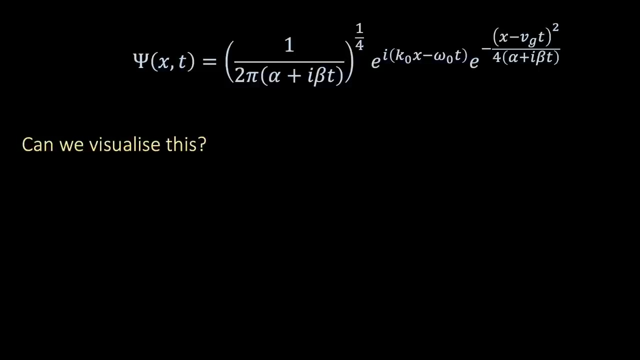 integral. we can simply write down the answer by taking the time independent solution and then making the substitutions contained within the red box. If we do this, we find the following beautiful expression for our time: dependent wave packet, wave function. So what is this wave function telling us and can we visualise it? Well, let's begin by plotting. 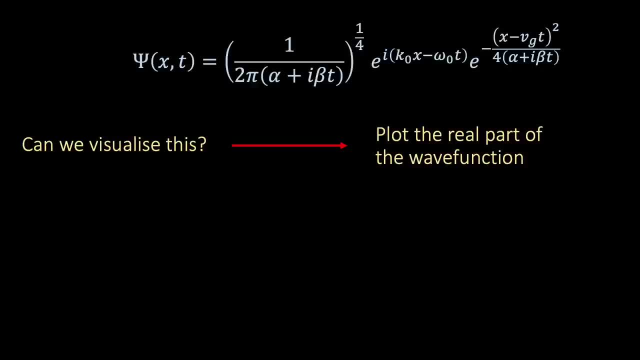 the real part of this wave function and observe how it evolves with time. If we do that, we see that the wave packet spreads and widens as the wave packet expands and widens as the wave packet moves through space. So does this mean that the particle itself is in some 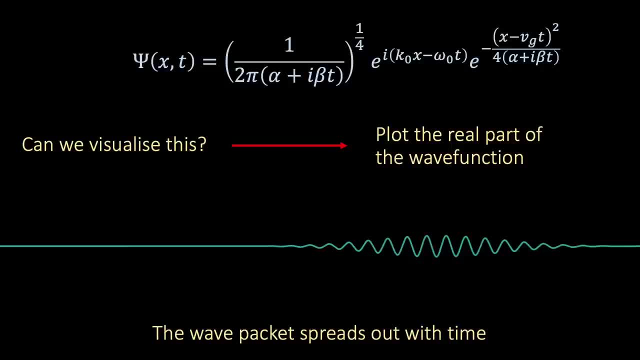 sense spreading out? Well, the answer is no. If you recall, the wave function provides information about the probability of finding the particle at a particular location in space. To be more precise, it's the modulus squared of the wave function that tells us the probability. 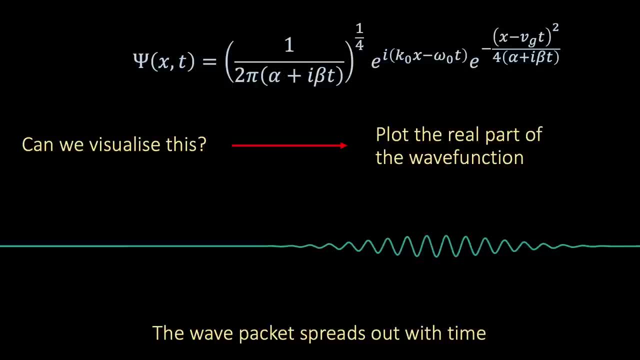 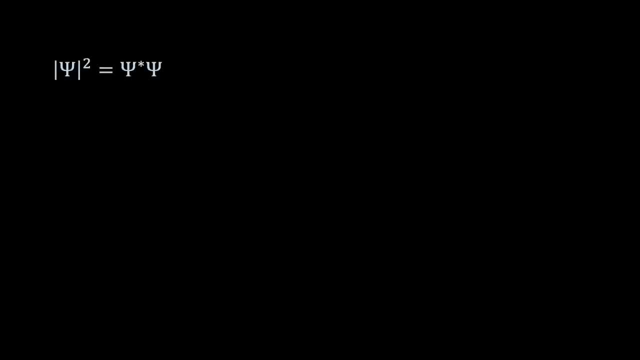 density. and so let's quickly calculate this and see what we get. Recall that the probability density is given by the modulus squared of the wave function. and if we calculate this for our time dependent wave function, we find the following expression: And if we plot this: 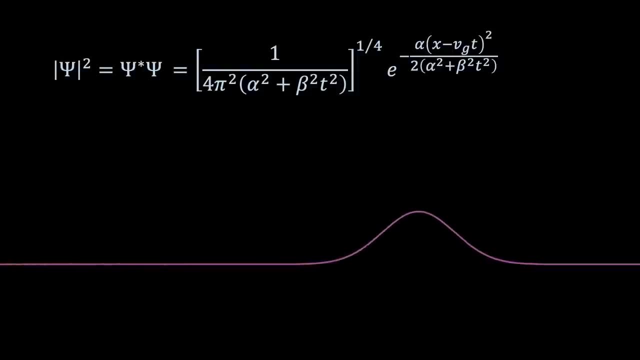 we see that the width of our probability distribution increases with time, meaning that the uncertainty in the particle's location also increases with time, which is precisely what we argued earlier. And so there you have it. If you've managed to follow up to this point, then when? 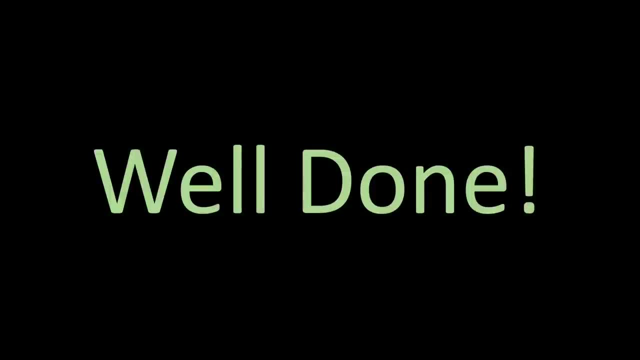 do you think you're going to be able to solve this problem? Let me know in the comments. Well done, I hope that you now have a slightly better understanding of how a freely moving particle is described within the framework of quantum mechanics And, furthermore, I hope. 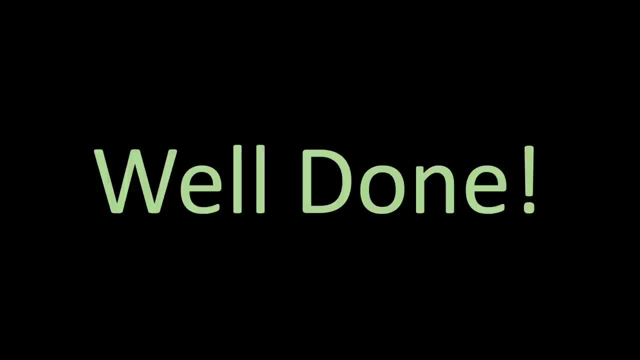 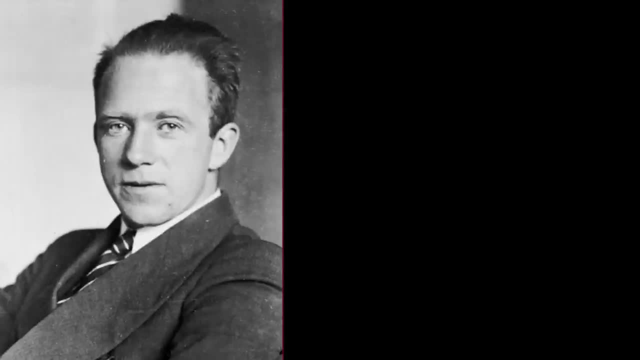 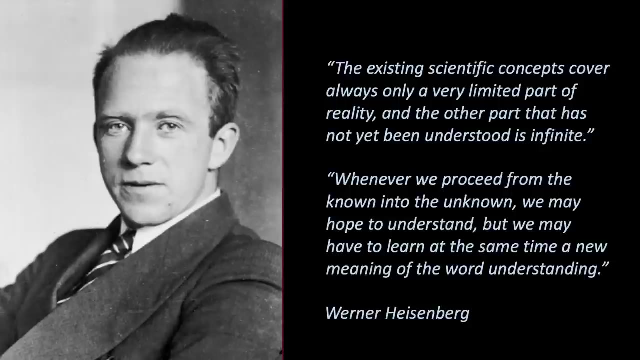 that you see the deep link between our probabilistic wave packet description of a particle and Heisenberg's uncertainty principle. I think it only appropriate that we end with the words of Werner Heisenberg, who said: the existing scientific concepts cover always only a very limited part of reality. 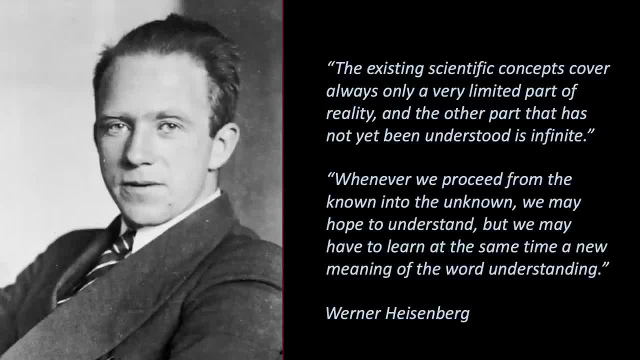 and the other part that has not yet been understood is infinite. Whenever we proceed from the known into the unknown, we may hope to understand, but we may have to learn at the same time a new meaning of the word understanding. I hope you've enjoyed this video and I'll see. you next time.